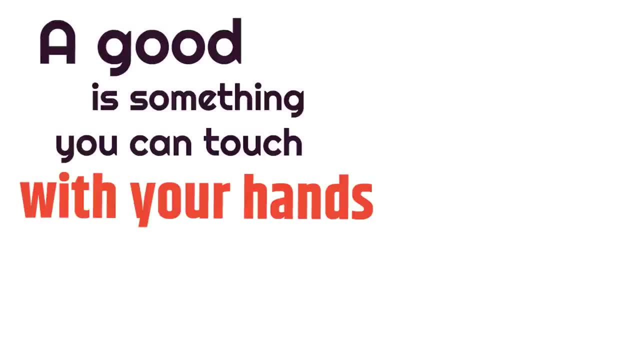 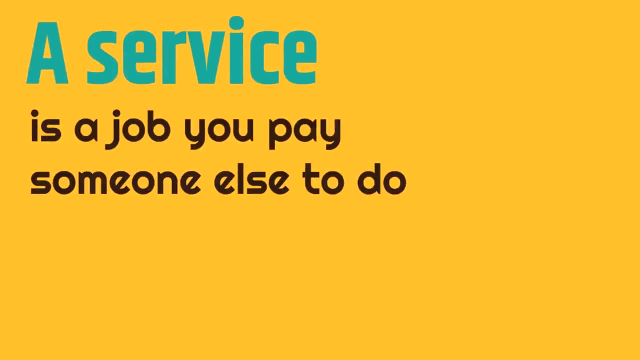 A good is something you can touch with your hands, like a skateboard. A skateboard is a good. It's something you can buy and you can touch with your hands. Now, a service is a job you pay someone else to do. A great example of that is painting a house. 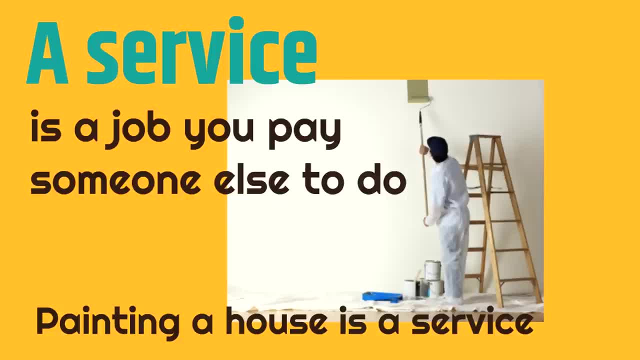 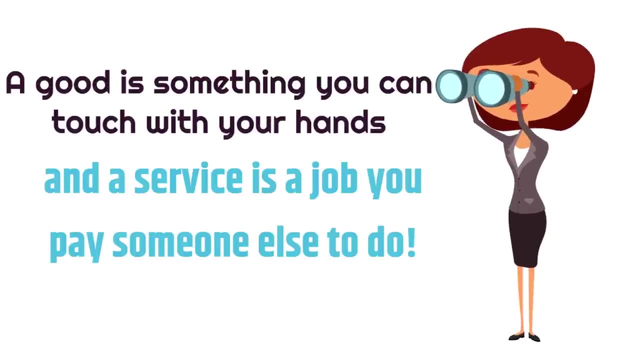 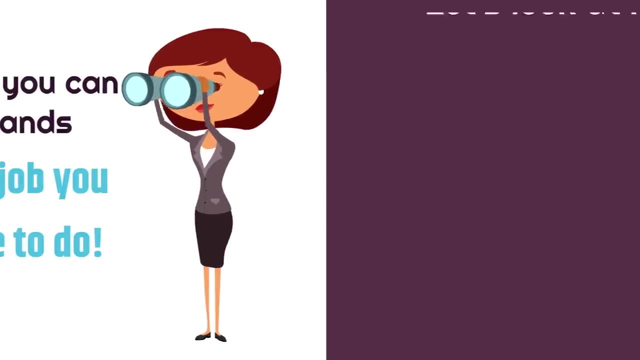 Painting a house is a service. It's a job you pay someone else to do. So a good is something you can touch with your hands, and a service is a job you pay someone else to do. Let's look at some more examples. 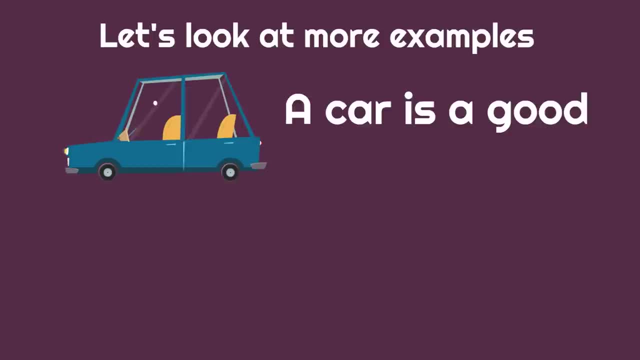 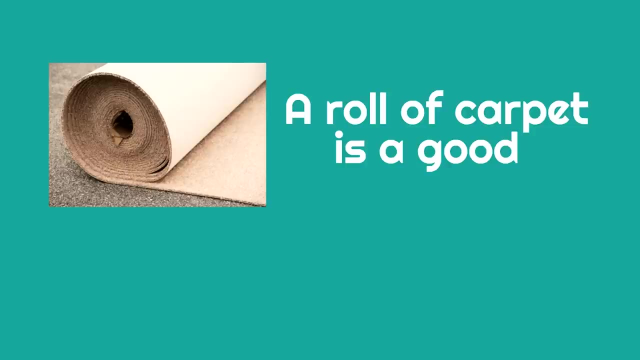 A car is a good. It's something you can touch. A car wash is a service. It's something you pay someone else to do. If you were to buy a roll of cardboard with a name tag, roll of carpet, that is a good. it's something you can touch, but laying 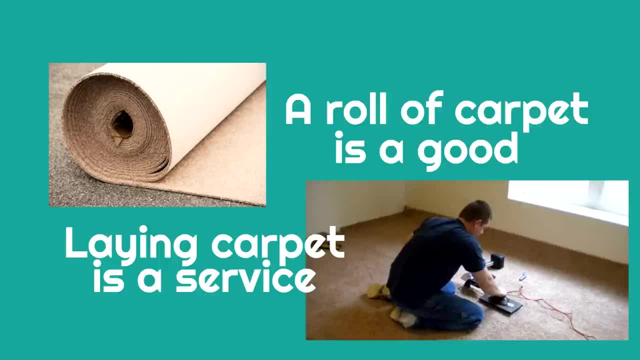 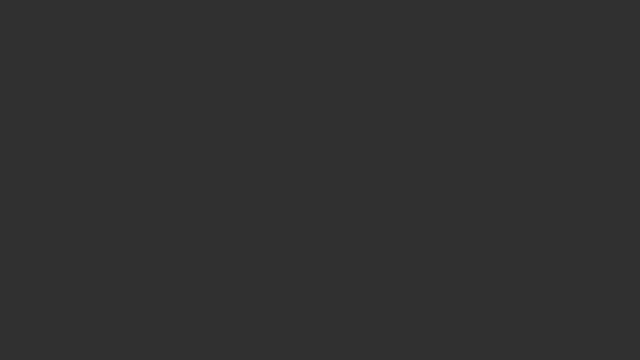 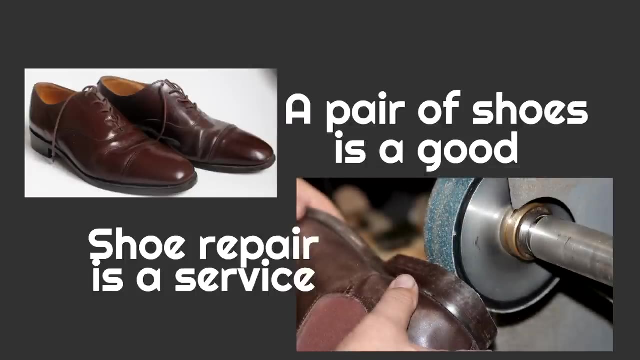 carpet is a service. when it gets installed, that is a service. last example: a pair of shoes is a good. if you bought shoes, that's a good, that's something you can touch. but if your shoes break, the shoe repair is a service, it's a job that. 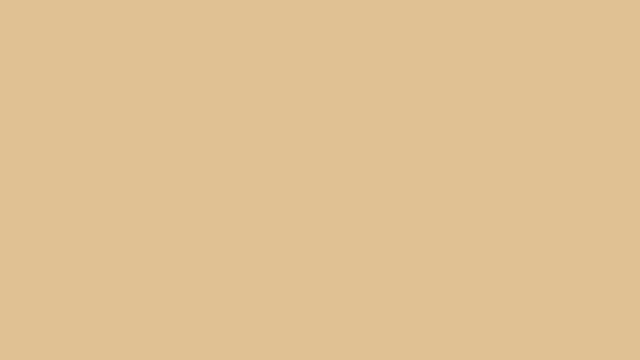 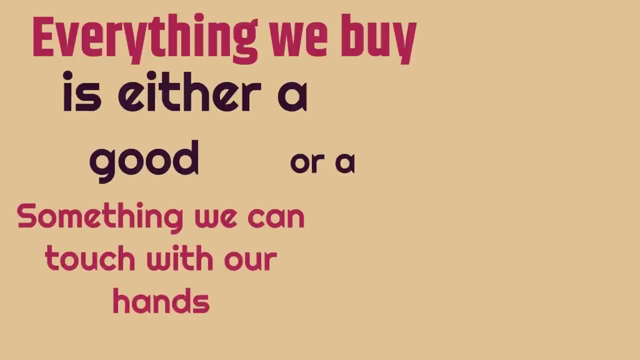 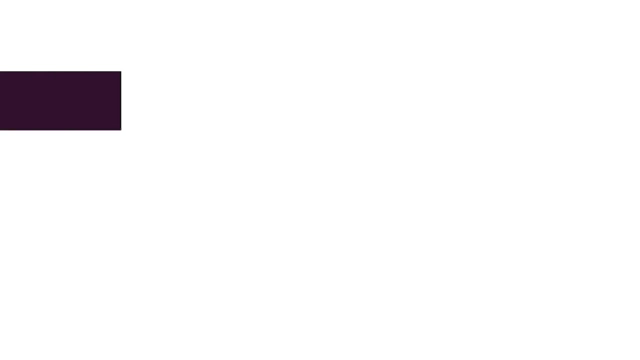 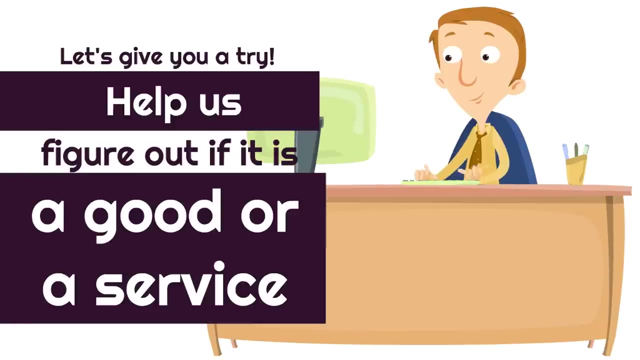 you pay someone else to do. everything we buy is either a good, something we can touch with our hands, or a service, a job we pay someone else to do. so let's give you a try. help us figure out if it is a good or a service. we're gonna do a. 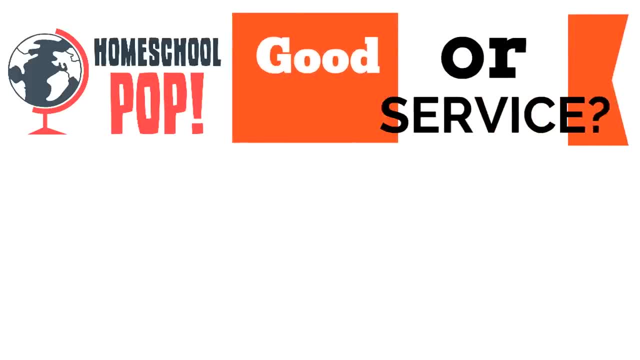 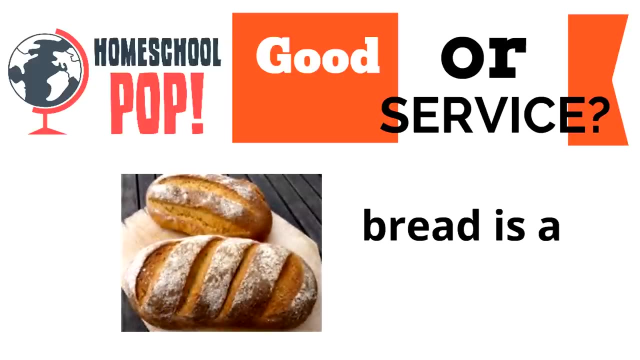 little game that we call homeschool pop good or service. we're gonna show you a picture and you're gonna tell us whether you think it's a good or a service. here's our first one: bread. bread is a. is it a good or a service? yeah, bread is a good. 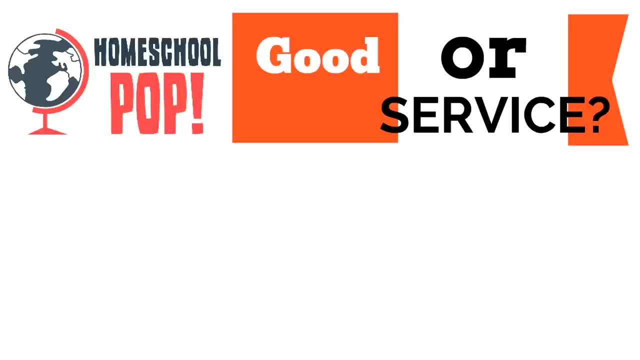 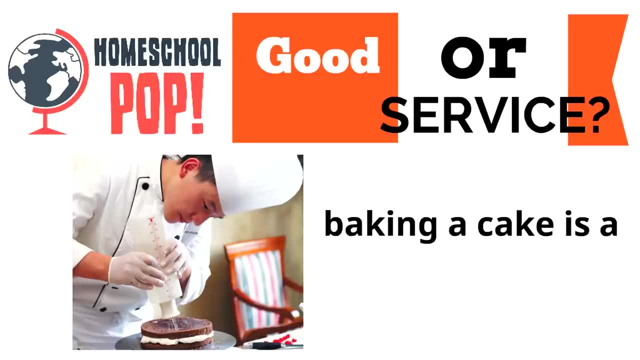 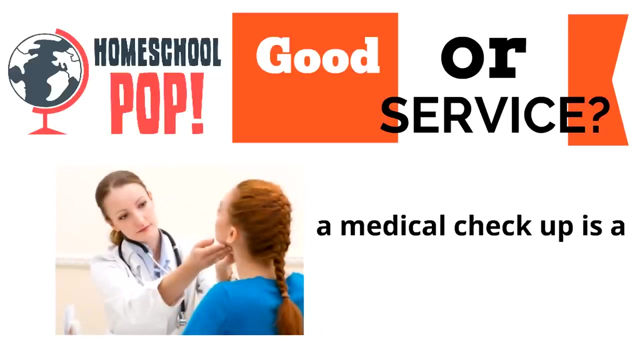 something you can touch. try this one: baking a cake. baking a cake is a. you know which one? it's a service. it's a job you pay someone else to do. what about this one? a medical checkup. a medical checkup is a. is it a good or service? yeah, it's a service. it's. 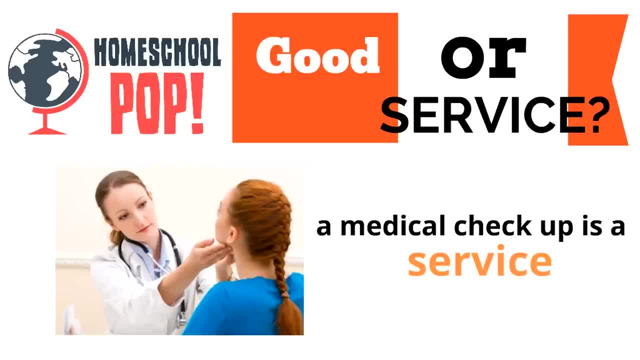 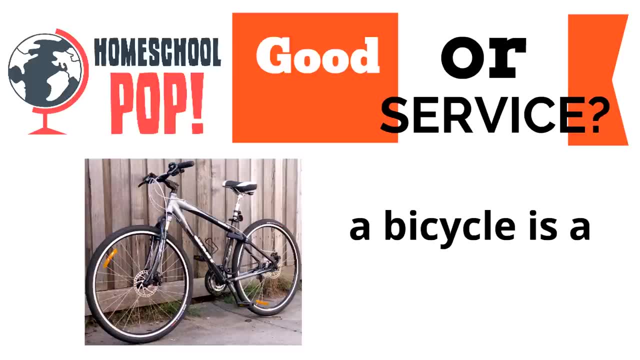 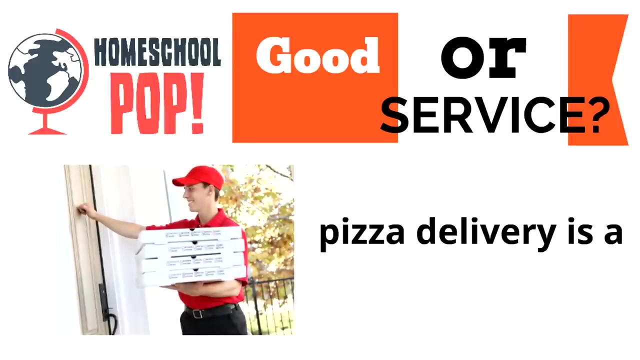 a job you pay someone else to do. what about this one? a bicycle. a bicycle is a a. yeah, it's a good. it's something that you buy, that you can actually touch. good job, we all like this one. pizza delivery is a. do you know which one it is, a good or a service? 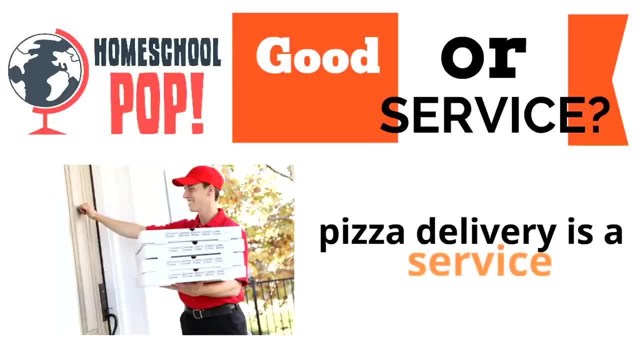 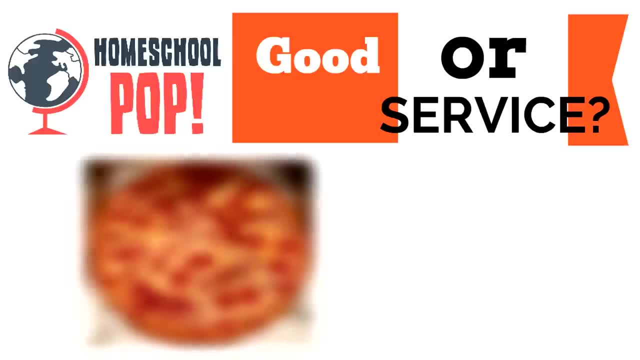 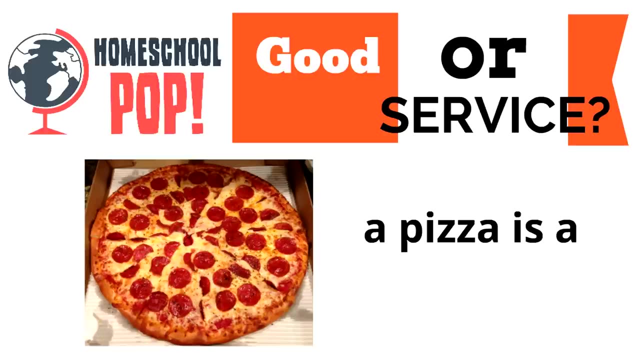 good or a service. It's a service. It's a job you pay someone else to do. Here's our last one. A pizza is a. We had to do this after the pizza delivery. What is a pizza? A pizza is a good. It's something that you buy, that you can actually touch. 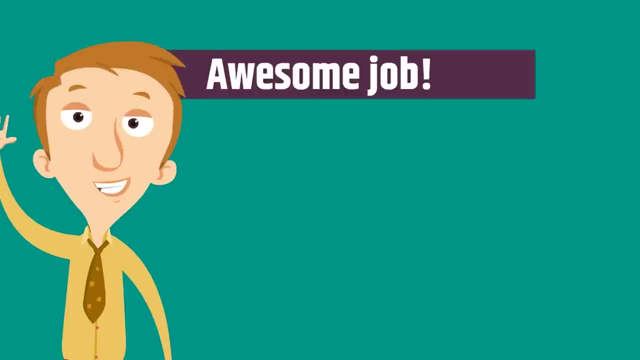 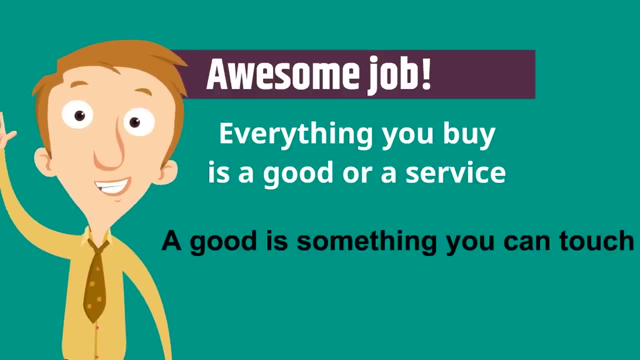 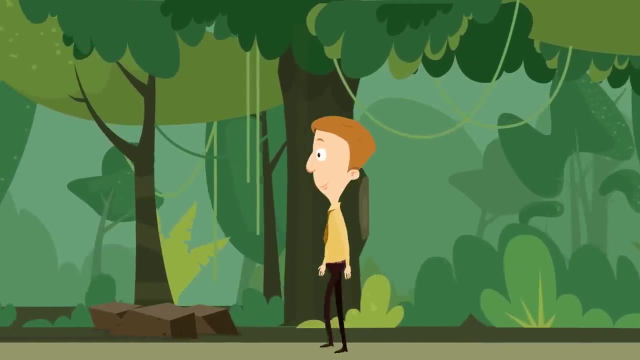 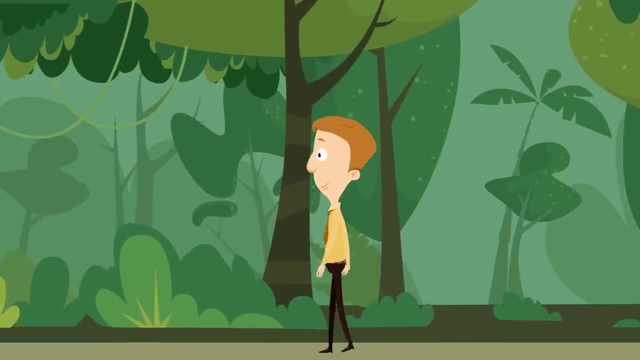 Awesome job. Thanks for playing. Everything you buy is a good or a service. A good is something you can touch. A service is a job you pay someone else to do. Well, that wraps it up. Next time you buy something, you can ask yourself: am I buying a good or a service, And you'll know the right. 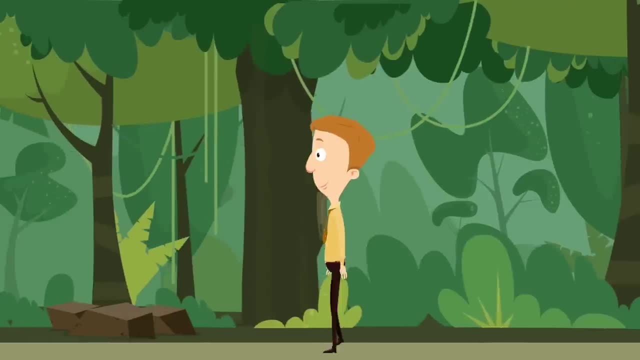 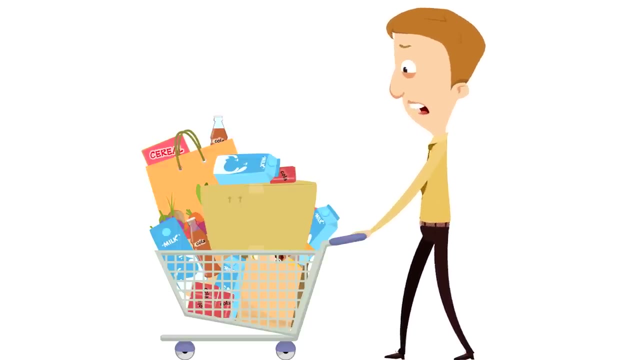 answer because you watched this whole video. Oh, this is such a heavy cart. Oh my goodness, It's hard work. You know, a lot of times, learning can be hard work too, but we hope that these videos are really helpful and make learning fun. 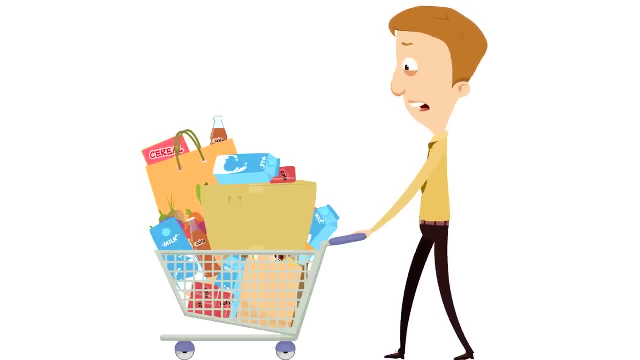 so that learning isn't hard like pushing this cart. Oh my goodness. All right, What's the next thing we should learn about? Let's learn about the purpose: The purpose of government. Governments are formed to keep people safe and to help people work. 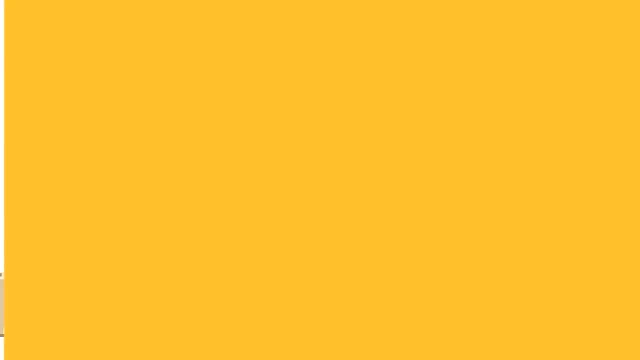 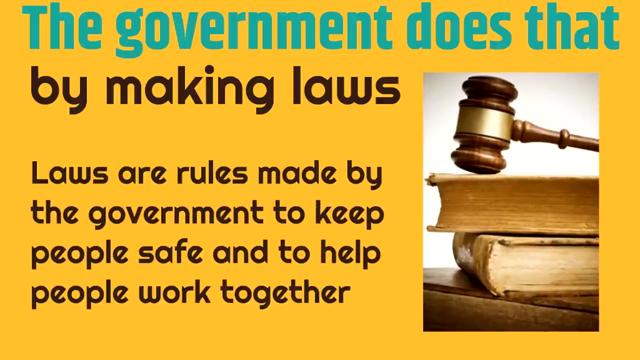 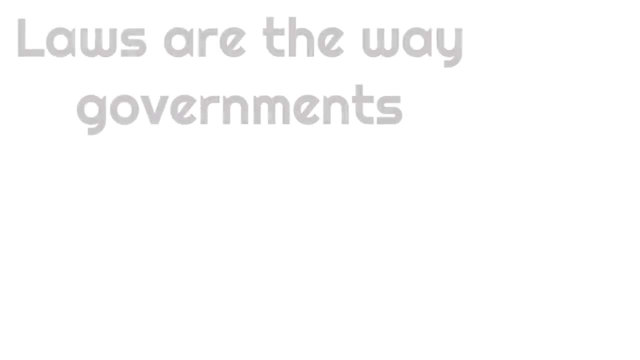 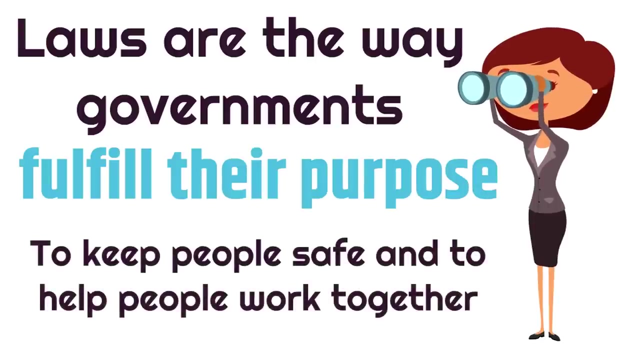 together. The government does that by making laws. Laws are rules made by the government to keep people safe and to help people work together. You see, laws are the way governments work And they fulfill their purpose: to keep people safe and to help people work together. Some laws you might. 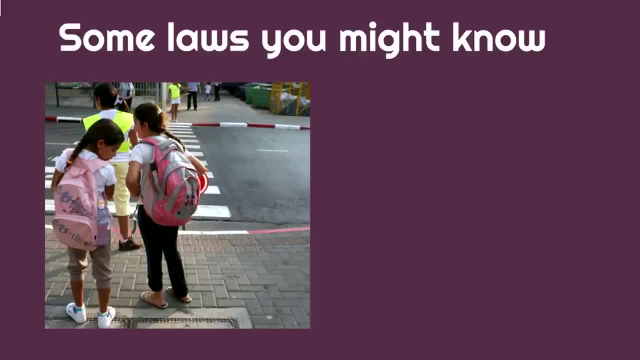 know What about this one? You must not cross the road when the light is red. This is an important law because it keeps people safe, And that's one of the main purposes of government is to keep people safe. if you cross the road when the light is red, you can get hurt, so they set up a 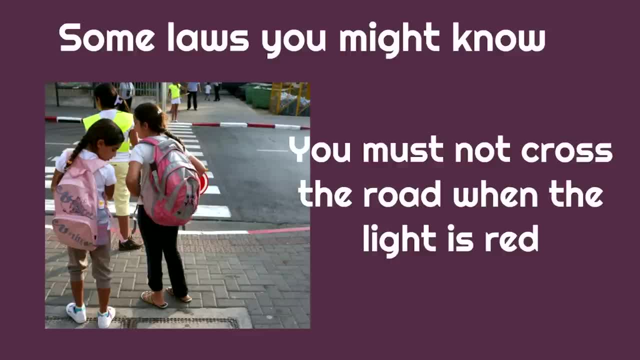 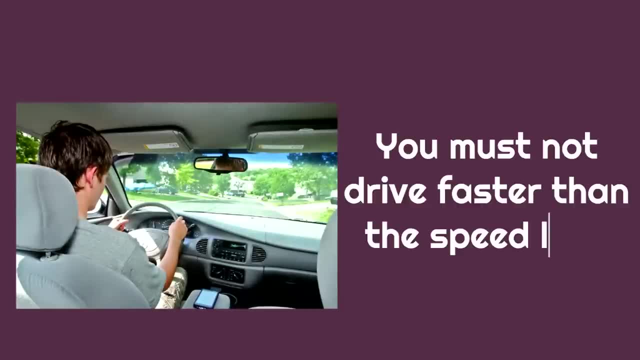 law: you must not cross the road when the light is red. what about this law? you must not drive faster than the speed limit. this is a law the government set up because it wanted to help keep people safe and help people work together. when you drive faster than the speed limit, you can hurt. 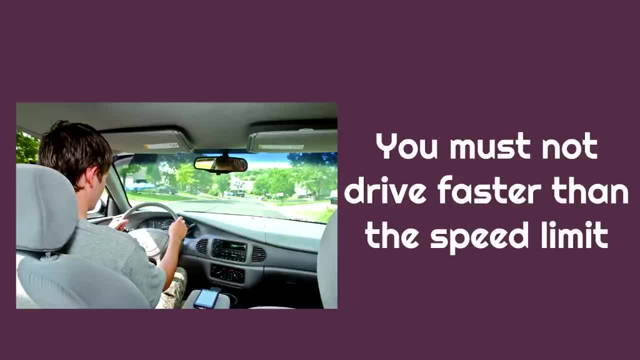 yourself and you can hurt other people. it's not safe now. it also doesn't help people work together, because when you're on the road with other drivers, you're working together to get to where you need to go and you need everyone to follow the laws. you must not drive faster than the speed limit is a law. 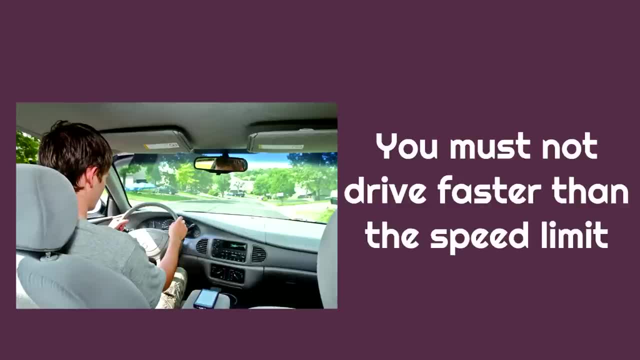 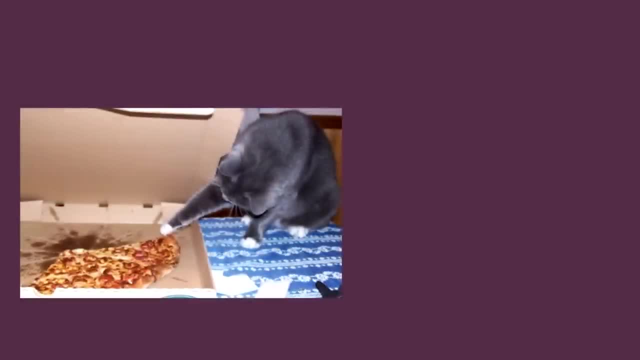 because it keeps people safe and it helps people work together. here's one I'm sure that you've heard of the speed limit. it's a law that allows people to drive faster than the speed limit and it's a law that you know you must not steal. 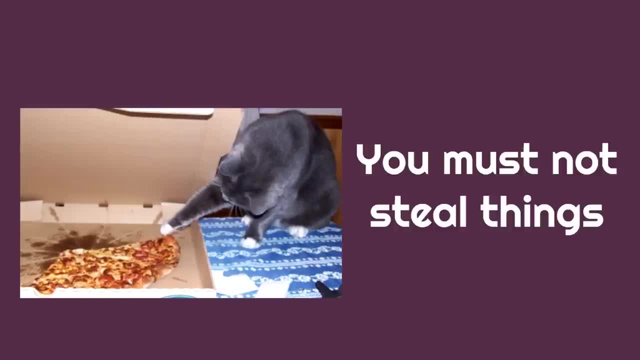 things. this is a law that's very important because it keeps people's possessions safe and it helps people work together. you can't work together and help other people if you're taking things that belong to them. that is why the government has a very important law: that you must not steal things when you. 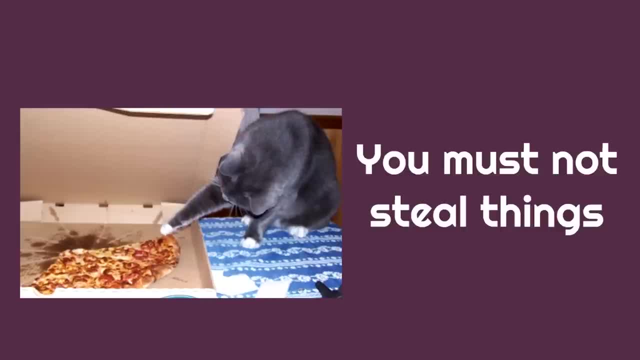 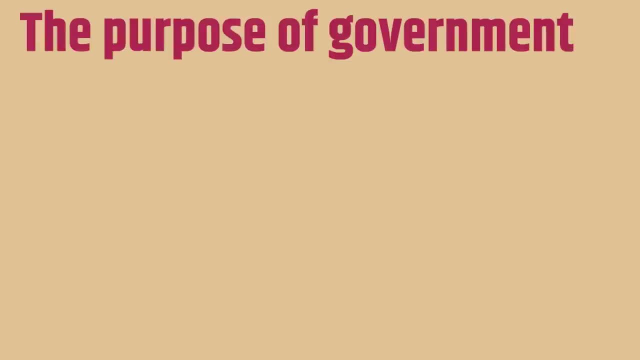 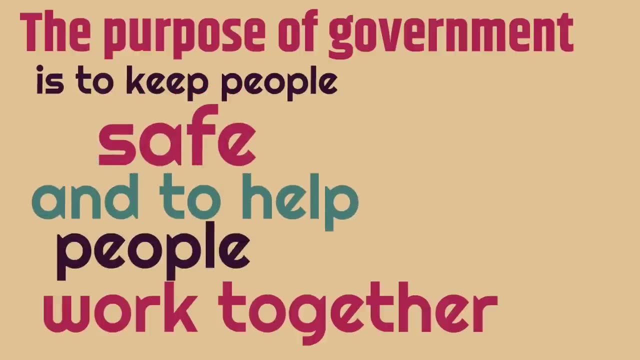 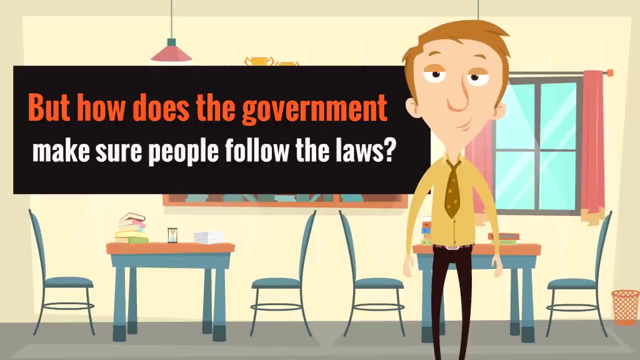 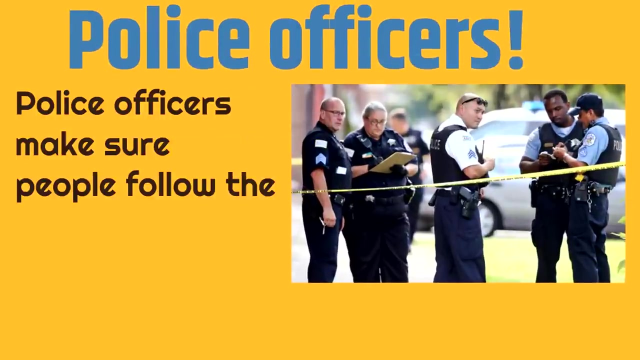 steal things. it hurts other people, it doesn't keep people safe and it doesn't keep people work together. the purpose of government is to keep people safe and to help people work together, but how does the government make sure people follow the laws? police officers, police officers- make sure people follow the laws. 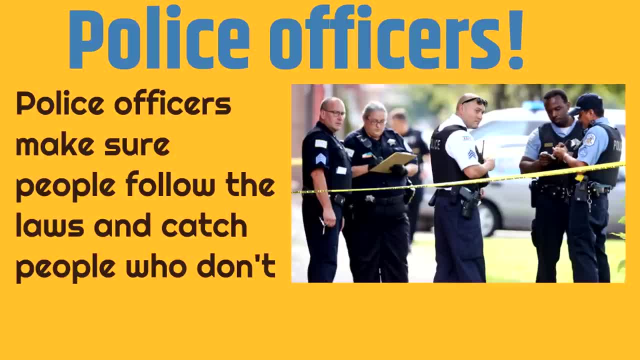 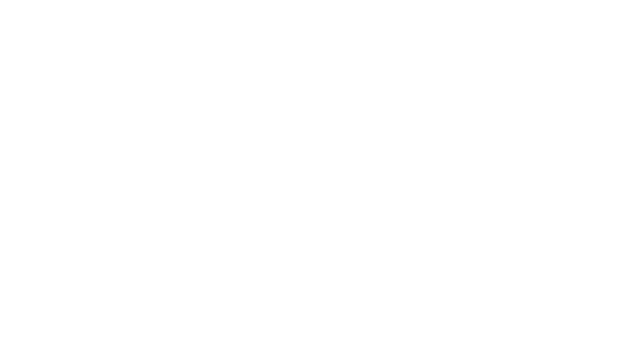 and catch people on the road with the speed limit. it can cause a lot of injuries in the future. catch people who don't. They also keep our communities safe and help people who are in trouble. Then, after they've been caught by the police, the court system. 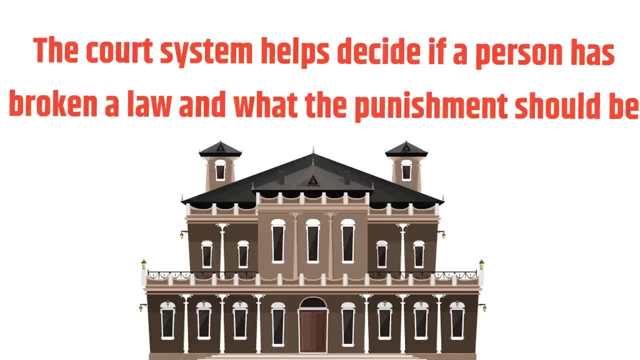 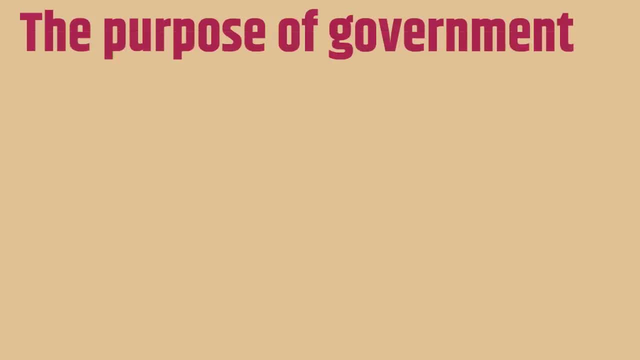 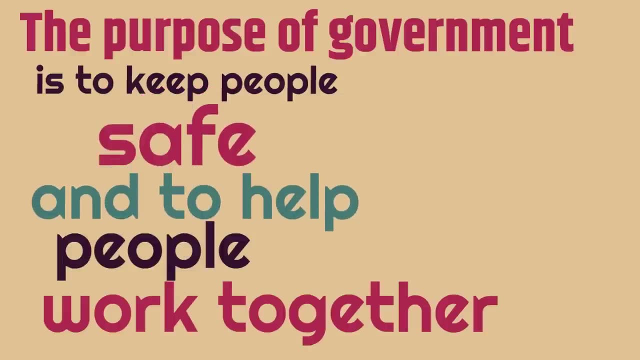 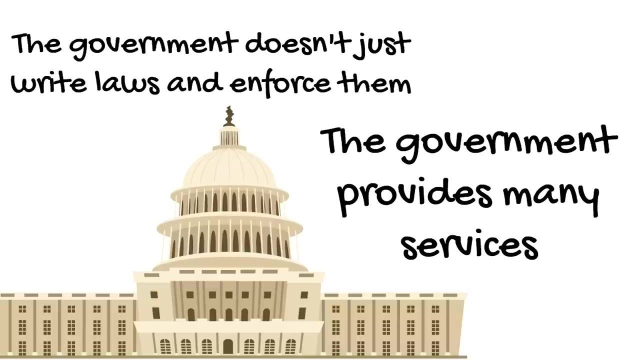 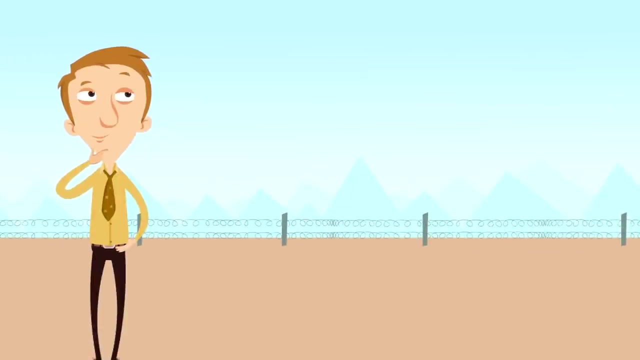 helps decide if a person has broken a law and what the punishment should be. The purpose of government is to keep people safe and to help people work together. The government doesn't just write laws and enforce them. The government also provides many services- Services like fire departments. That's something the government runs because it 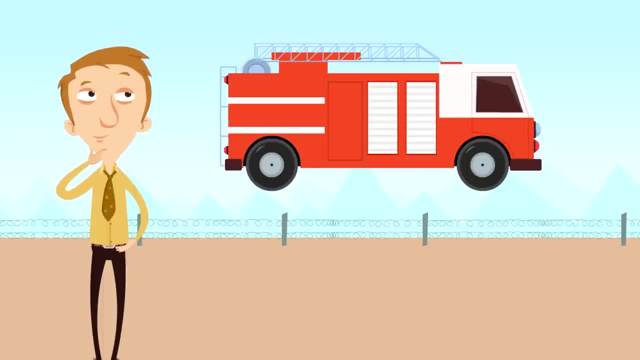 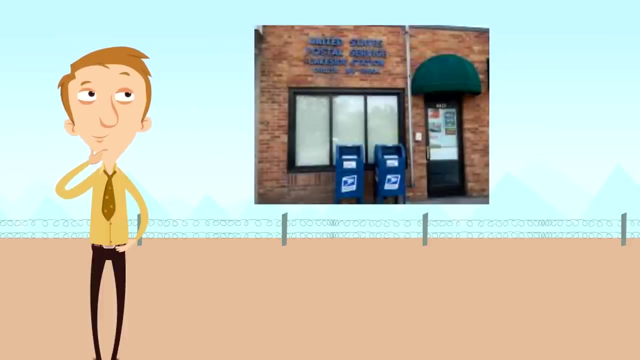 helps keep people safe. It's part of the purpose of the government to keep people safe and that's why they provide the service of fire departments. The government also provides the Postal Service. The Postal Service is the way that we send letters and packages and all kinds of fun things. 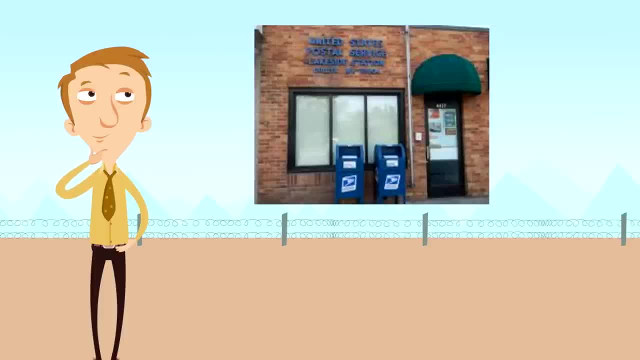 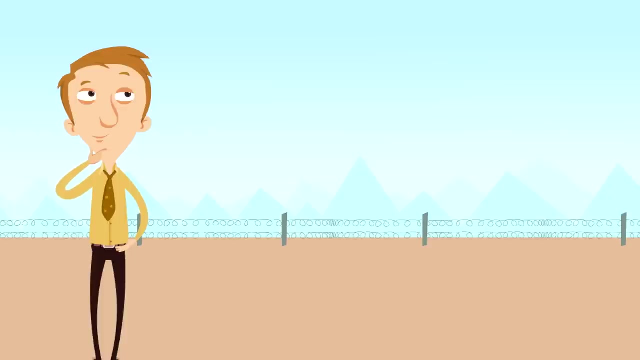 and helps us work together. That's part of the purpose of government is to help us work together, and the Postal Service helps us do that. That's why the government provides that service. The government also provides the services of libraries. Libraries are very, very important. The government runs. 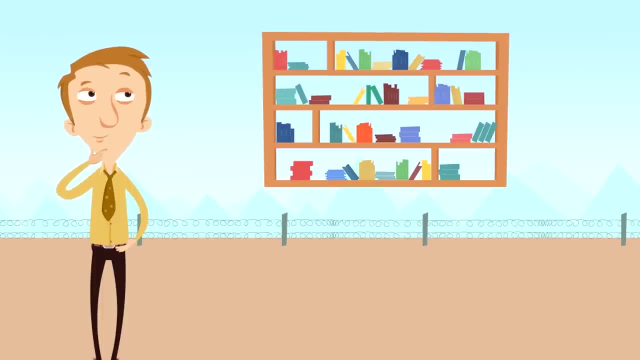 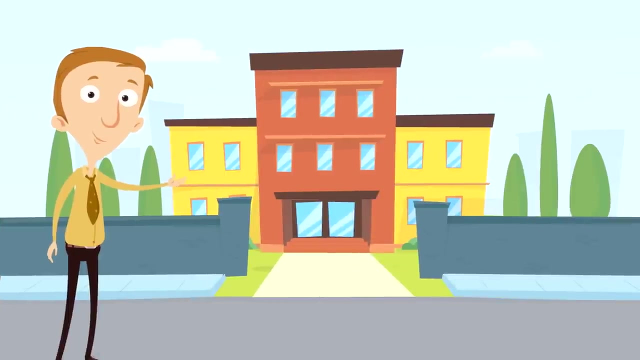 those, because libraries teach us and we get knowledge and with that knowledge it helps us work together. That's why the government provides libraries. The government also provides public schools. This is very, very important because everyone has the right to learn, and when we learn and when we get. 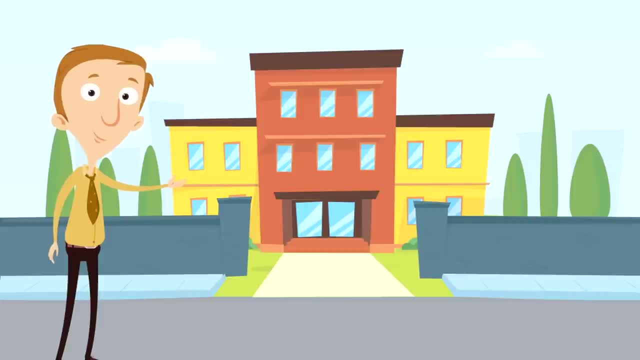 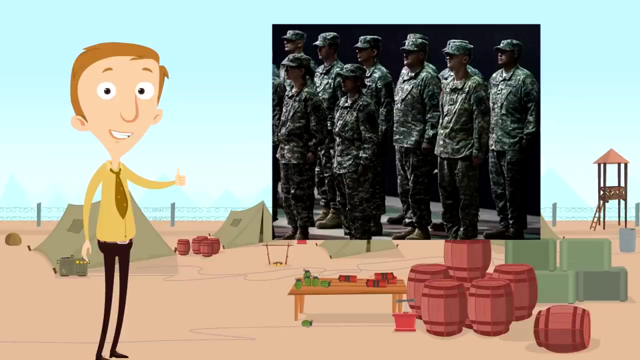 an education, we are able to work together better, which is why the government provides schools. The government also provides the services of the military, who protect us here and overseas, and it's very important for us to be safe. The government has to keep us safe, and the 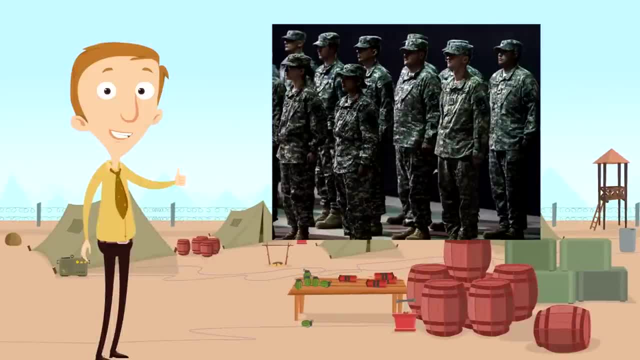 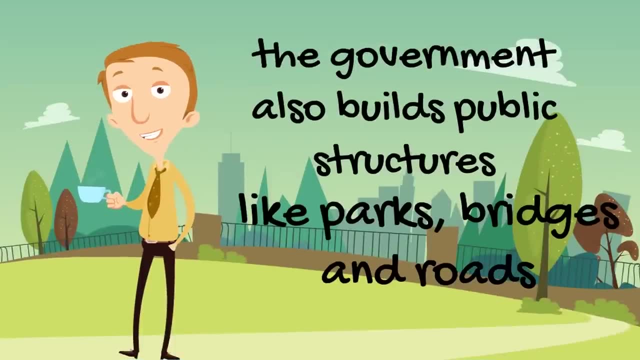 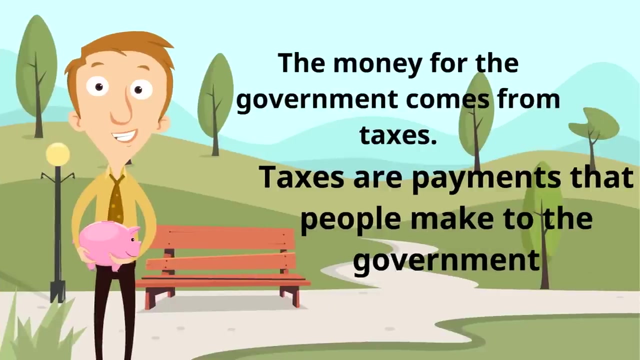 government does that through the service of brave men and women who serve in the military. The government also- Onu too- built public structures like parks and bridges and roads. This is very important because it alternately helps us to work onlight. So how do we pay for all this? 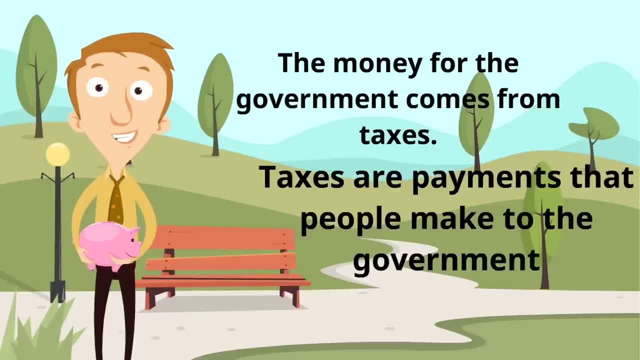 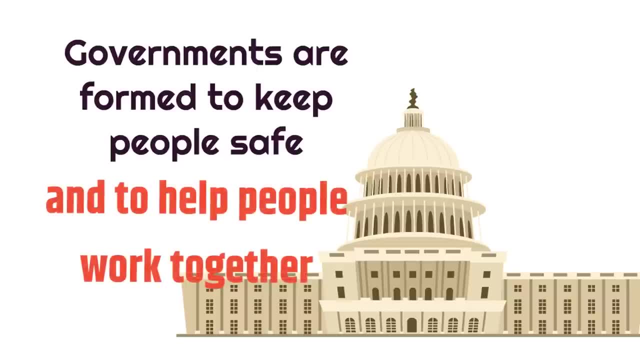 Well, the money for the government must come from taxes. Taxes are payments that people make to the government. Government can only do that through tax. You pay, Wouldn't you like to? Governments are formed to keep people safe and to help people work together. 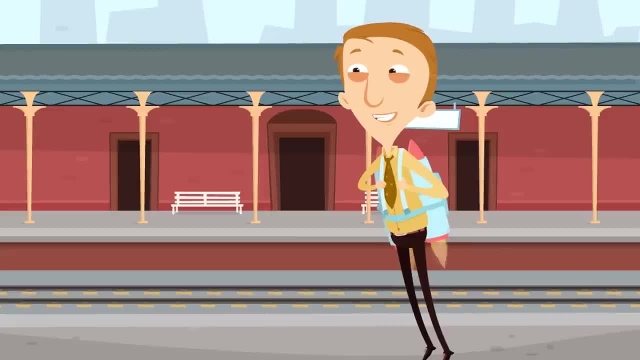 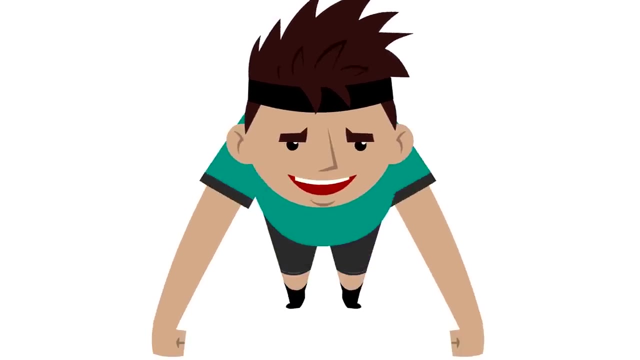 Well, that just about does it. If somebody ever asks you what does the government do and why is it there, You'll know what to tell them because you watched this video. How cool is that? You have been doing a great job, just like Mike who's doing these push-ups. 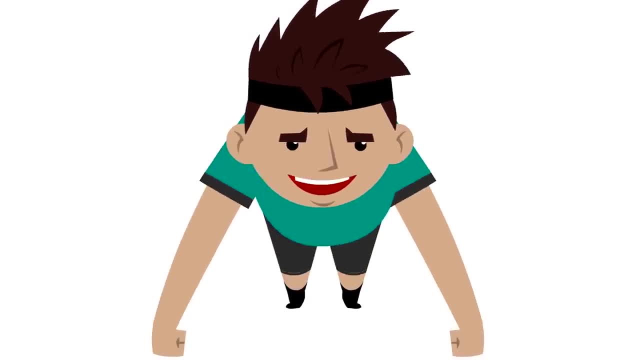 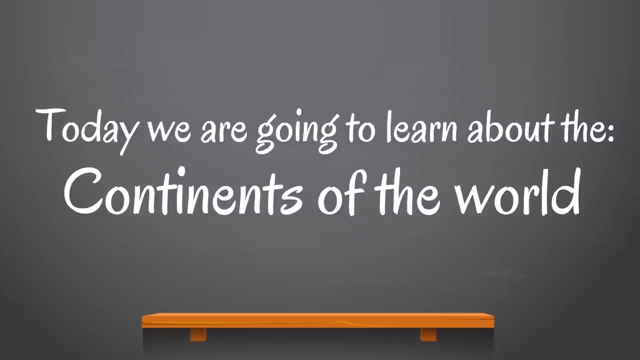 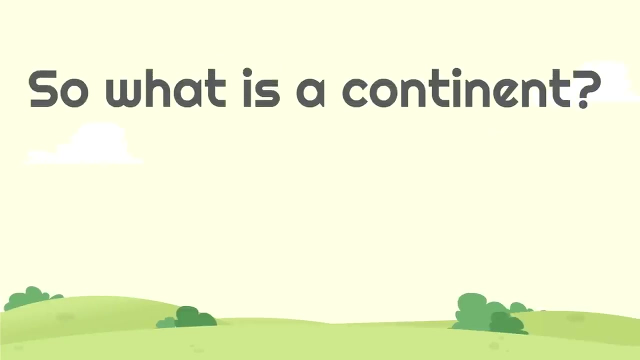 You know, he knows it's important to stay fit and exercise and to stay healthy, And you're like exercising your mind right now, which is super cool, And next we are going to learn about the continents of the world. So what is a continent? A continent is a large mass of land. 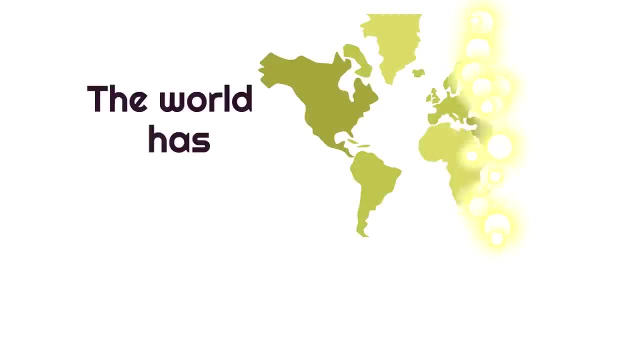 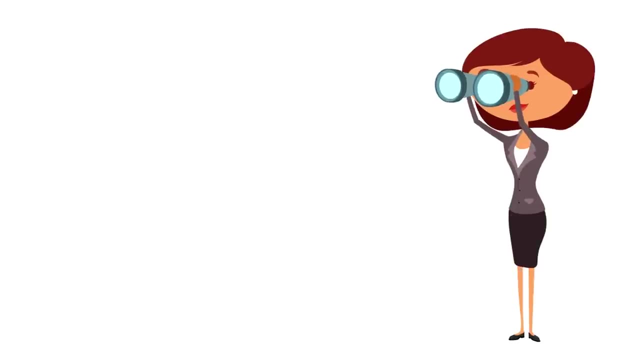 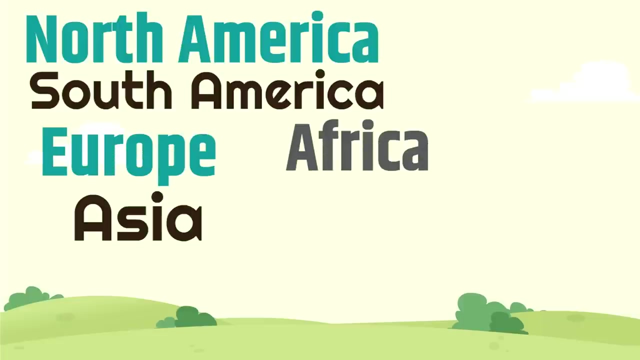 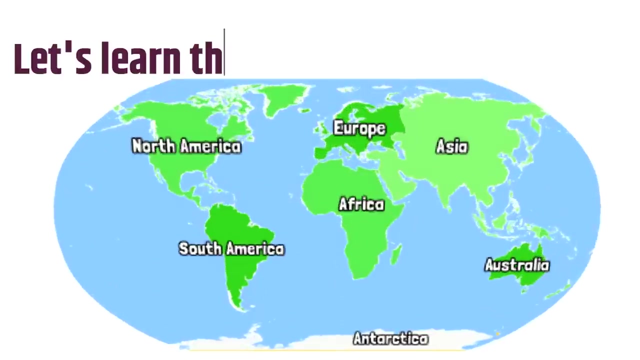 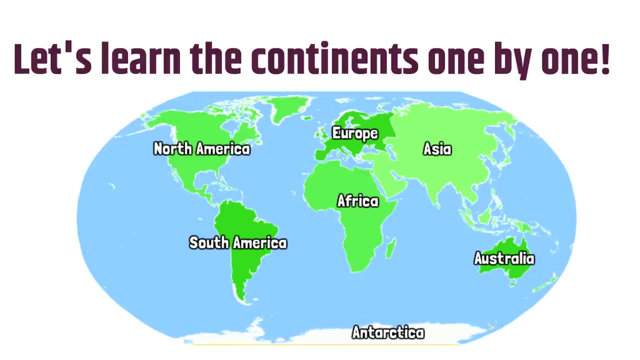 The world has seven continents. So how many continents are in the world? Yeah, seven. The names of the seven continents are North America, South America, Europe, Africa, Asia, Australia and Antarctica. So if you're ready, let's learn the continents one by one. 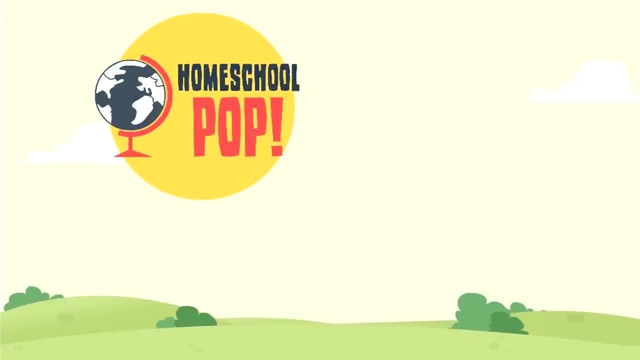 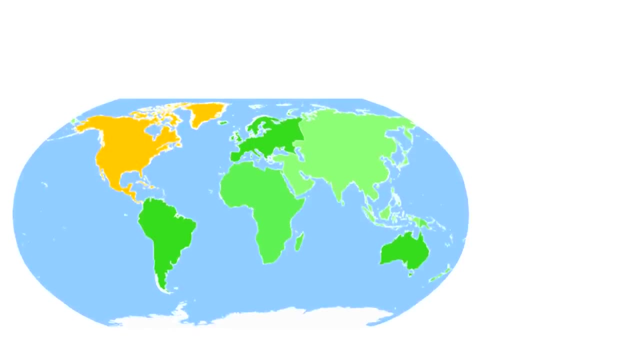 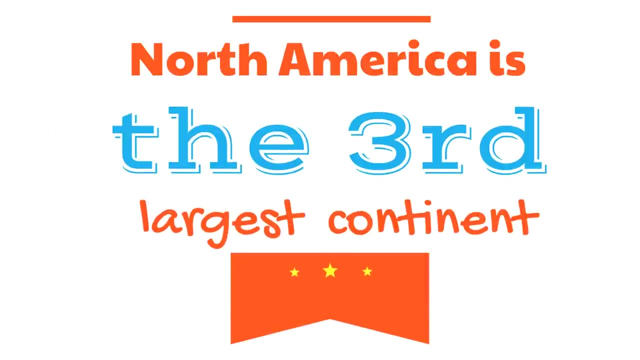 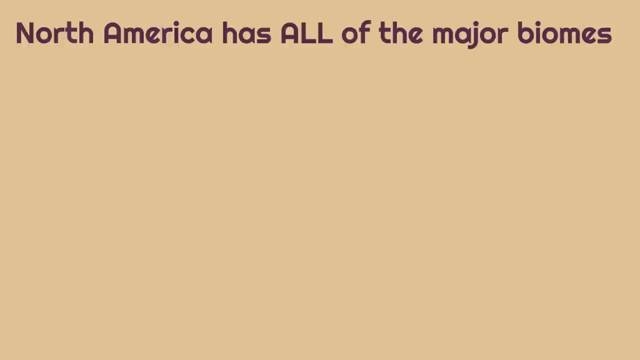 The first continent we're going to learn about today is Africa. The second continent is North America. North America is at the top left corner of most world maps And North America is the third largest continent. It's a pretty big continent And it's interesting. North America has all of the major biomes, including deserts, grasslands, forests, aquatic and tundra. 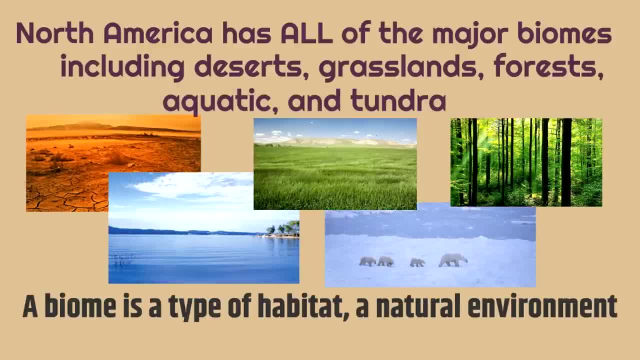 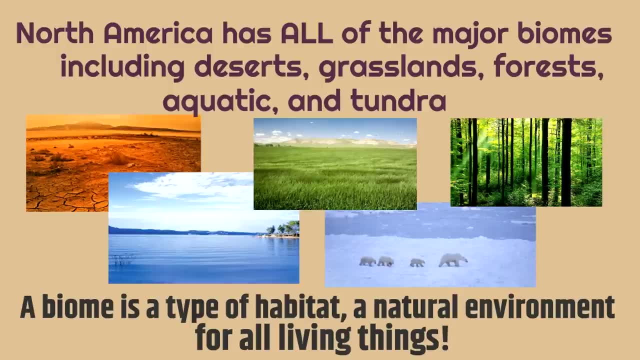 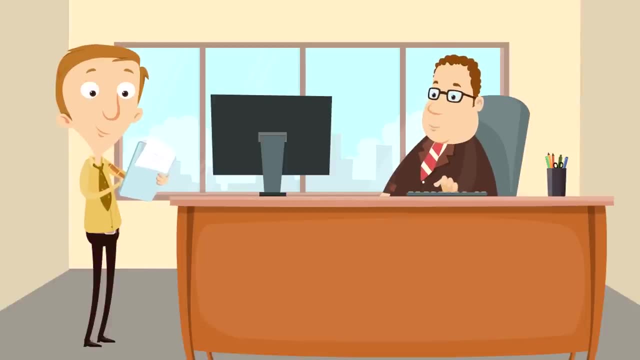 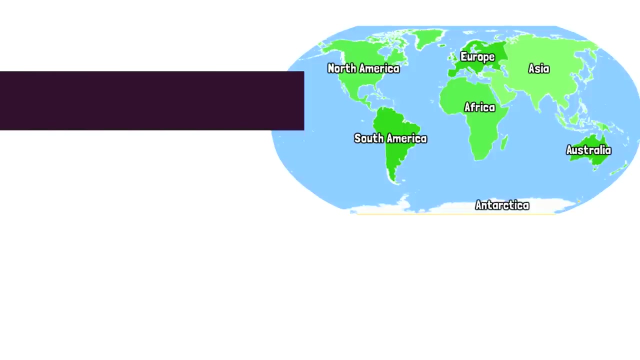 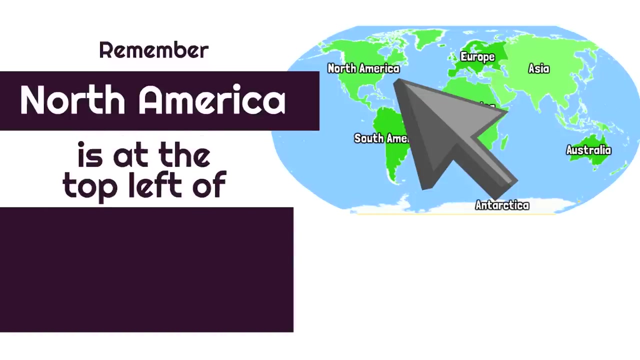 A biome is a type of habitat, a natural environment for all living things. Oh wait, Hold on a second. Okay, Remember, North America is at the top left of the world map. The next continent we're going to learn about is South America. 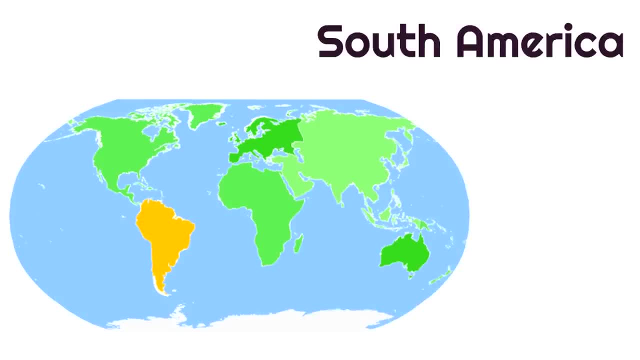 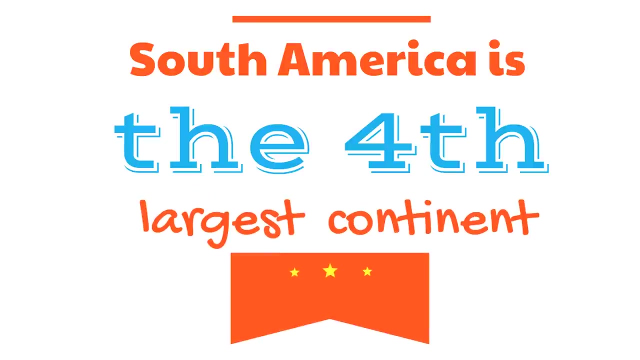 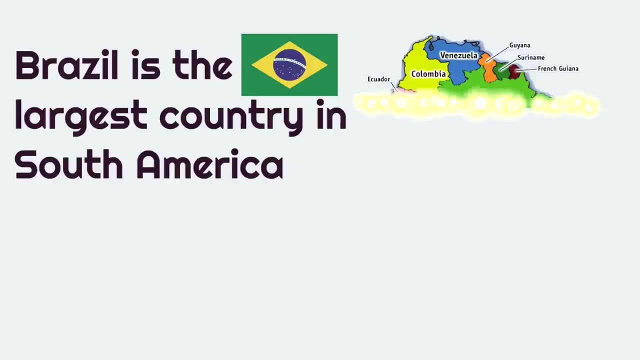 South America is at the bottom left corner of most world maps, just below North America. South America is the fourth largest continent. That means it's a medium-sized continent. The third largest continent is South America. Brazil is the largest country in South America. 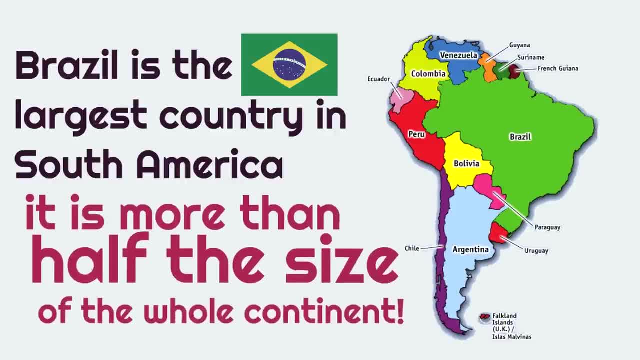 It is more than half the size of the whole continent. You can see Brazil is colored green on this map. Brazil is so big: it's almost the size of the United States of America. The third largest continent is South America. South America is home to the Amazon. 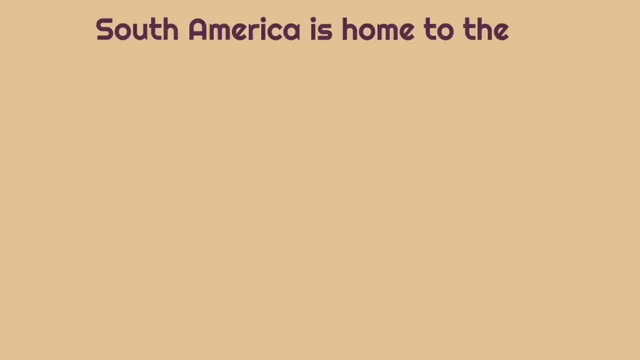 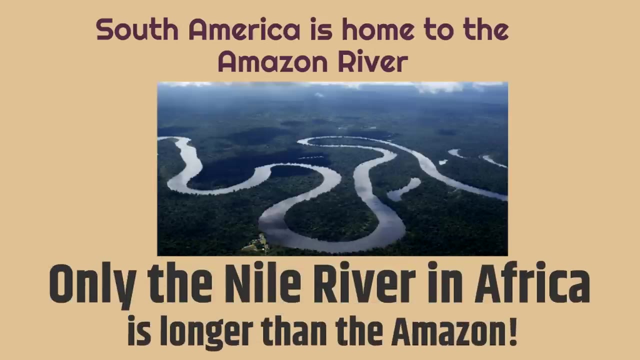 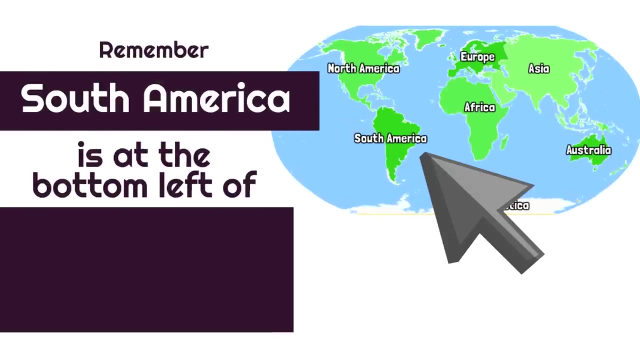 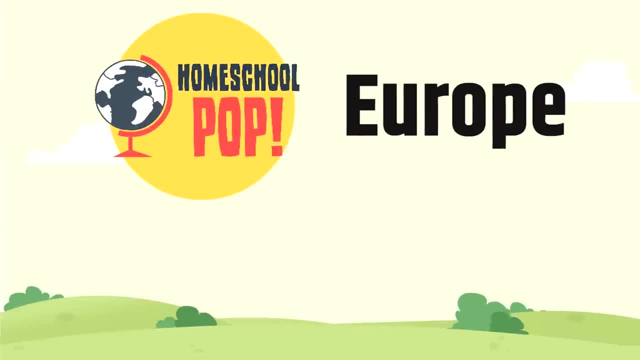 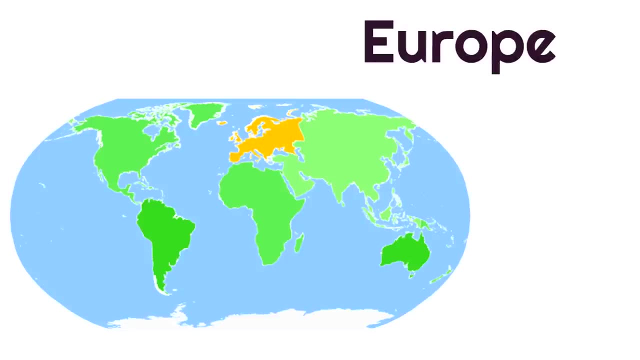 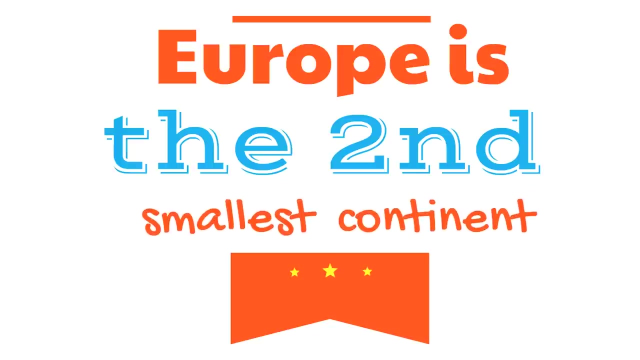 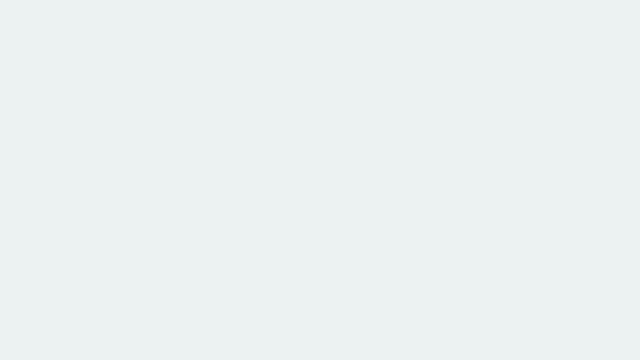 The next continent we're going to talk about is Europe. Europe is at the top middle of most world maps. Europe isn't a very big continent. In fact, Europe is the second smallest continent And, it's interesting, Europe is the only continent that does not have a desert biome. 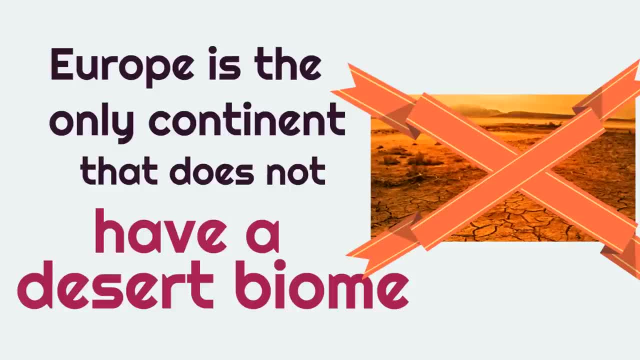 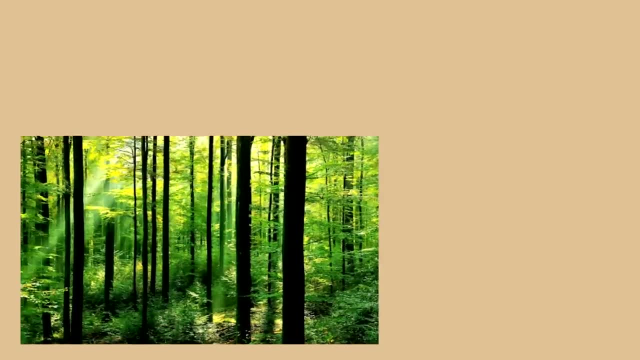 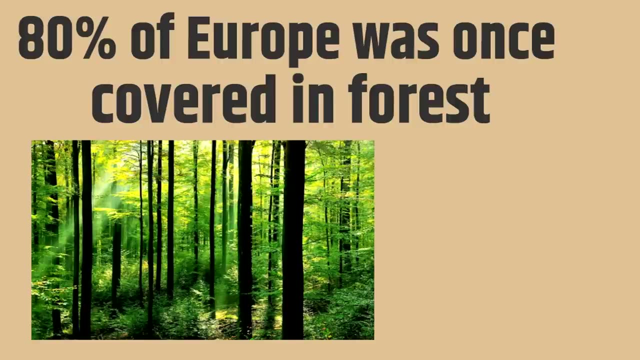 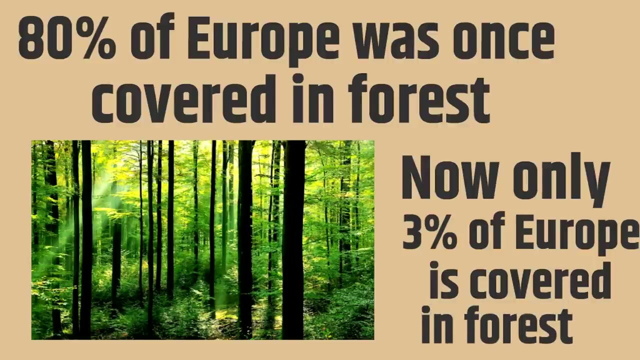 Remember, biome is a habitat, an environment for living things. Forests were the main biome of Europe. 80% of Europe was once covered in forests, But sadly now only 3% of Europe is covered in forests because so many of the trees have been cut down. 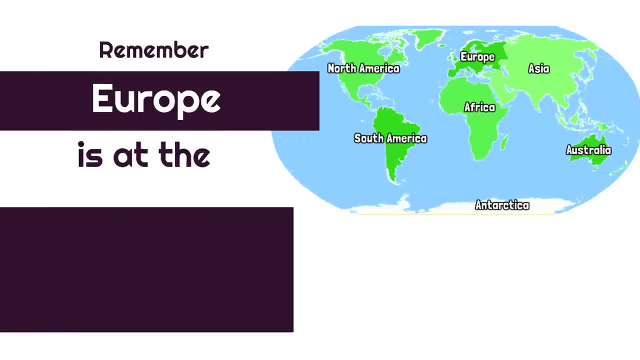 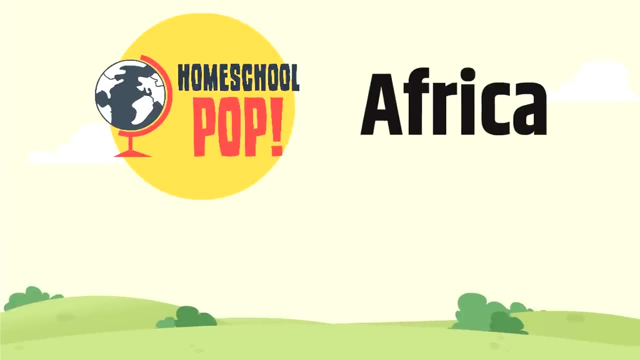 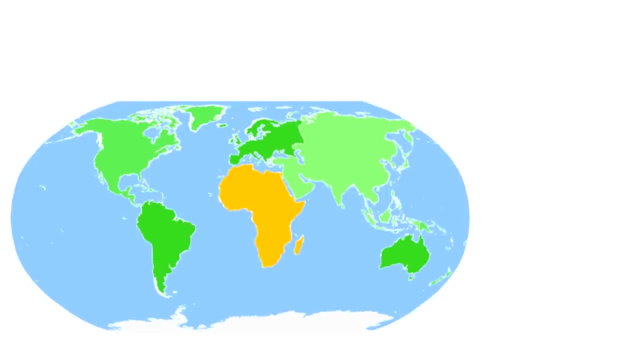 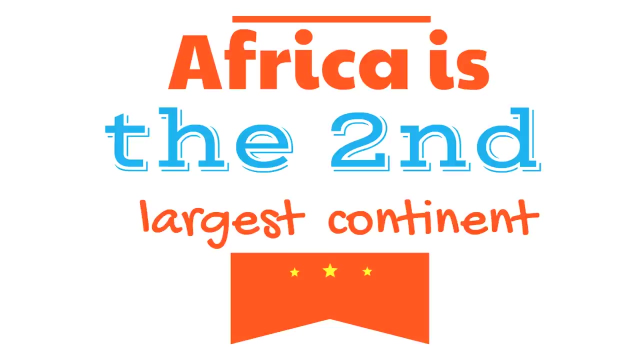 Remember, Europe is at the top middle of the world map. The next continent we're going to talk about is Africa. Africa is easy to find on the map because Africa is right in the middle of most world maps. Africa is the second largest continent. 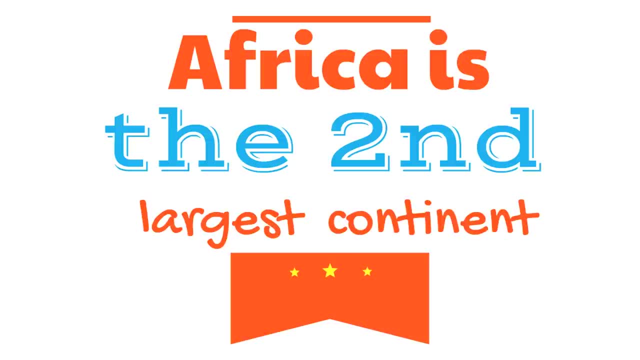 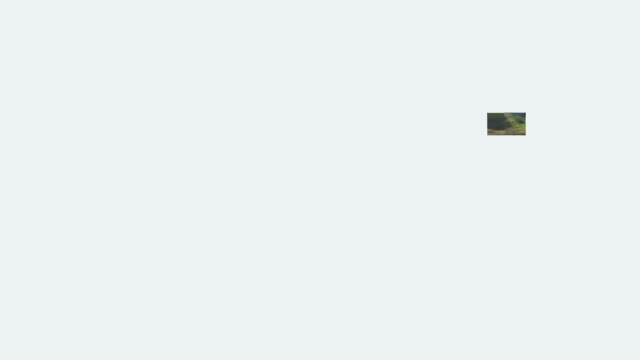 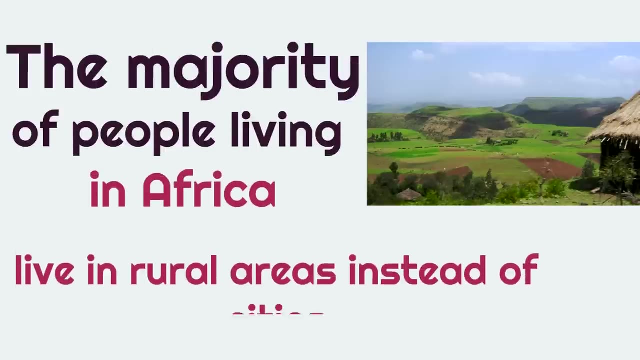 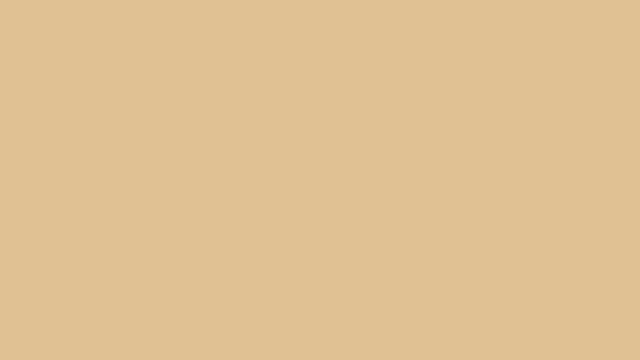 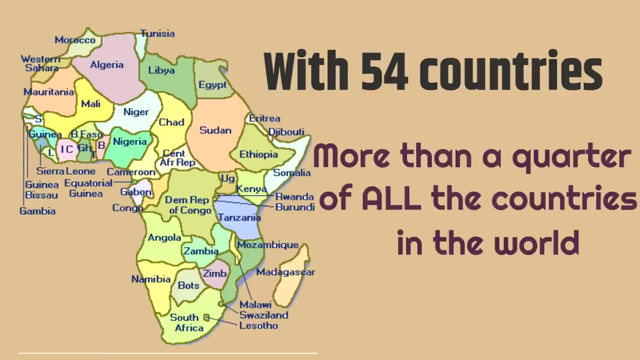 Africa is huge. While in many continents, much of the population are in urban areas, the majority of people living in Africa live in rural areas instead of cities, And this is interesting. with 54 countries, more than a quarter of all the countries in the world are in Africa. 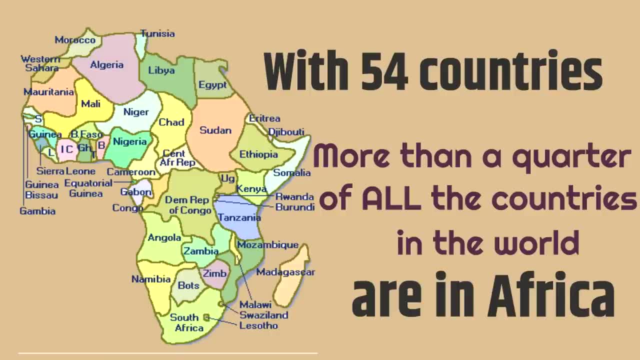 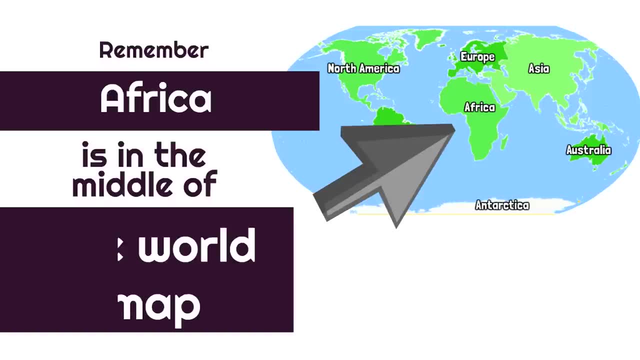 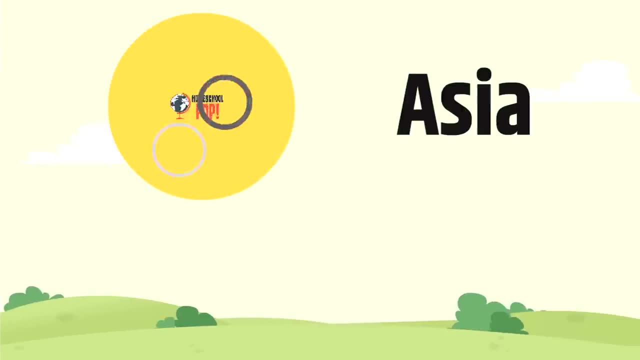 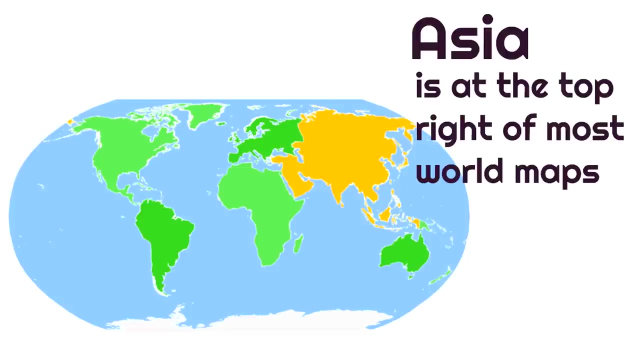 Remember, Africa is in the middle of the world map. The next continent we're going to talk about is Asia. Asia is at the top right of most world maps. Asia is at the top right of most world maps. Asia is the largest continent. 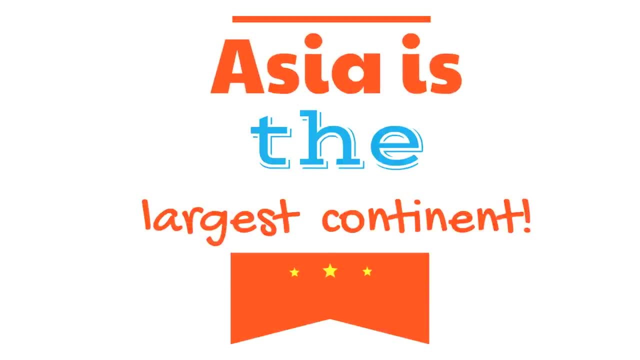 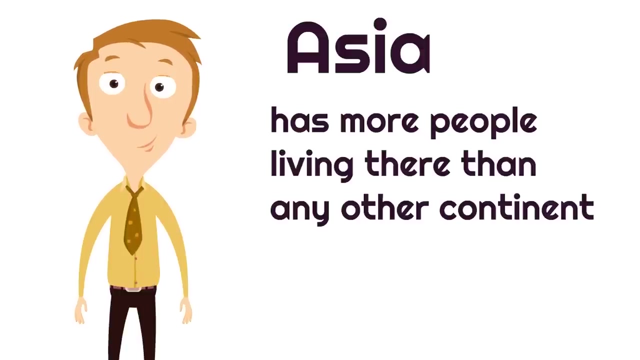 It's even larger than Africa. It's the biggest continent in the world. Asia has more people living there than any other continent. Over all, Over 4.2 billion people live in Asia. So not only is Asia the largest continent, but it also has the most people. 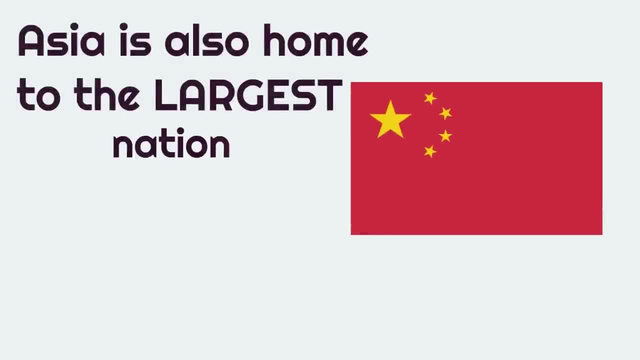 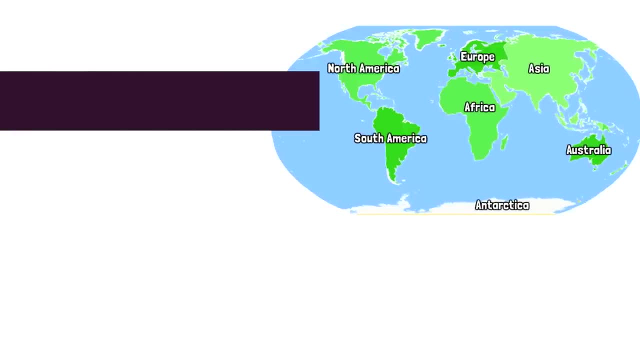 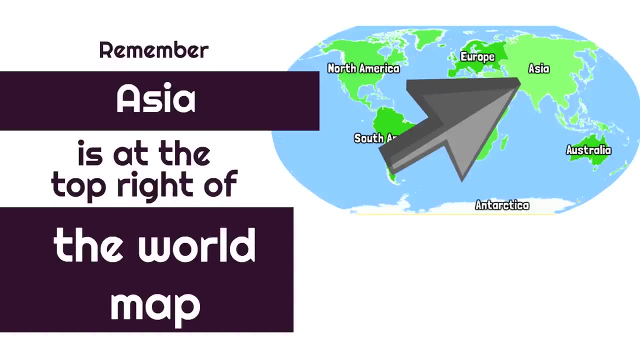 Asia is also home to the largest nation in the world, China. China is home to the largest nation in the world. Remember, Asia is at the top right of the world map. Asia is at the top right of the world map. Now it's time to talk about the next continent, Australia. 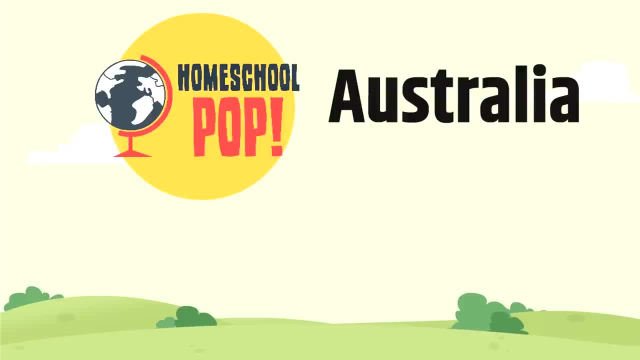 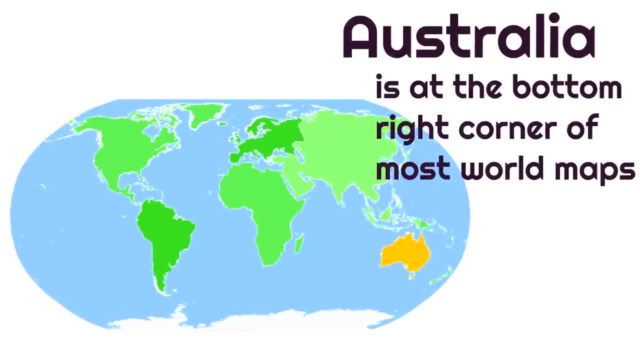 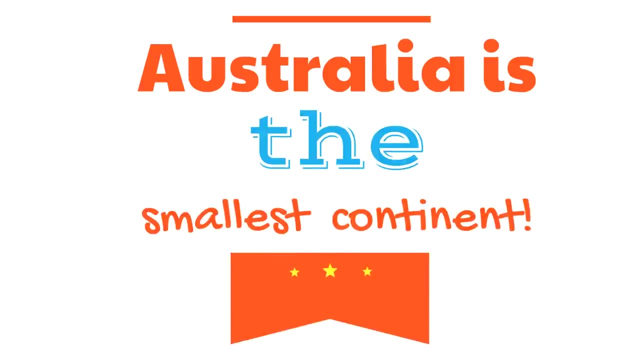 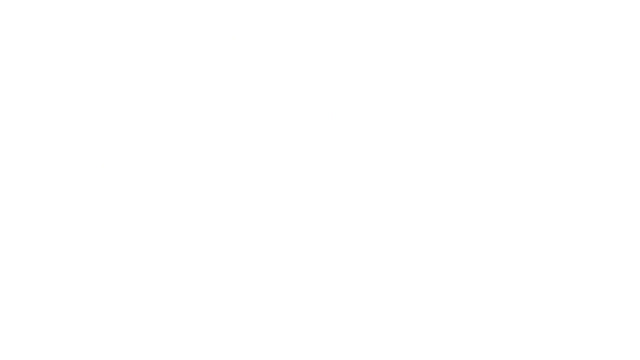 Next Continent, Australia. Australia is at the bottom right corner of most world maps. Australia is at the bottom right corner of most world maps. Australia is the smallest continent. Australia also has the fewest countries, Just one country. Can you guess what the country is? 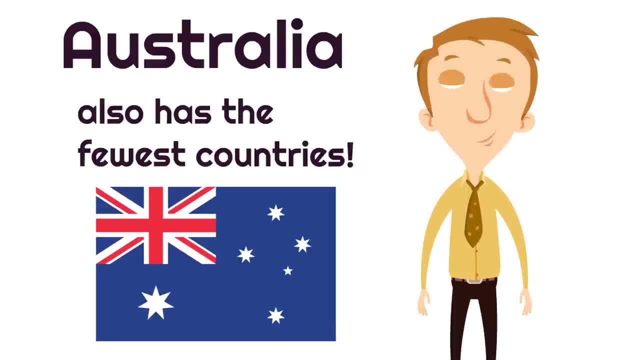 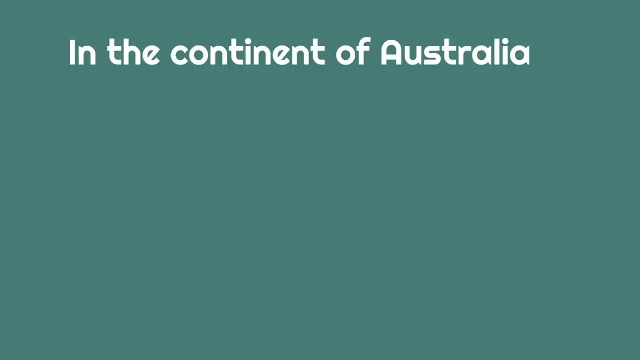 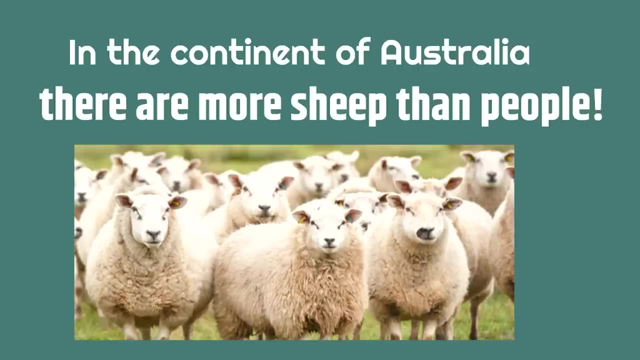 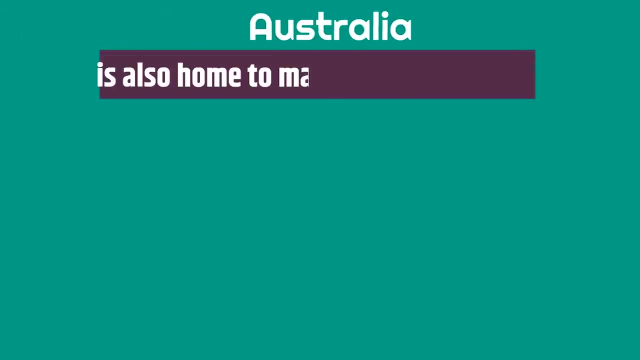 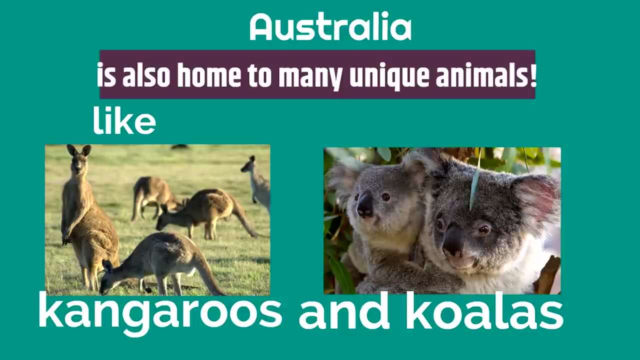 Yeah, The country of Australia. This is interesting. In the continent of Australia there are more sheep than people: tons and tons of sheep. Australia is also home to many unique animals like kangaroos and koalas. Remember, Australia is at the bottom right of the world map. 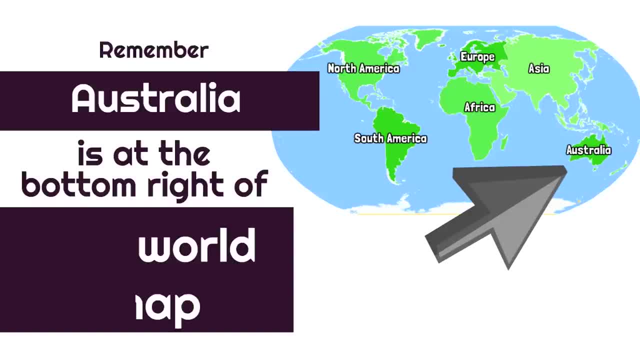 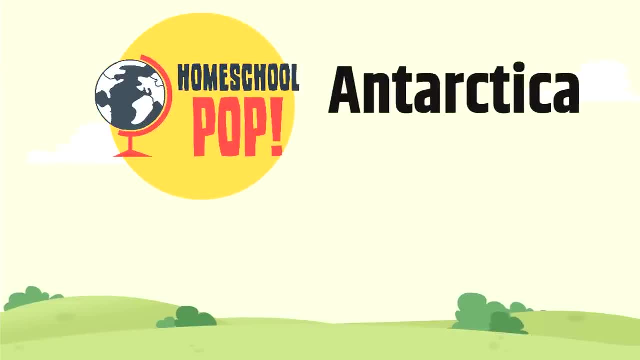 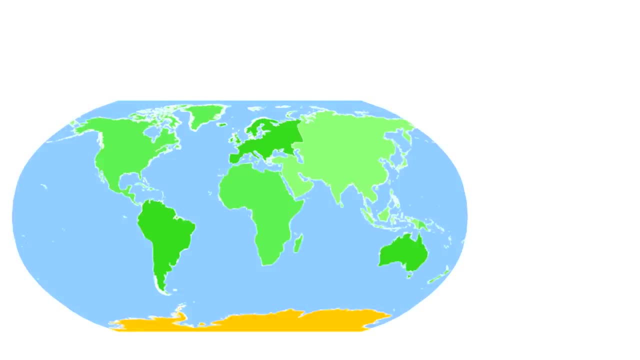 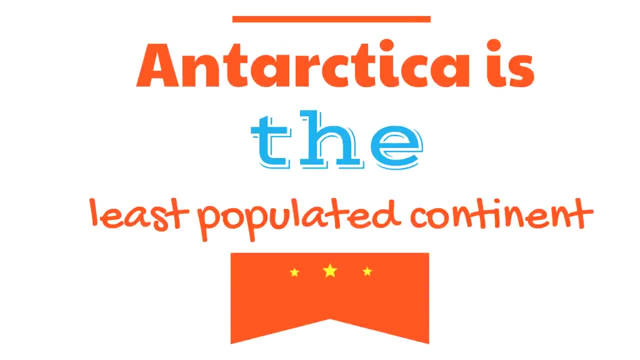 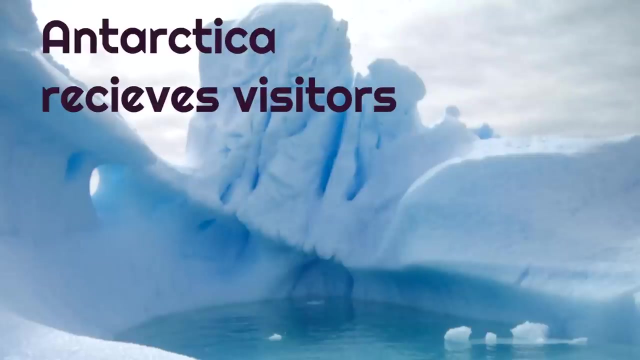 Our last continent is Antarctica. Antarctica is at the very bottom of most world maps. Antarctica is the least populated continent. It has the lowest population, Which means it is the most populated continent. Antarctica receives visitors, but has zero permanent residents. That means no one lives there full time. 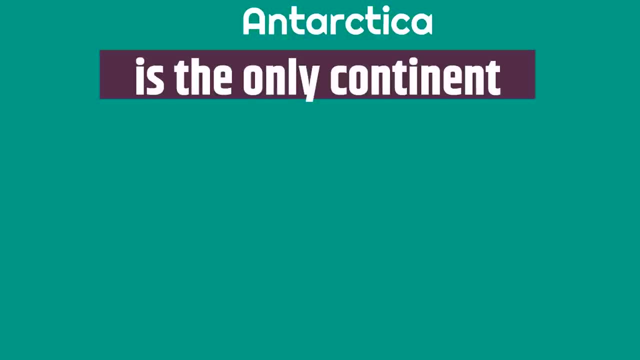 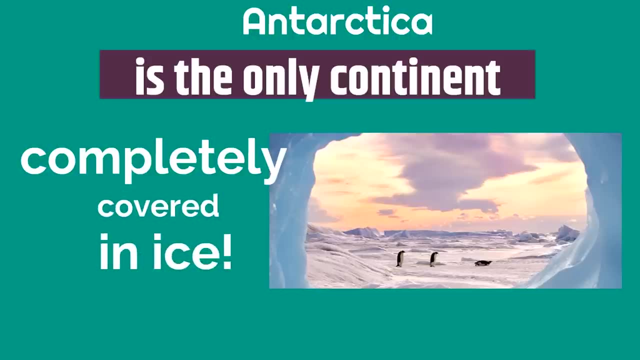 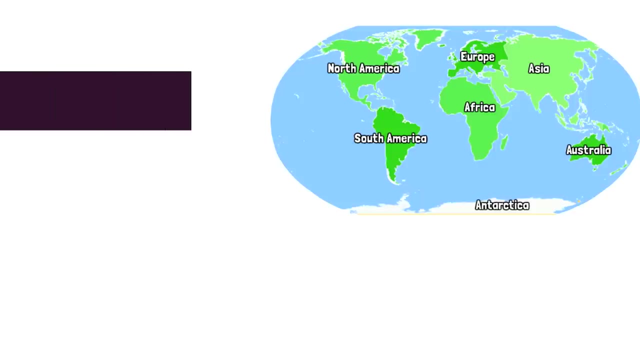 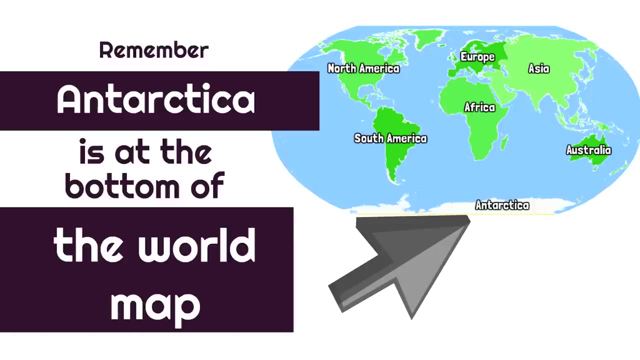 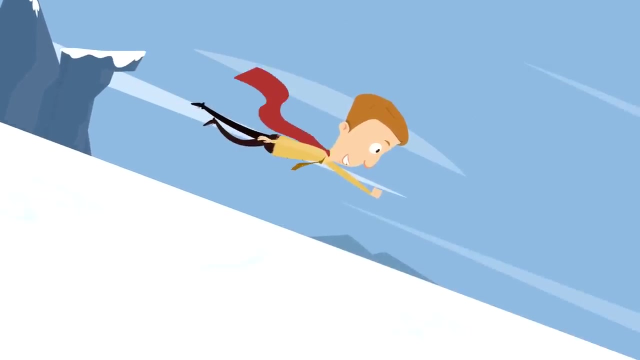 Antarctica is the only continent completely covered in ice. That means the only biome that Antarctica has has is the tundra biome. remember, Antarctica is at the bottom of the world map. you've done such a great job. now it's time to put you to the test and see how. 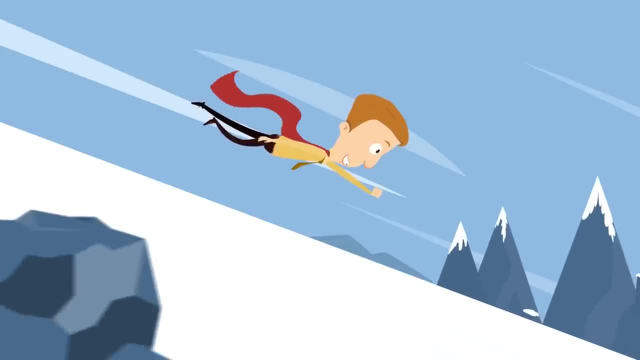 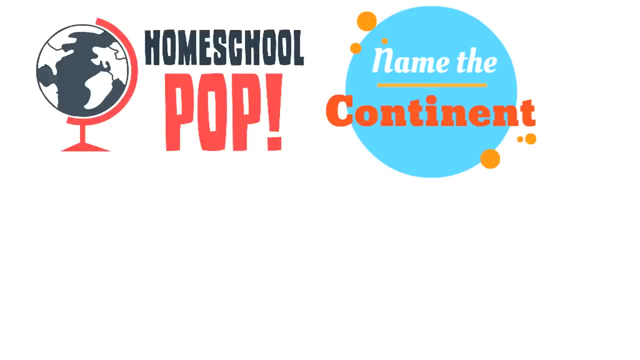 much you learned. we're going to play a quick game called name the continent, where you're going to see the continent on the map and you're going to tell us which continent you think it is. here's the first one. look at the yellow region. which continent is that? 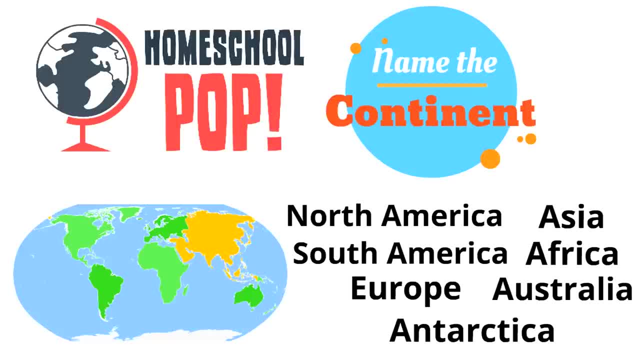 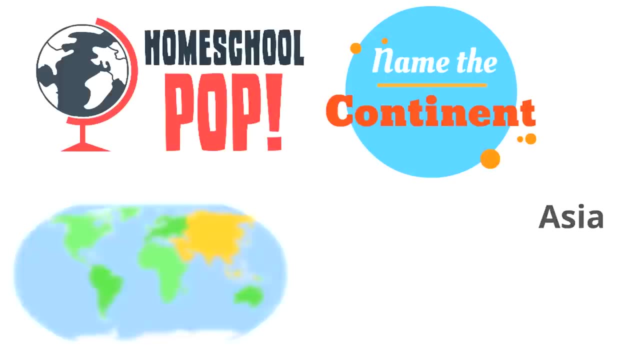 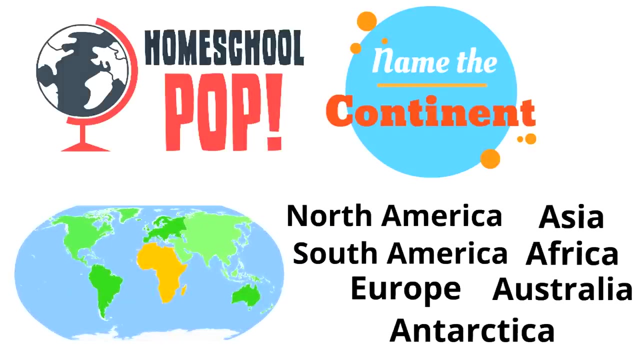 you've done such a great job. now it's time to put you to the test and see how much you learned. you can see the seven choices. just go ahead and say it out loud: yeah, it's Asia. how about this one? which continent is the yellow region? it's right in the 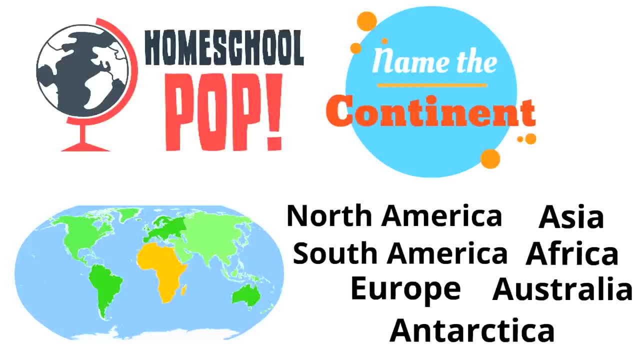 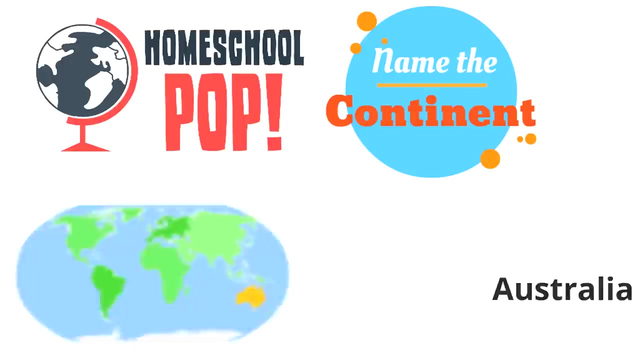 middle of the map. yeah, it's Africa. all right now. look at the continent colored yellow in this one way, at the bottom right corner of the world map. which continent is it? all right, Australia, how about this one? look at the yellow region. it's way at the bottom on this. 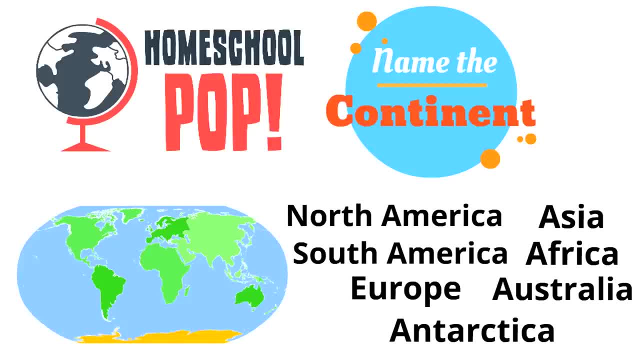 one. which continent is it? do you have an idea? yeah, Antarctica. yeah, I would say this is the continent. that's really like an interesting one. Here's another one. Look at the yellow continent. Which continent is it? Uh huh, It's South America. 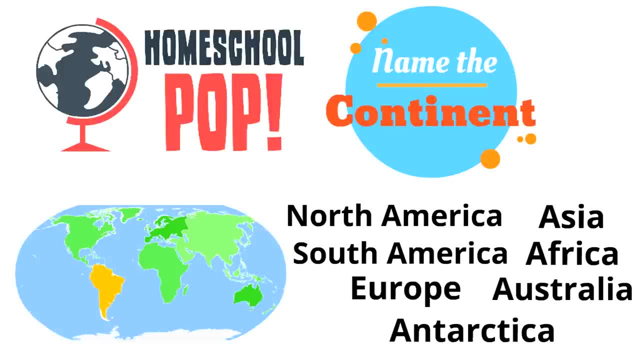 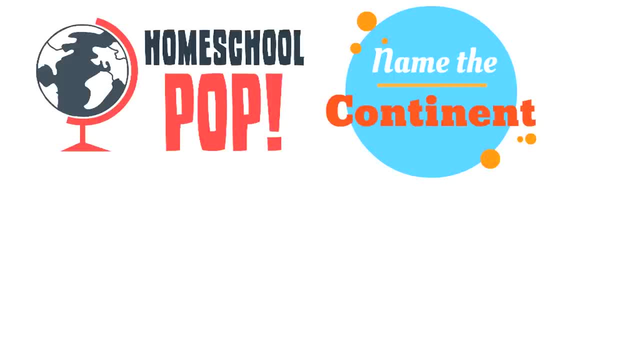 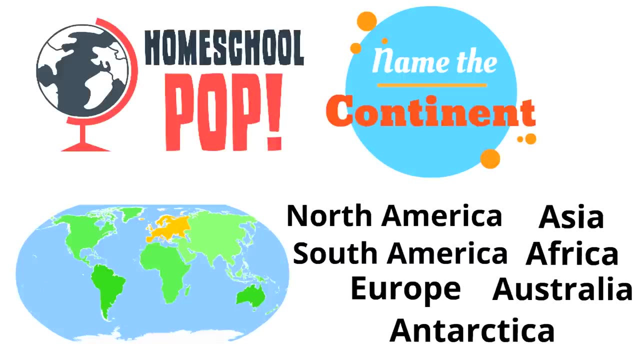 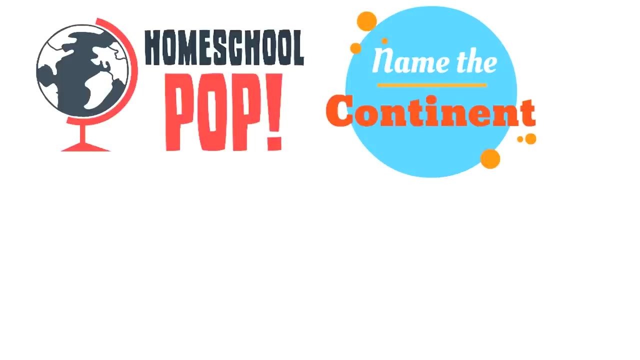 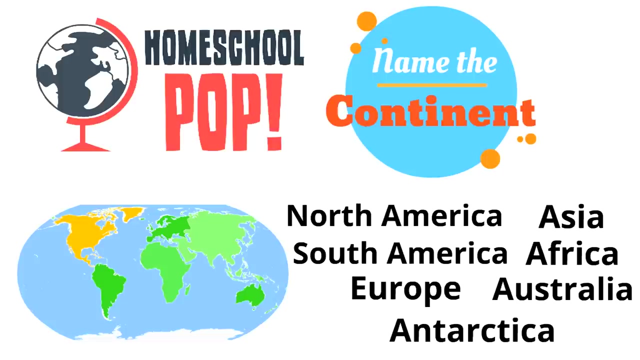 Great job. Here's another one. Which continent is the yellow continent? It's in the top, middle of the map. Yeah, it's Europe. Here's our final one. Look at the yellow continent. Which continent is it? Yes, North America. 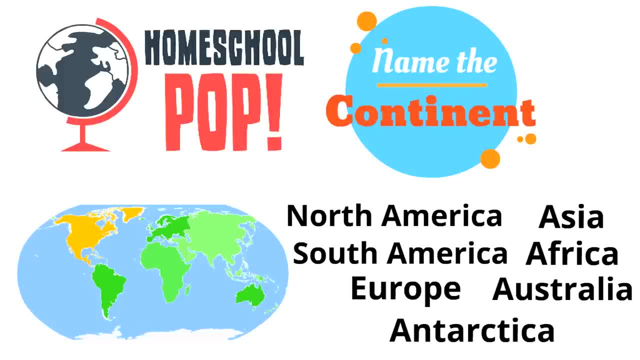 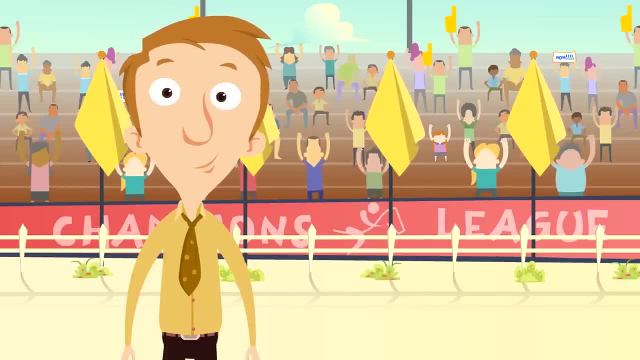 Awesome job, Awesome job. Well, that's all for the continents. We appreciate you playing the game with us and learning with us, And next time somebody asks you about the continents, you'll know all seven of them, Hey, Petey. 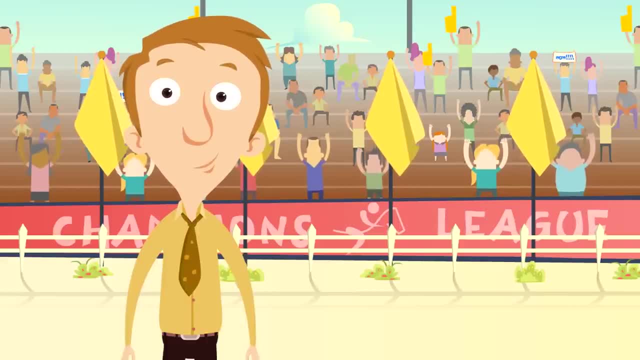 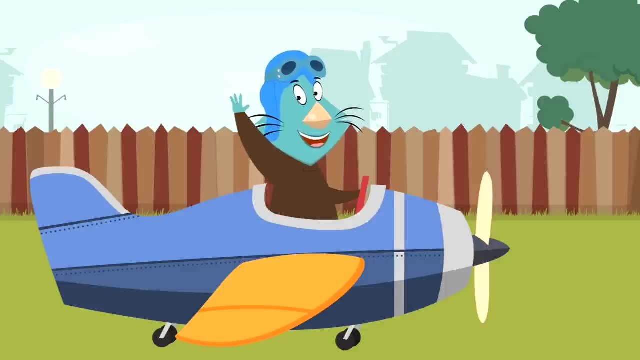 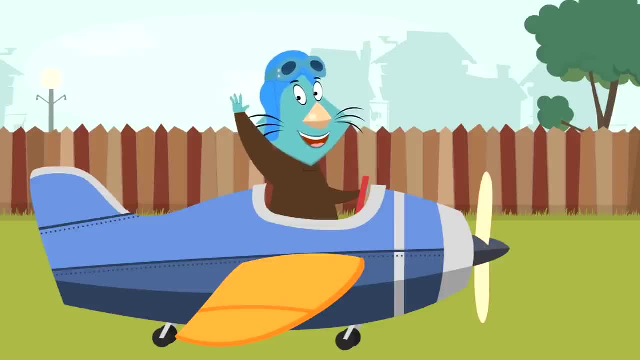 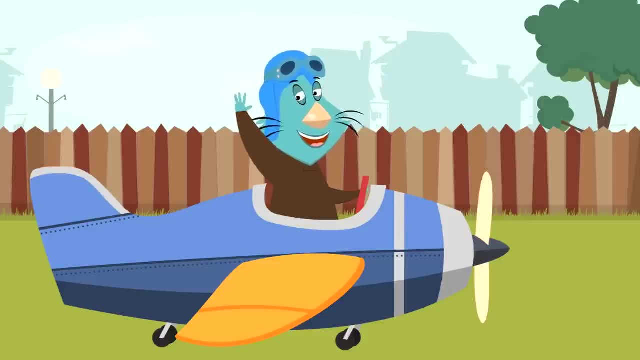 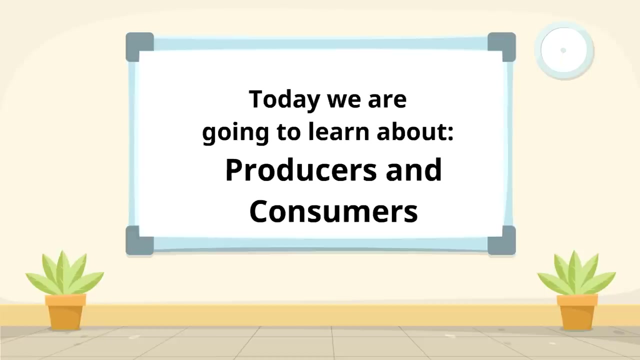 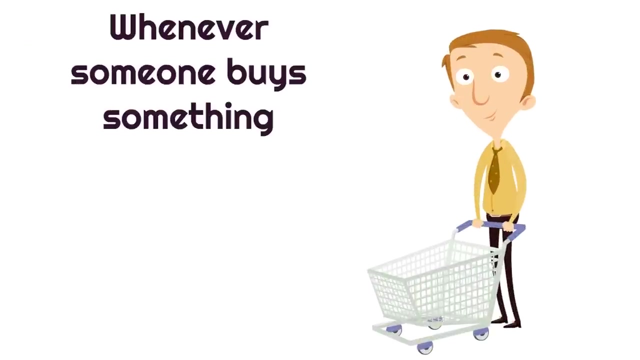 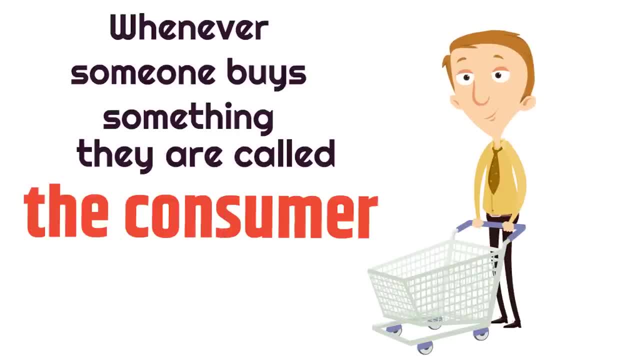 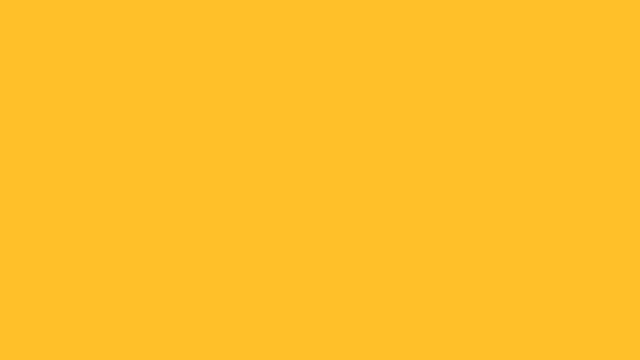 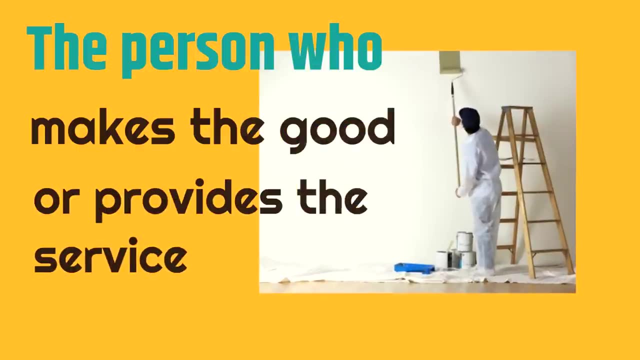 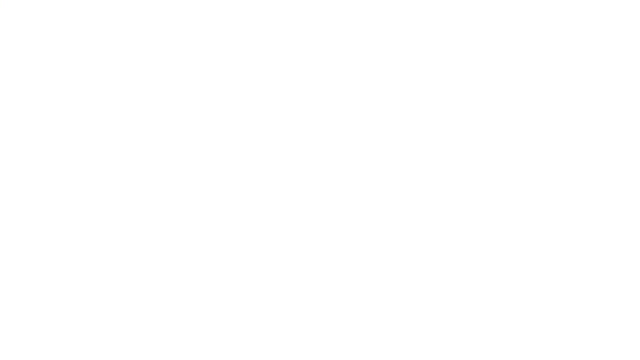 are called the consumer. the consumer is the one who buys the good or the service. now, the person who makes the good or provides the service is called the producer. the person who makes the good or provides the service is called the producer. the person who makes or provides the good or service is the. 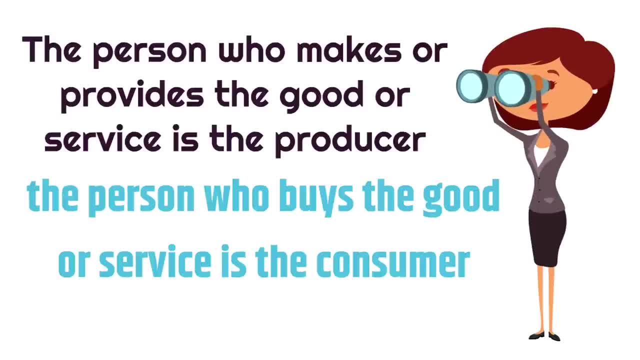 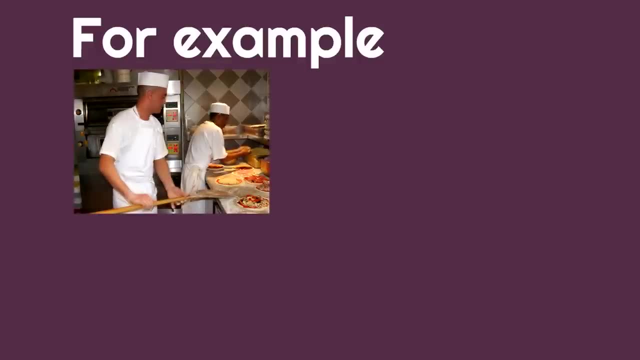 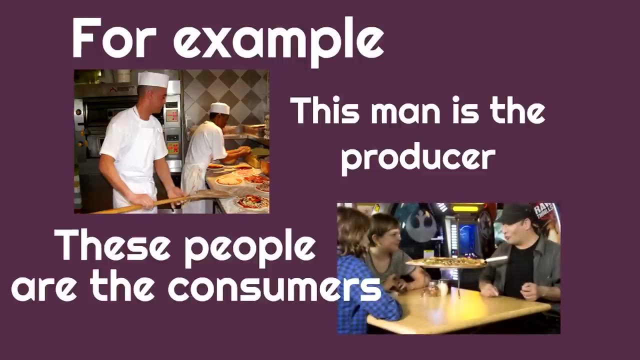 producer and the person who buys the good or service is the consumer. so the producer makes it, the consumer buys it. for example, here's a picture of a man who's making a pizza. this man is the producer. now see these people. these people are the consumers, they are the. 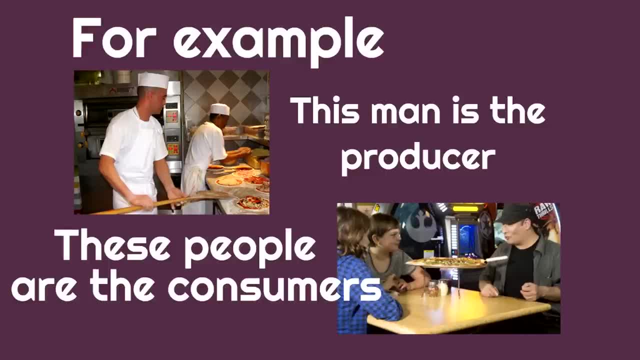 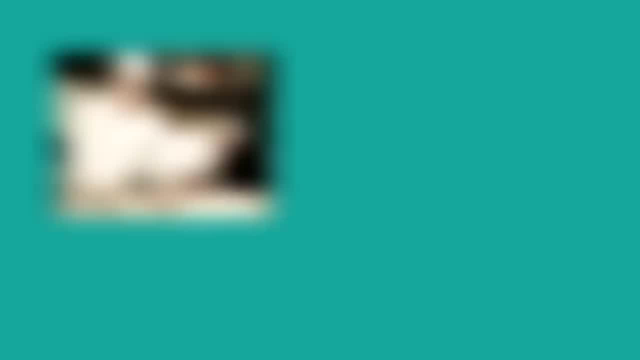 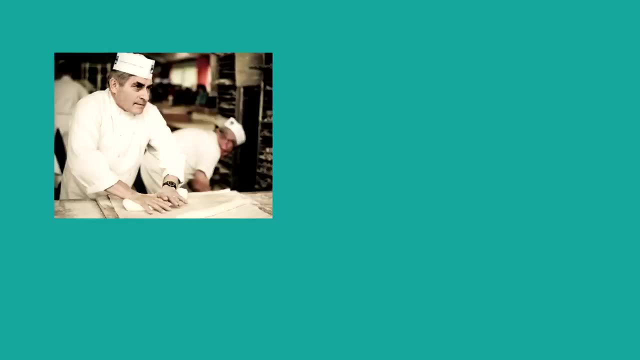 ones that bought the pizza. the producer made the pizza. the consumers buy the pizza. here's a man who's working very hard. he's making bread now I need to. here's a man who's working very hard. he's making bread now I need to your help on this one. do you think this man is a producer or consumer? he's. 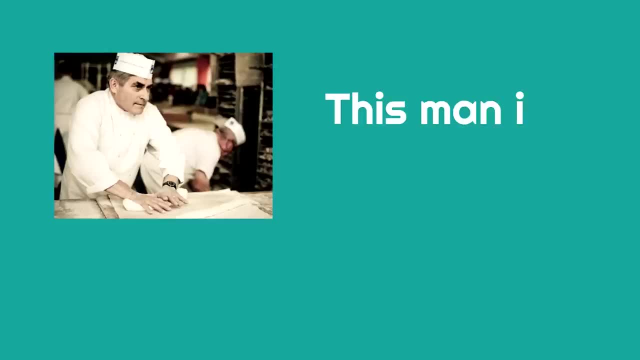 your help on this one. do you think this man is a producer or consumer? he's making the bread. this man is the producer. he's the one that's making the making the bread. this man is the producer. he's the one that's making the bread. now, see this lady. do you think this lady is the producer or the? 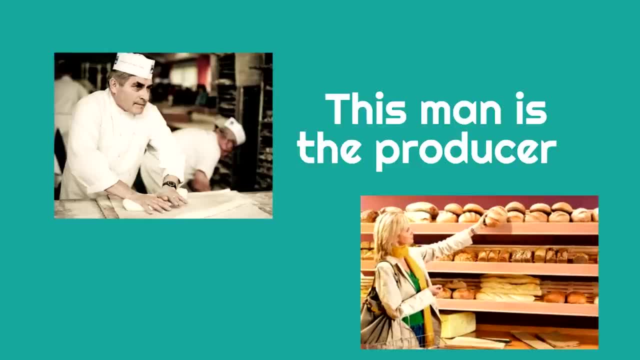 bread. now see this lady. do you think this lady is the producer or the consumer? yeah, this lady is the consumer. she's going to buy the bread consumer consumer. yeah, this lady is the consumer, she's going to buy the bread consumer. yeah, this lady is the producer, she's going to buy the bread. the baker made the bread, but this lady is. 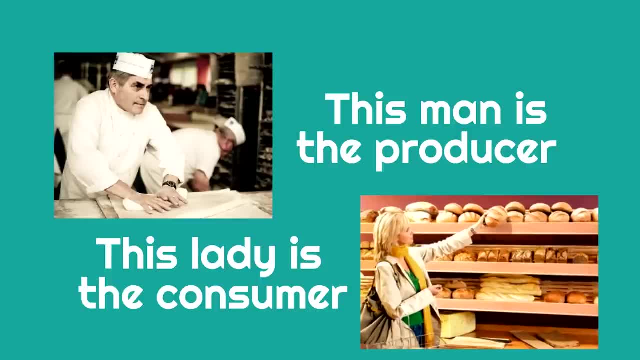 the baker made the bread, but this lady is. the baker made the bread, but this lady is going to buy the bread. she is the going to buy the bread. she is the going to buy the bread. she is the consumer. look at this picture. it's a lady. 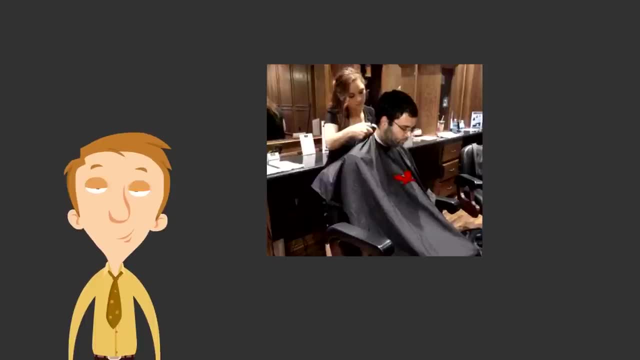 consumer. look at this picture: it's a lady consumer. look at this picture: it's a lady giving a haircut to this man. now, what? giving a haircut to this man now? what? giving a haircut to this man? now? what do you think the lady is? is the lady the? 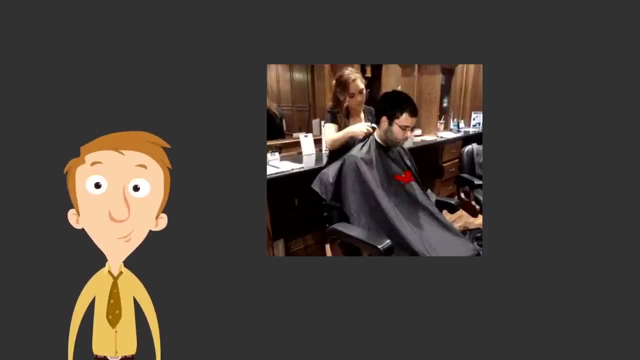 do you think the lady is? is the lady the? do you think the lady is? is the lady the producer or is the lady the consumer the producer? or is the lady the consumer the producer or is the lady the consumer? the lady is the one giving the haircut. yeah, 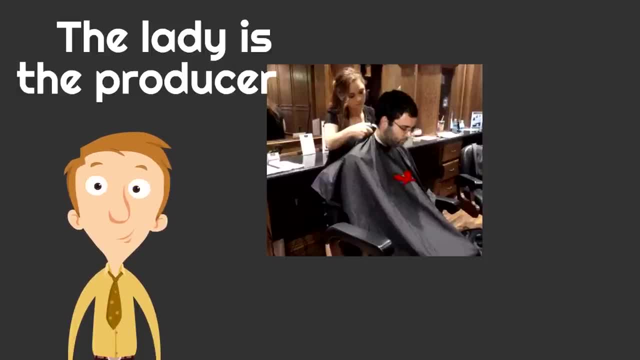 lady is the one giving the haircut. yeah, lady is the one giving the haircut. yeah, the lady is the producer, now the man. the lady is the producer, now the man. the lady is the producer. now the man sitting in the chair. is he the consumer sitting in the chair? is he the consumer? 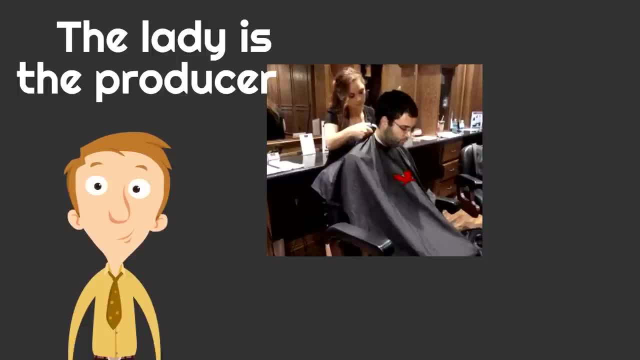 sitting in the chair. is he the consumer or the producer? he's the one buying the or the producer he's the one buying the, or the producer he's the one buying the haircut? yeah, the man is the consumer. the one who buys the good or service is. 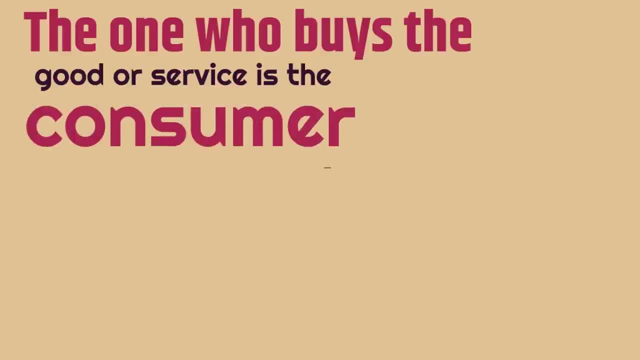 the one who buys the good or service is. the one who buys the good or service. is the consumer, the one who provides the. the consumer, the one who provides the. the consumer, the one who provides the good or service. good or service, good or service- is the consumer. the one who provides the good or service is. 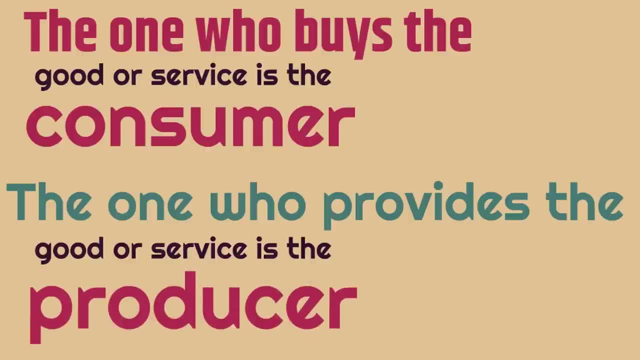 is the consumer the one who provides the good or service is. is the consumer the one who provides the good or service is the producer. you might the producer, you might the producer. you might not know this, but did you know? even kids not know this, but did you know? even kids? 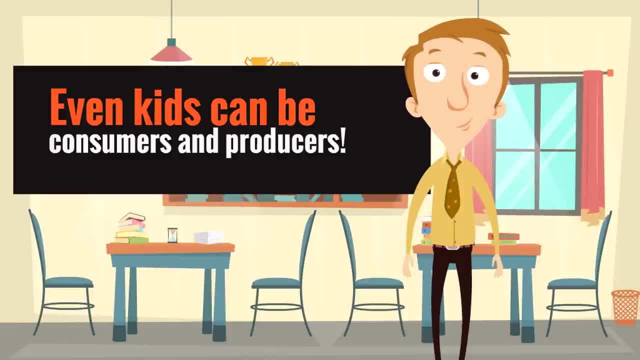 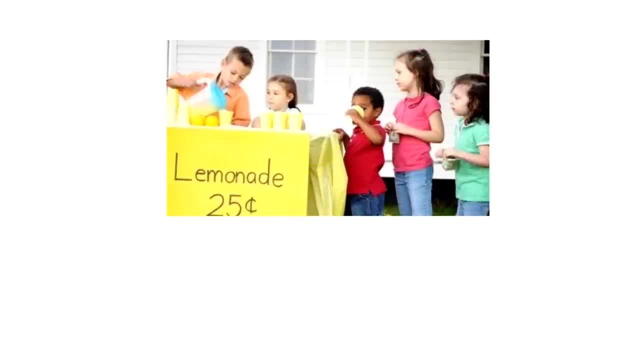 not know this, but did you know? even kids can be consumers and producers. how cool can be consumers and producers. how cool can be consumers and producers. how cool is that here? we've got a picture for you. is that here? we've got a picture for you. is that here? we've got a picture for you to look at and we're gonna need your. 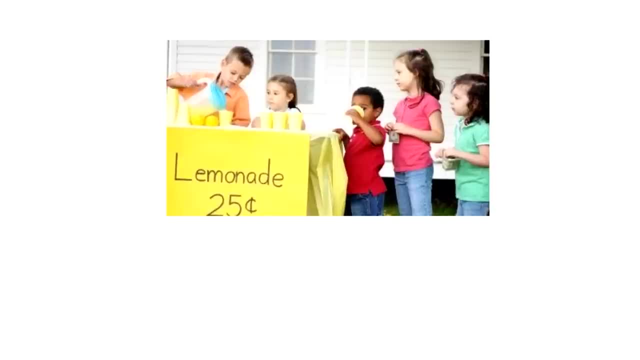 to look at and we're gonna need your to look at and we're gonna need your help. you see, in this picture, the kids help. you see in this picture, the kids help. you see in this picture the kids are either producers or consumers. are either producers or consumers. 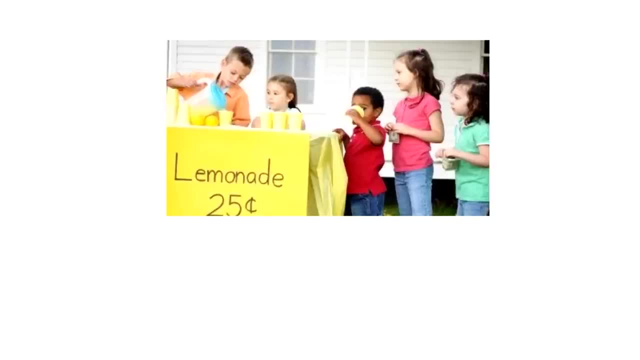 are either producers or consumers. wonder if you could help me figure out. wonder if you could help me figure out. wonder if you could help me figure out how many are producers and how many are. how many are producers and how many are. how many are producers and how many are consumers. so how many of these kids are? 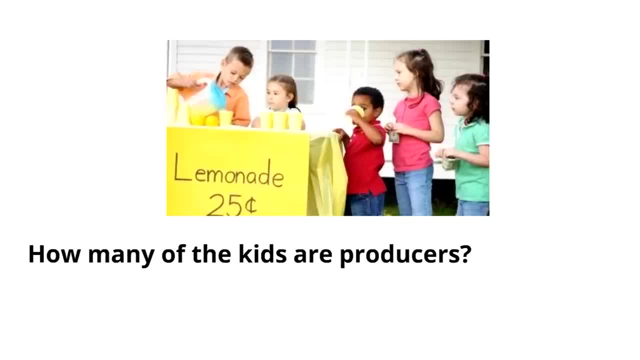 consumers. so how many of these kids are consumers? so how many of these kids are producers? this is a picture of a producers. this is a picture of a producers. this is a picture of a lemonade stand. how many of the kids are lemonade stand? how many of the kids are? 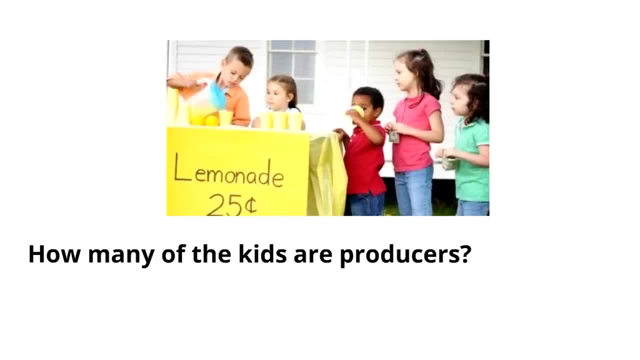 lemonade stand. how many of the kids are producers? yeah, two. two of them are producers? yeah, two. two of them are producers? yeah, two. two of them are producers- now this might be easier. how producers? now this might be easier. how producers- now this might be easier. how many of the kids are consumers? how many? 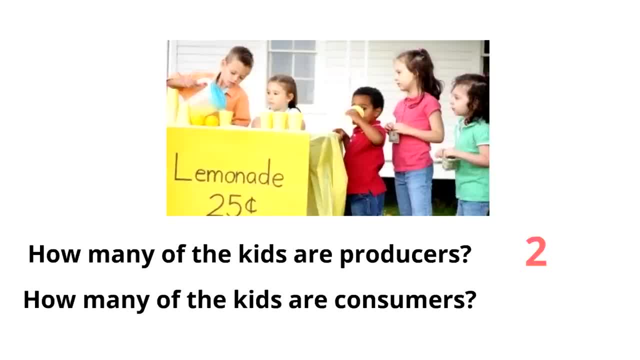 many of the kids are consumers. how many many of the kids are consumers? how many of them are gonna buy the lemonade? yeah of them are gonna buy the lemonade. yeah of them are gonna buy the lemonade. yeah, three now. do you remember the last time? 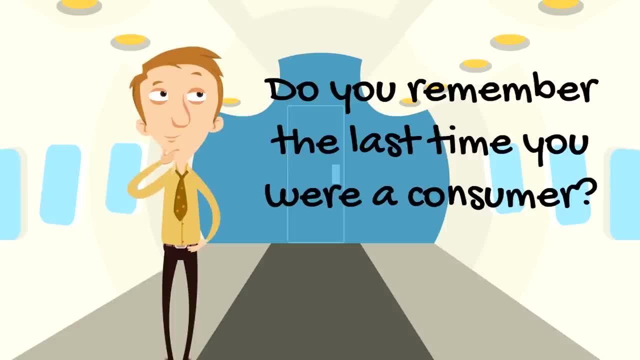 three now. do you remember the last time? three now. do you remember the last time you were a consumer? think about it for a. you were a consumer. think about it for a: you were a consumer. think about it for a moment: when was the last time you bought? 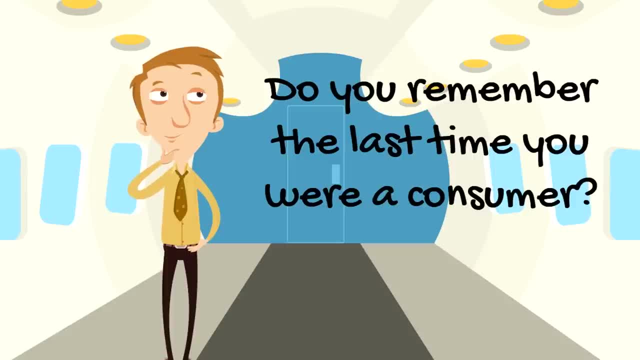 moment? when was the last time you bought moment? when was the last time you bought a good or a service? when was the last a good or a service? when was the last a good or a service? when was the last time you were a consumer? it probably. time you were a consumer, it probably. 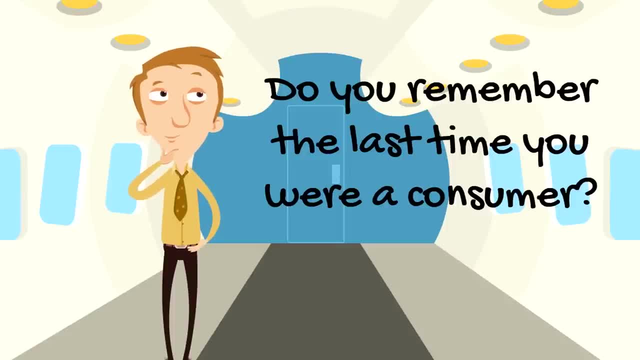 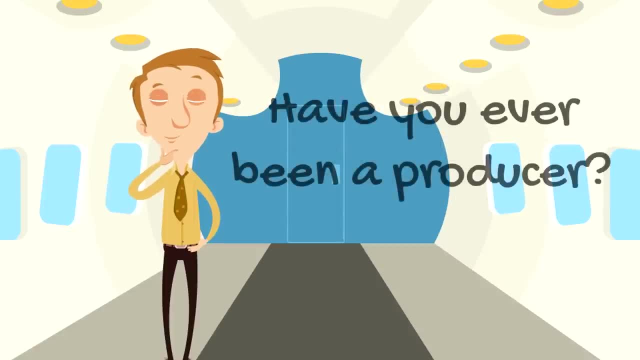 time you were a consumer? it probably wasn't that long ago. we buy goods and wasn't that long ago. we buy goods and wasn't that long ago. we buy goods and services- all the time me. services, all the time me, services, all the time me now. have you ever been a producer? many? 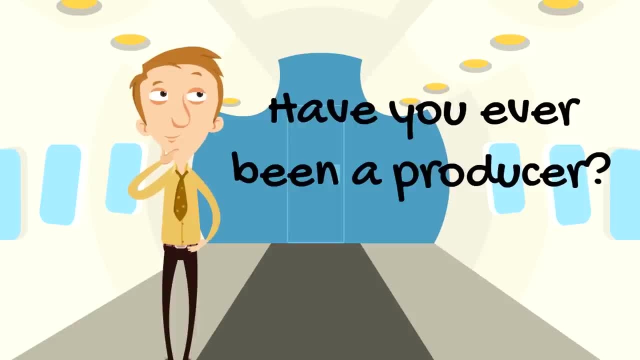 now have you ever been a producer? many now have you ever been a producer? many kids haven't been producers before. but kids haven't been producers before. but kids haven't been producers before. but you may have been a common example of. you may have been a common example of 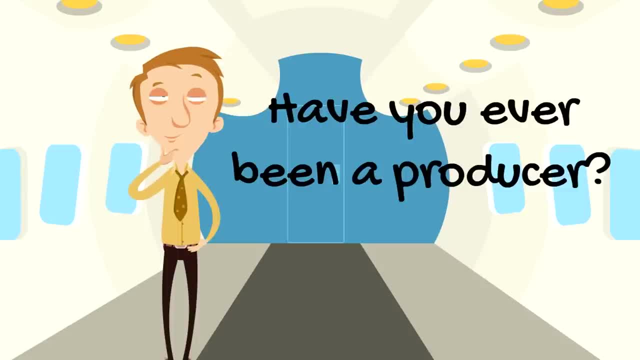 you may have been a common example of kids being a producer is at a lemonade. kids being a producer is at a lemonade. kids being a producer is at a lemonade stand. have you ever been a producer stand? have you ever been a producer stand? have you ever been a producer? it's fun. you might want to try it out. 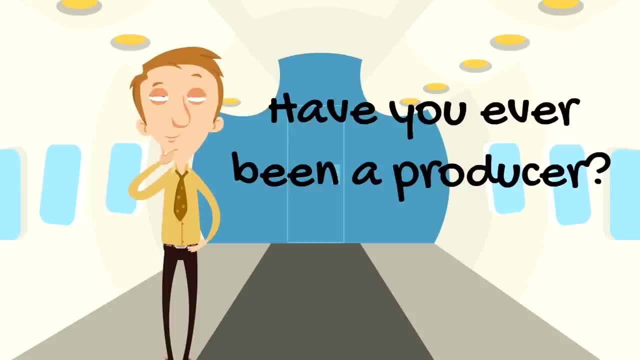 it's fun, you might want to try it out. it's fun, you might want to try it out sometime. remember the one who buys sometime. remember the one who buys sometime. remember the one who buys the good or service is the consumer, the one. the good or service is the consumer: the one. 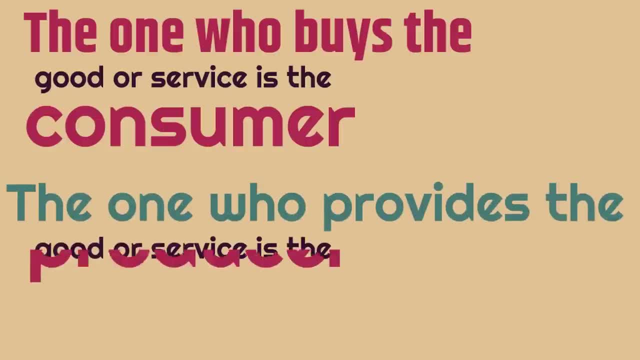 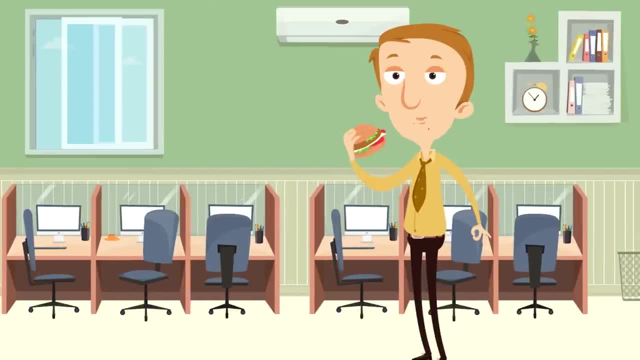 the good or service is the consumer, the one who provides the good or service is. who provides the good or service is who provides the good or service is the producer. so the next time you're a consumer, you. so. the next time you're a consumer, you. so the next time you're a consumer, you buy something like a burger or a toy, or 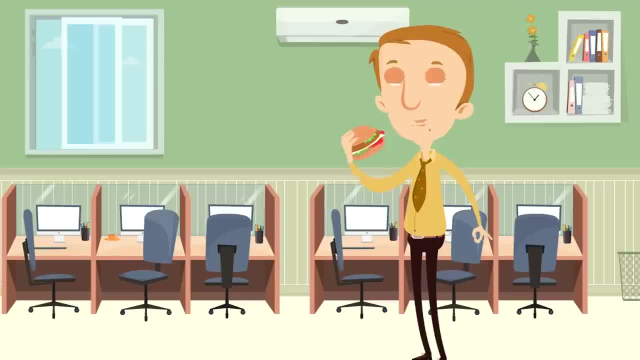 buy something like a burger or a toy. or buy something like a burger or a toy, or a piece of gum or a haircut? you can know a piece of gum or a haircut. you can know a piece of gum or a haircut. you can know, hey, I was a consumer and you can point. 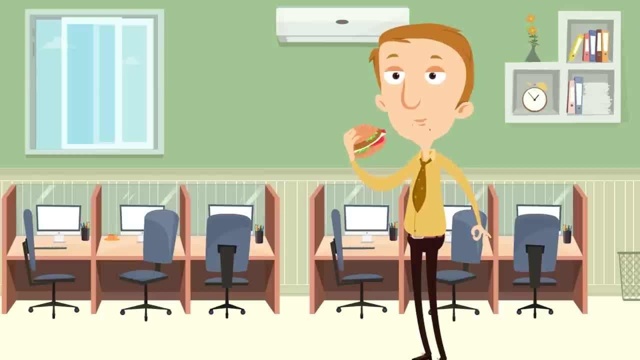 hey, I was a consumer and you can point, hey, I was a consumer. and you can point to the person who provided and say thank to the person who provided, and say thank to the person who provided and say thank you, thank you for being such a great you, thank you for being such a great. 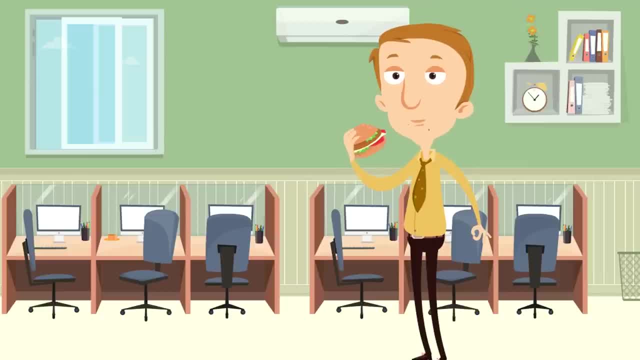 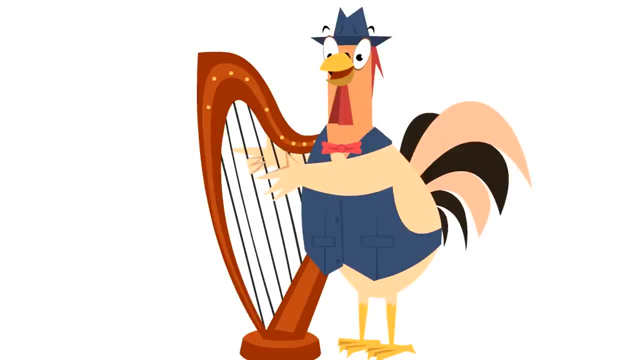 you. thank you for being such a great producer. here's our friend Fred. we heard that he. here's our friend Fred. we heard that he. here's our friend Fred. we heard that he just took up the harp. he just started. just took up the harp, he just started. 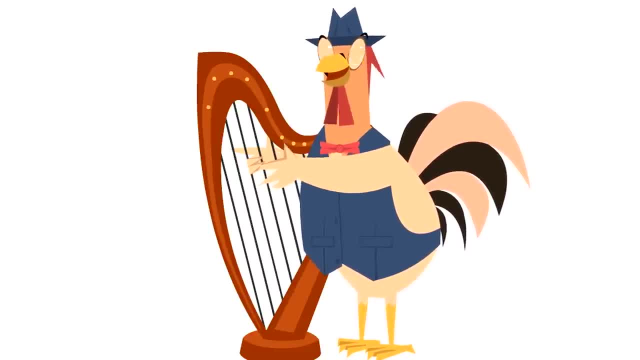 just took up the harp. he just started playing the harp Fred. we can't, we can't playing the harp Fred. we can't, we can't playing the harp Fred. we can't, we can't hear it. we're having audio problems with hear it. we're having audio problems with. 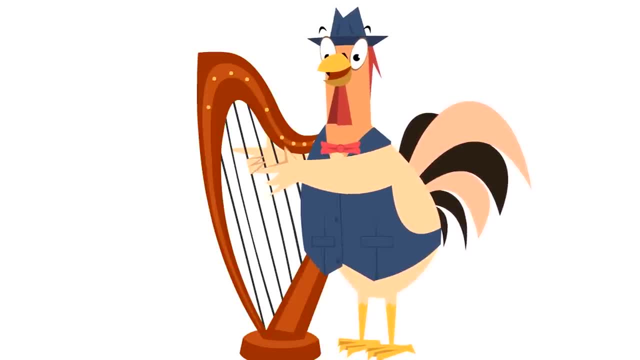 hear it. we're having audio problems with Fred right now. Fred, you look so happy Fred, right now Fred, you look so happy Fred, right now, Fred, you look so happy playing we. we can't hear you, okay, you playing we. we can't hear you. okay, you playing we. we can't hear you. okay, you got it. you gotta wear your mic or 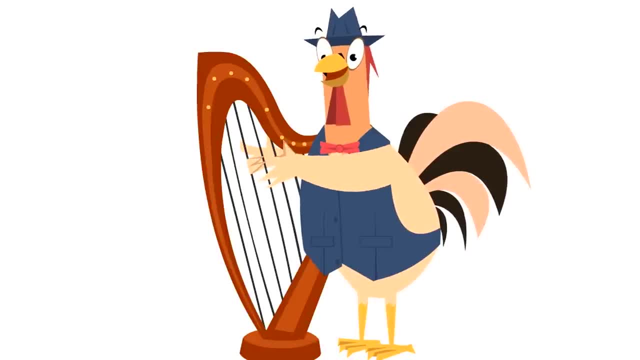 got it. you gotta wear your mic, or got it, you gotta wear your mic, or something. we can't hear the music he something we can't hear. the music he something we can't hear. the music he doesn't even know, doesn't, isn't that? doesn't even know, doesn't, isn't that? 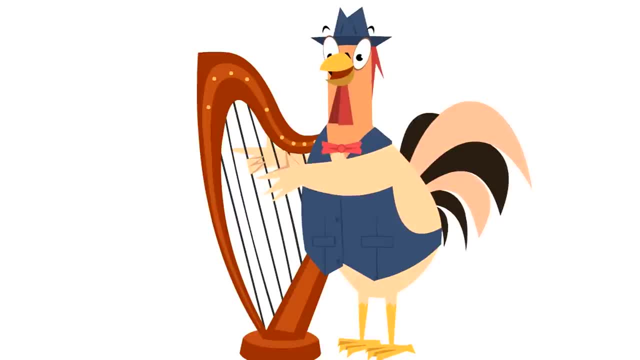 doesn't even know, doesn't? isn't that nice. you know Fred is just plucking away. nice, you know Fred is just plucking away. nice, you know Fred is just plucking away. he's having a good time, you know kind he's having a good time, you know kind. 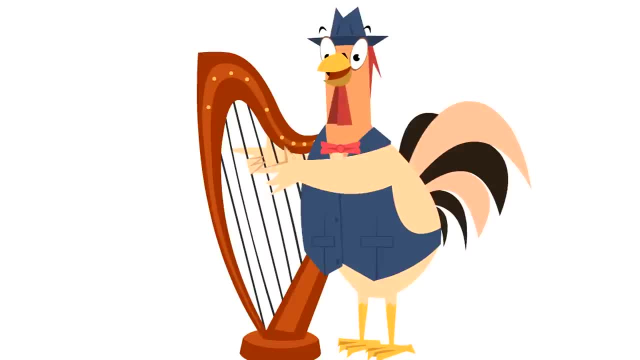 he's having a good time. you know, kind of like we're having a good time, right of like we're having a good time right of like we're having a good time right now with these learning videos, and next now with these learning videos, and next now with these learning videos, and next we are going to learn about urban. 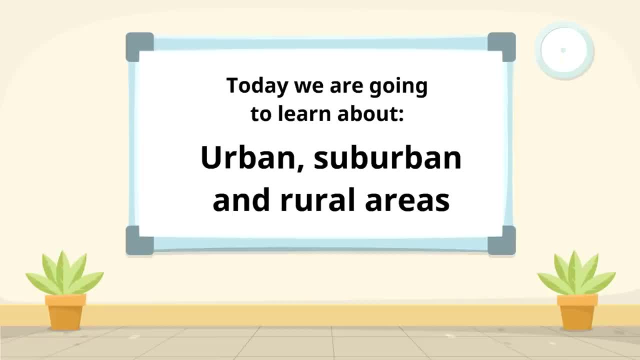 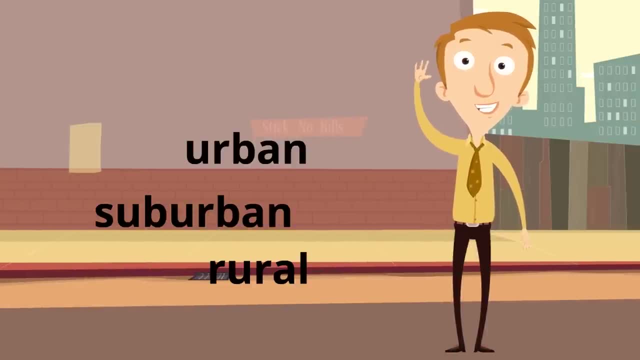 we are going to learn about urban. we are going to learn about urban, suburban and rural areas, these three suburban and rural areas, these three suburban and rural areas, these three words- urban, suburban and rural- describe words. urban, suburban and rural describe words urban, suburban and rural describe where we live. some people live in urban. 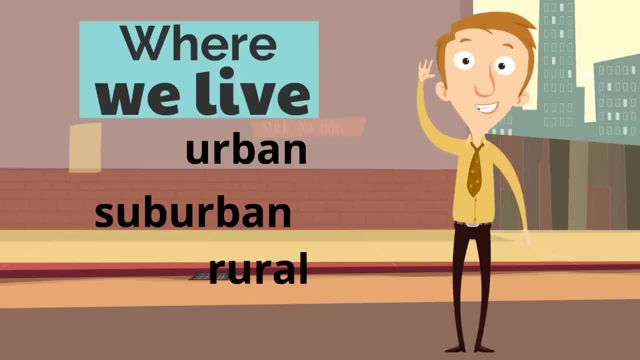 where we live. some people live in urban where we live. some people live in urban areas. some people live in rural areas areas. some people live in rural areas areas. some people live in rural areas and some people live in suburban areas and some people live in suburban areas. 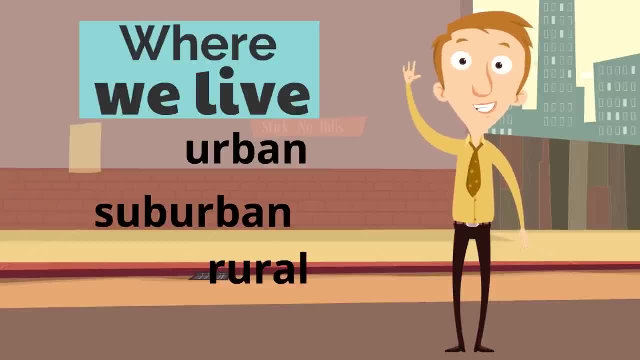 and some people live in suburban areas. we're gonna learn all three of these. we're gonna learn all three of these. we're gonna learn all three of these different types of areas, so you can different types of areas. so you can different types of areas, so you can describe where you live. the first type: 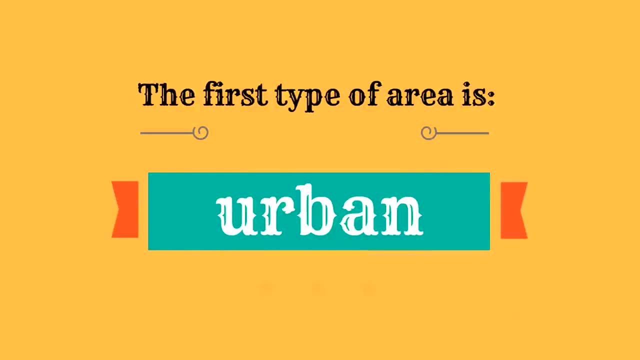 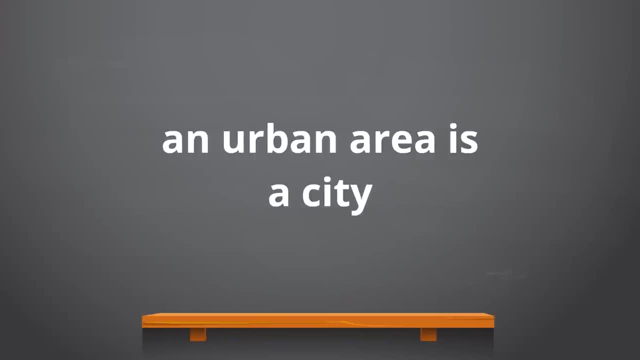 describe where you live. the first type: describe where you live. the first type of area that we're gonna learn is urban of area. that we're gonna learn is urban of area. that we're gonna learn is urban urban areas. an urban area is a city it urban areas. an urban area is a city it. 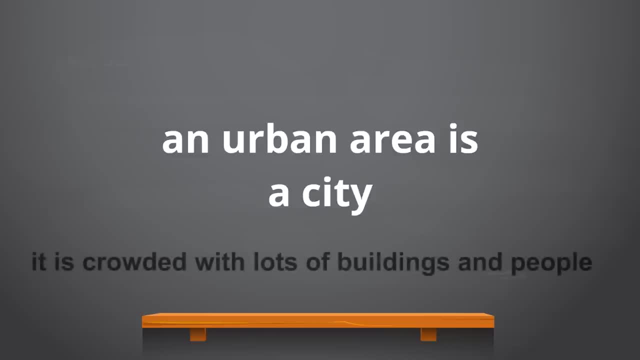 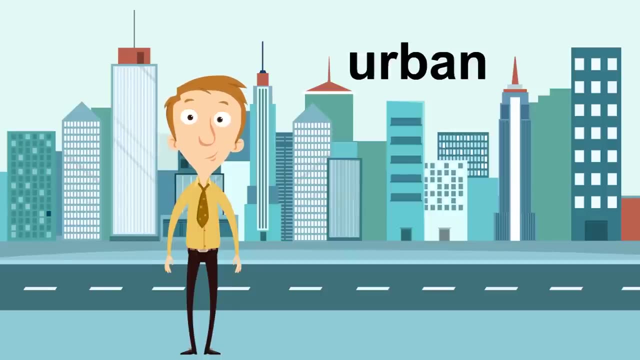 urban areas. an urban area is a city. it is crowded with lots of buildings and is crowded with lots of buildings and is crowded with lots of buildings and people. here we have a great example of an urban. here we have a great example of an urban. here we have a great example of an urban area. the buildings are close together. 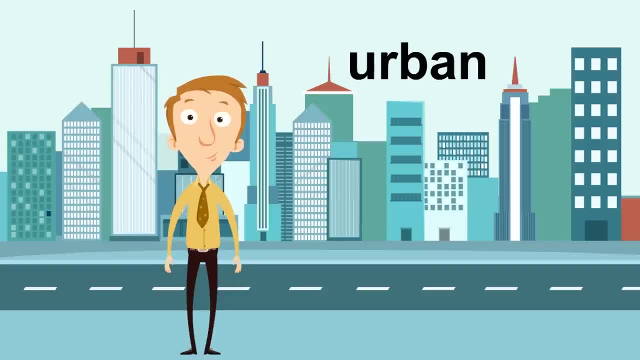 area the buildings are close together. area. the buildings are close together. they're very tall, lots of people, they're very tall, lots of people, they're very tall, lots of people, and traffic would come through here might, and traffic would come through here might, and traffic would come through here might be very loud. this is an urban area. 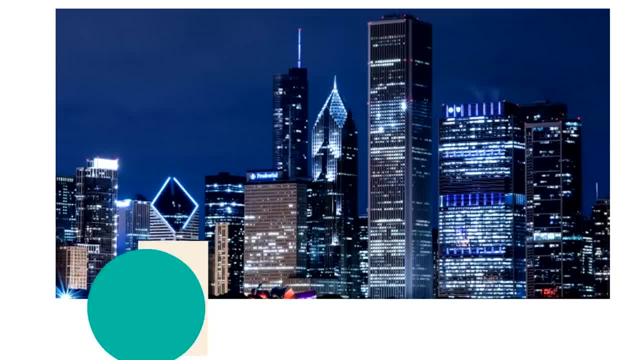 be very loud. this is an urban area. be very loud. this is an urban area, city environment. here's another great city environment. here's another great city environment. here's another great example of an urban environment. look at example of an urban environment. look at example of an urban environment. look at these tall buildings of lights. this is a. 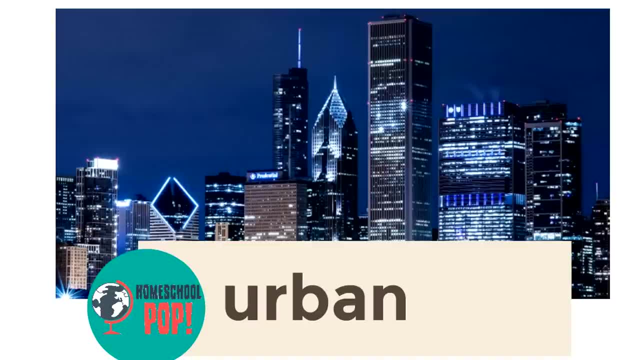 these tall buildings of lights. this is a. these tall buildings of lights. this is a city. if it's a city, that means it's an city. if it's a city, that means it's an city. if it's a city, that means it's an urban area. this is an urban area. 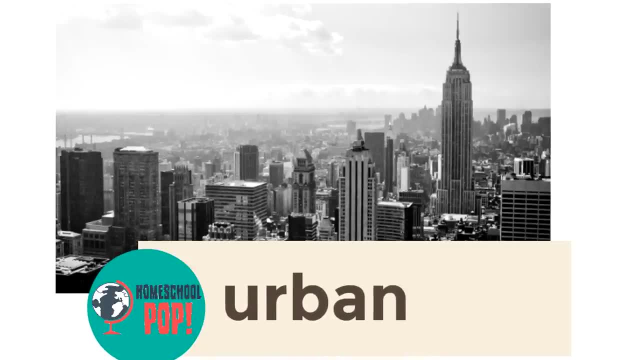 here's another urban area. lots of here's another urban area, lots of here's another urban area. lots of buildings, lots of buildings. they're all buildings, lots of buildings, they're all buildings, lots of buildings. they're all close together. some of them are very close together, some of them are very. 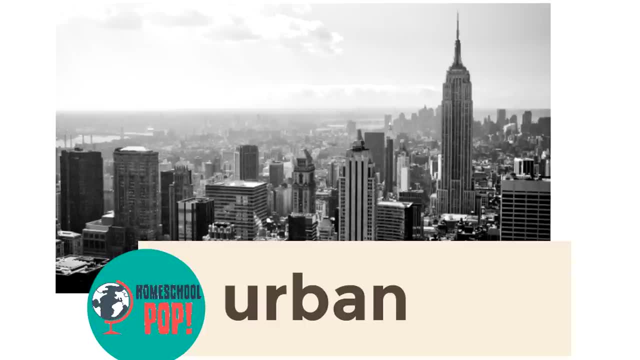 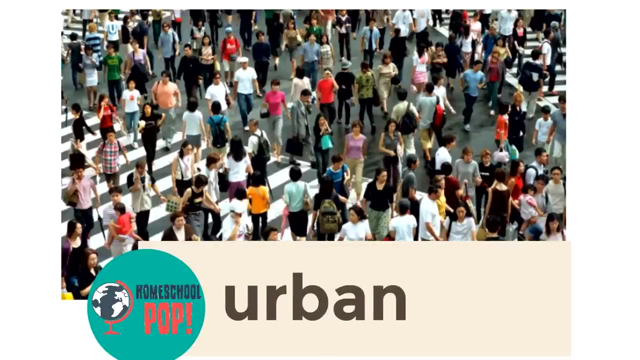 close together. some of them are very tall. you can imagine all the traffic all tall. you can imagine all the traffic all tall. you can imagine all the traffic, all the people there. this is an urban area. here's another example of an urban area. here's another example of an urban area. 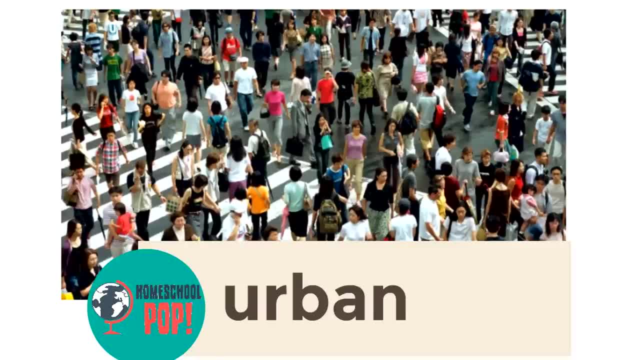 here's another example of an urban area and you see all the people crowds of and you see all the people crowds of and you see all the people crowds of people. urban areas are very crowded, lots people. urban areas are very crowded, lots people. urban areas are very crowded. lots of people, lots of traffic, not just in. 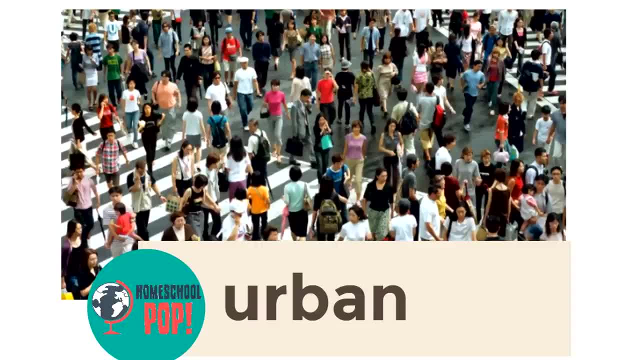 of people. lots of traffic, not just in of people. lots of traffic not just in cars but foot traffic. lots of people, cars but foot traffic. lots of people, cars but foot traffic. lots of people walking in urban area, walking in urban area, walking in urban area. here's another example of an urban area. 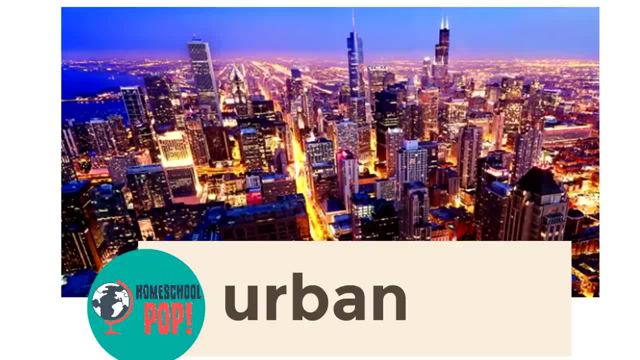 here's another example of an urban area. here's another example of an urban area, and we know it's an urban area because and we know it's an urban area because, and we know it's an urban area because it's a picture of a city. all cities are. 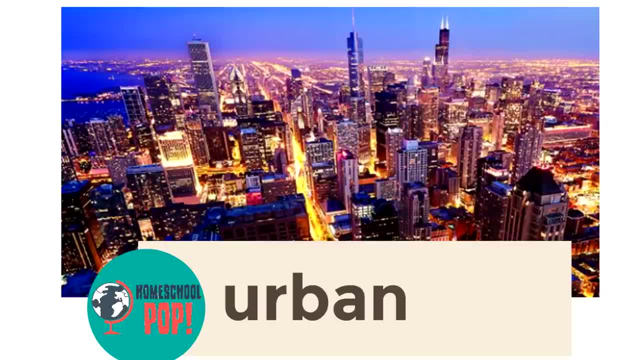 it's a picture of a city. all cities are. it's a picture of a city: all cities are urban areas. this is an urban area: tons urban areas. this is an urban area, tons urban areas. this is an urban area: tons of buildings, many of them tall, lots of. 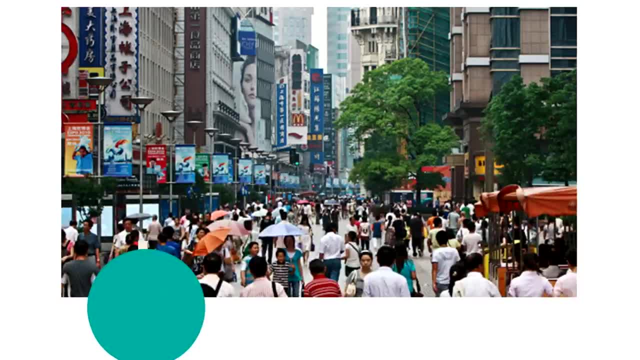 of buildings, many of them tall. lots of of buildings, many of them tall. lots of people, lots of traffic. here's another people, lots of traffic. here's another people, lots of traffic. here's another great picture of an urban area, all the great picture of an urban area, all the 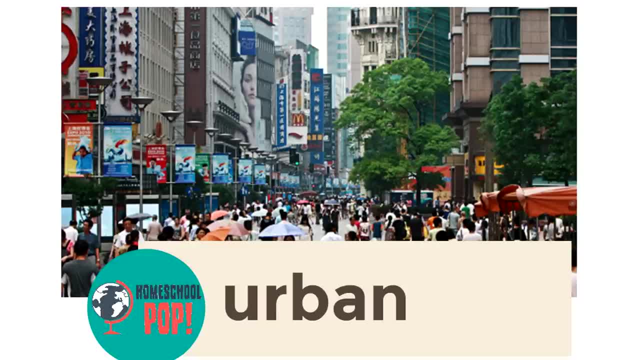 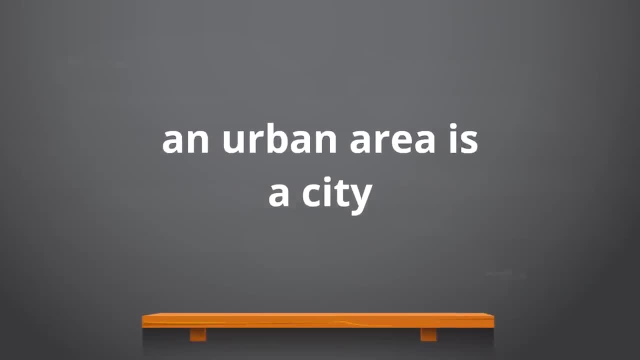 great picture of an urban area: all the people, all the buildings, everything's people, all the buildings, everything's people, all the buildings, everything's close together, everything's crowded. this close together, everything's crowded, this close together, everything's crowded. this is an urban area to review. an urban area is a city. it is. 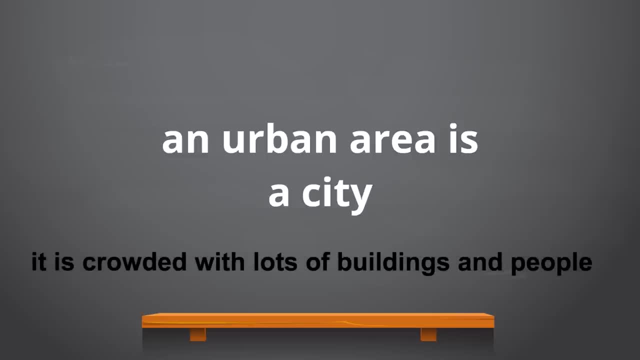 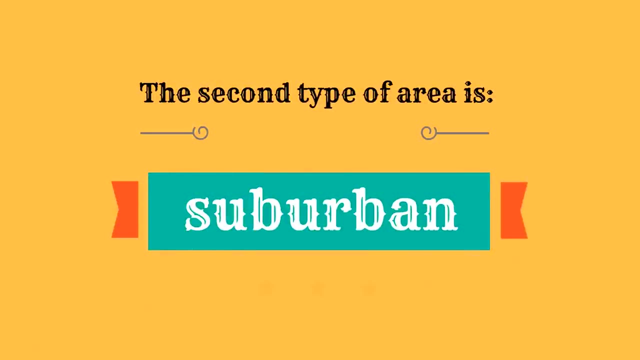 to review an urban area is a city. it is to review an urban area is a city. it is crowded with lots of buildings and crowded with lots of buildings and crowded with lots of buildings and people. the second type of area is suburban. the second type of area is suburban. 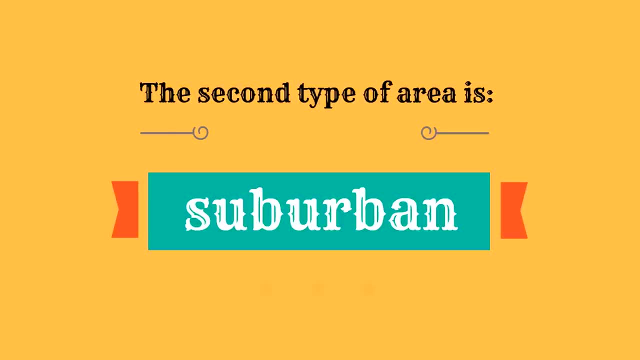 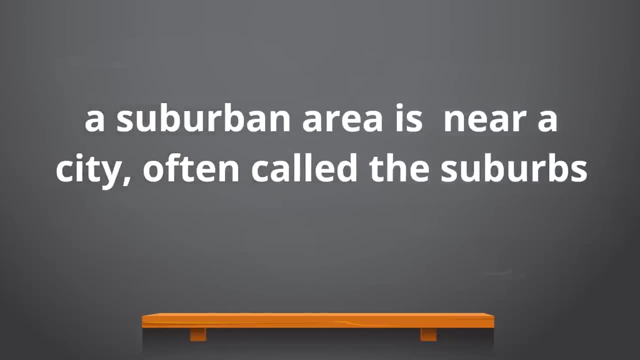 the second type of area is suburban suburban areas. a suburban area is suburban areas. a suburban area is suburban areas. a suburban area is near a city, and it's often called the near a city. and it's often called the near a city and it's often called the suburbs. it's less crowded than the city. 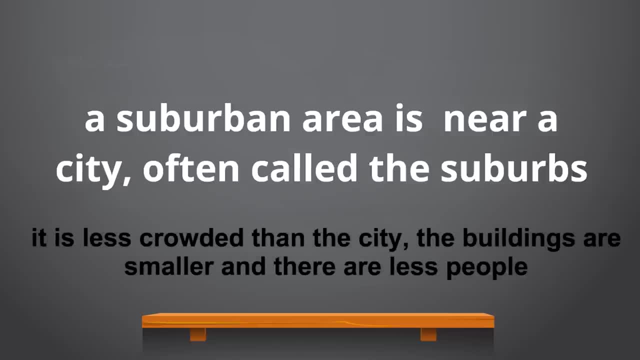 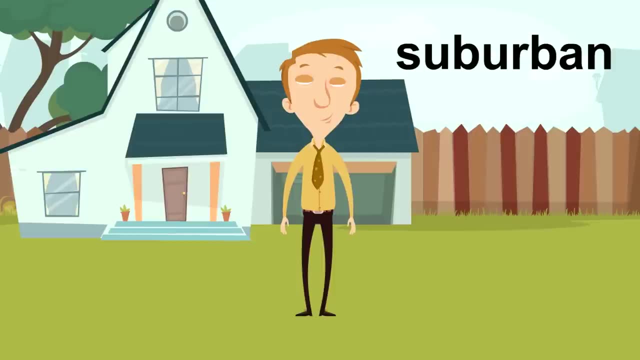 suburbs: it's less crowded than the city. suburbs: it's less crowded than the city. the buildings are smaller. there are less. the buildings are smaller. there are less the buildings are smaller. there are less people than are in the urban areas. here is an example of a suburban. 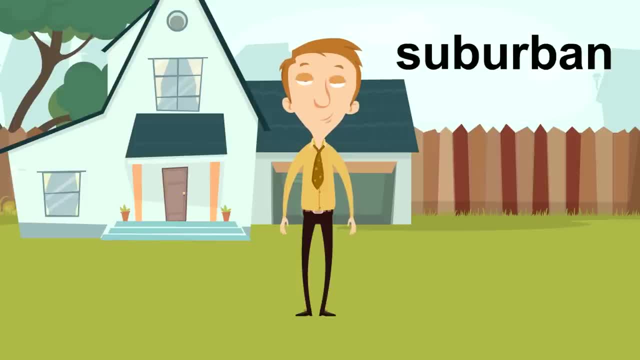 here is an example of a suburban. here is an example of a suburban. environments less crowded. it's quieter environments less crowded. it's quieter environments, less crowded. it's quieter than the urban areas people live in, than the urban areas people live in. than the urban areas people live in houses with yards. they usually drive. 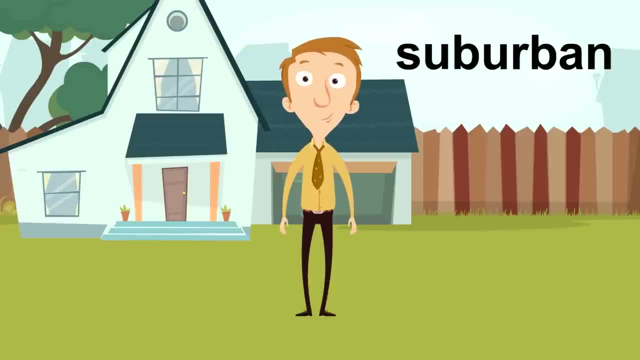 houses with yards. they usually drive houses with yards. they usually drive because they aren't able to walk, because they aren't able to walk, because they aren't able to walk everywhere on foot. here is another everywhere on foot. here is another everywhere on foot. here is another suburban area. as you can see, it's less. 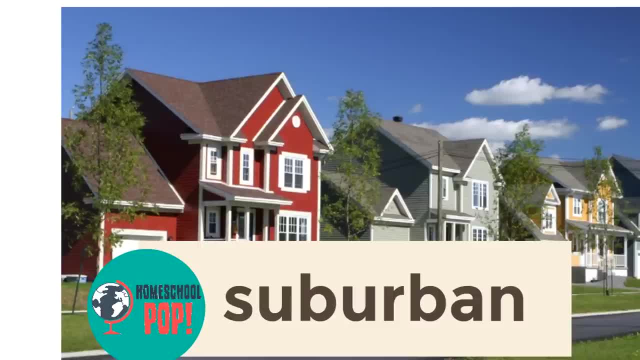 suburban area. as you can see, it's less suburban area. as you can see, it's less crowded than the city. the houses have crowded than the city. the houses have crowded than the city. the houses have yards. there's more space. it's a little yards. there's more space, it's a little. 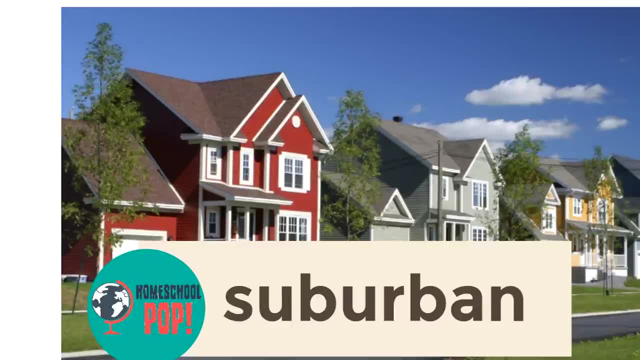 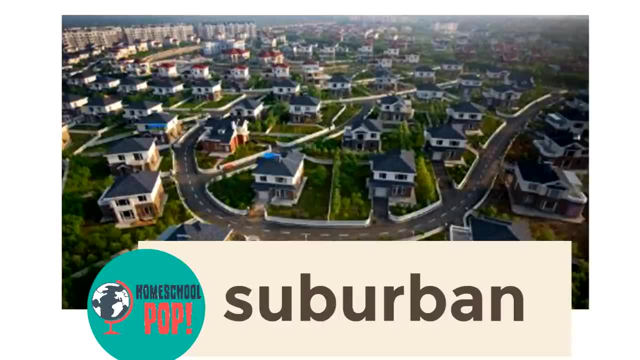 yards. there's more space. it's a little bit more quiet. it's a suburban area, bit more quiet. it's a suburban area, bit more quiet. it's a suburban area. here's another suburban area, and this is here's another suburban area, and this is here's another suburban area. and this is looking up from the sky and you can see. 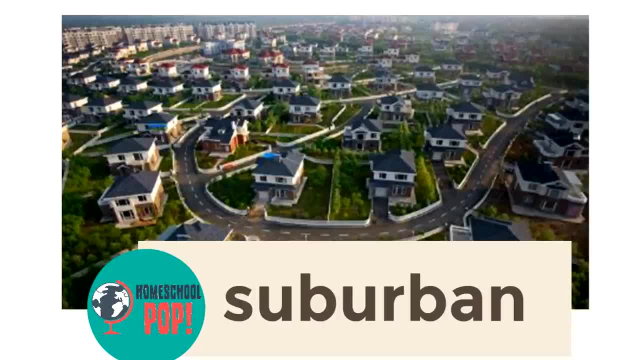 looking up from the sky and you can see. looking up from the sky and you can see all the homes, all the homes have yards. all the homes, all the homes have yards. all the homes, all the homes have yards. there's a little bit more space, it's not. 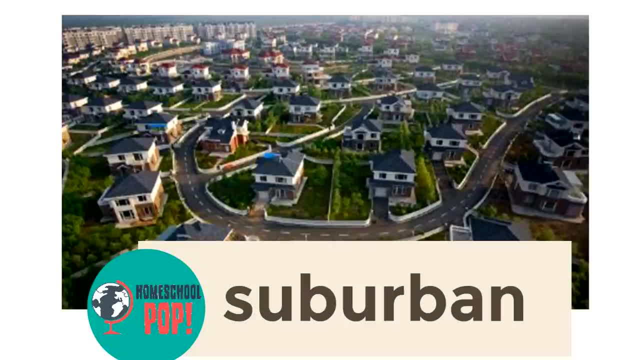 there's a little bit more space. it's not. there's a little bit more space. it's not as crowded. it's not as busy as the as crowded. it's not as busy as the as crowded. it's not as busy as the urban areas. here's a picture of a. 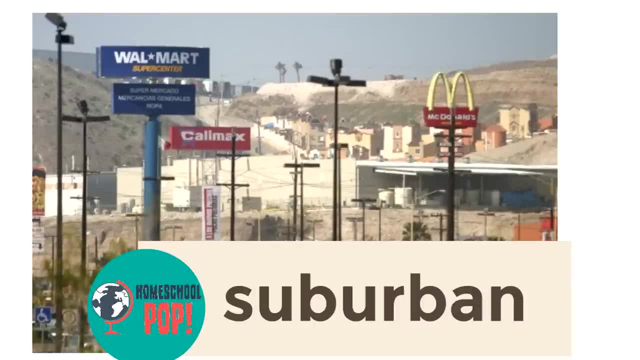 urban areas. here's a picture of a urban areas. here's a picture of a suburban area and you can see different suburban area and you can see different suburban area and you can see different stores. there's a little bit more space. stores: there's a little bit more space. 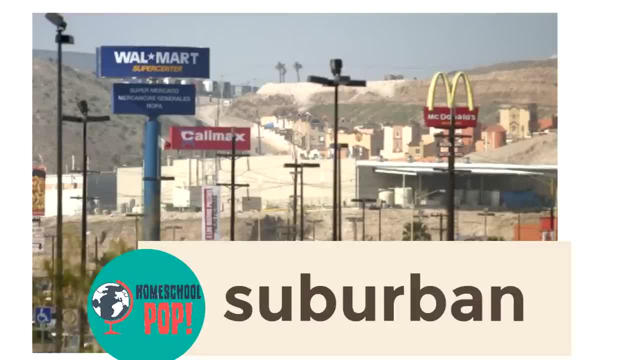 stores there's a little bit more space in between them in an urban area, in between them in an urban area, in between them. in an urban area, everything is totally crowded. but in a, everything is totally crowded. but in a, everything is totally crowded. but in a suburban area there's a little bit more. 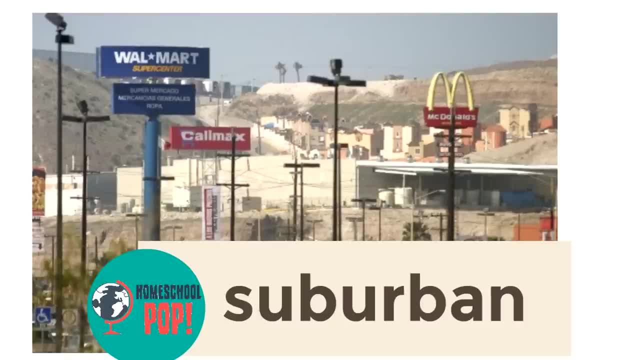 suburban area. there's a little bit more suburban area. there's a little bit more space. here's our final picture of suburban. here's our final picture of suburban. here's our final picture of suburban area. you can look and see it's not as area. you can look and see it's not as. 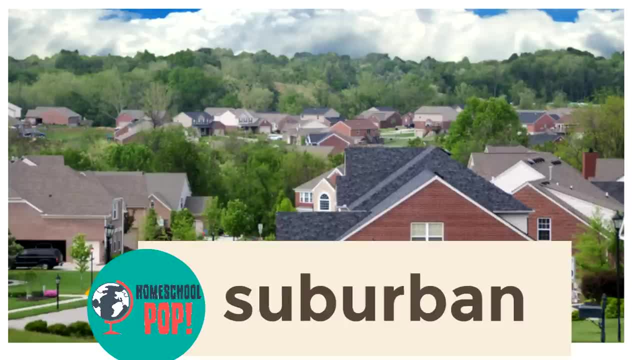 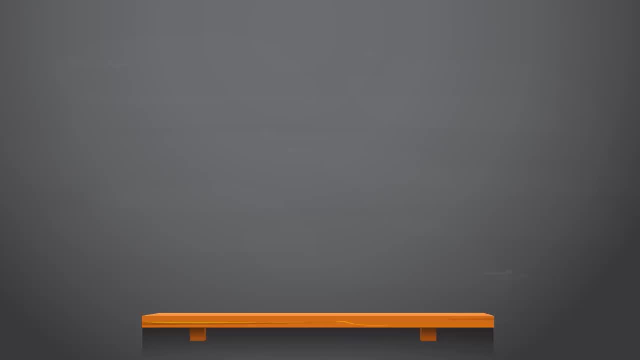 area. you can look and see it's not as crowded as the urban areas. this is a crowded as the urban areas. this is a crowded as the urban areas. this is a suburban area, just a little more space. a suburban area, just a little more space. a suburban area, just a little more space, a little more quiet. to summarize, a. 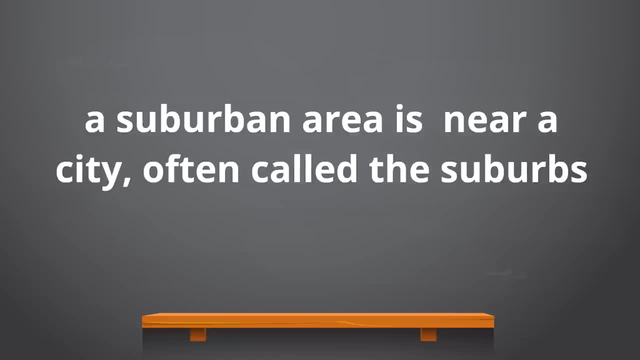 little more quiet. to summarize: a little more quiet. to summarize: a suburban area is near a city and it's suburban area is near a city and it's suburban area is near a city and it's often called the suburbs. it is less often called the suburbs, it is less. 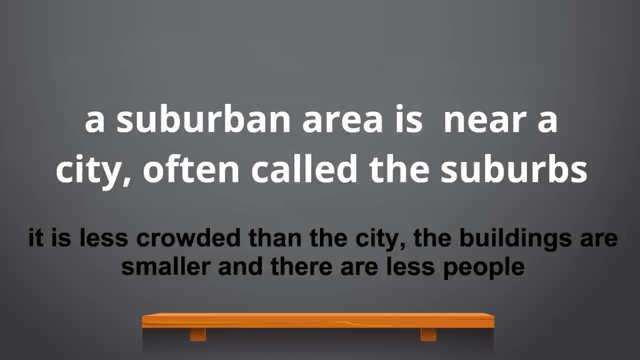 often called the suburbs. it is less crowded than the city. the buildings are crowded than the city. the buildings are crowded than the city. the buildings are smaller and there are less people than smaller and there are less people than smaller and there are less people than are in the urban areas. the third and 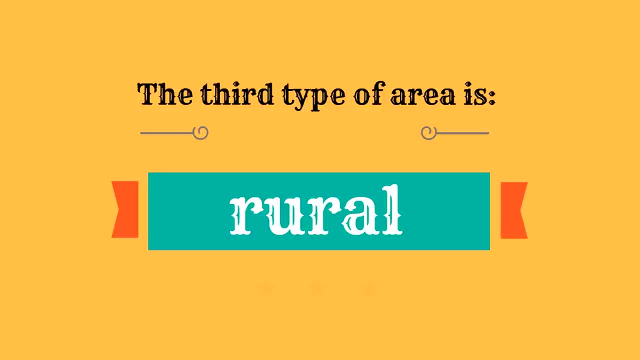 are in the urban areas. the third and are in the urban areas. the third and final type of area is rural. a rural final type of area is rural. a rural final type of area is rural. a rural area is away from the cities and suburbs area is away from the cities and suburbs. 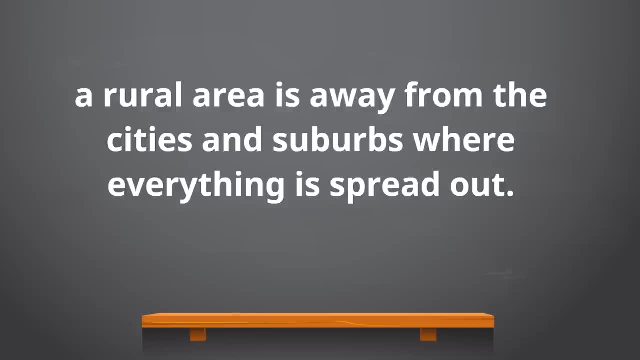 area is away from the cities and suburbs, where everything is spread out. it, where everything is spread out. it where everything is spread out, it is not crowded. there are not many people is not crowded. there are not many people is not crowded. there are not many people or buildings. here's a. 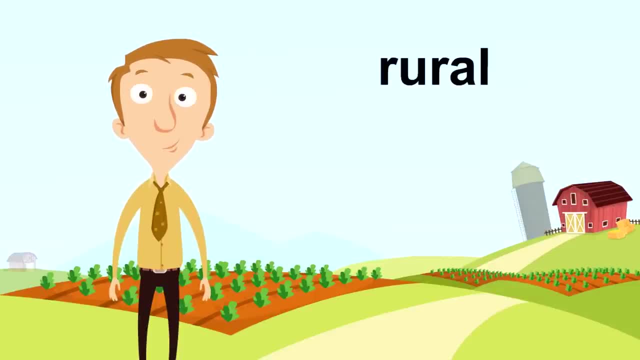 or buildings- here's a. or buildings- here's a. here's an example of a rural area. it's a rural example of a rural area. it's a rural example of a rural area. it's a rural area because it's not in the city or the area, because it's not in the city or the. 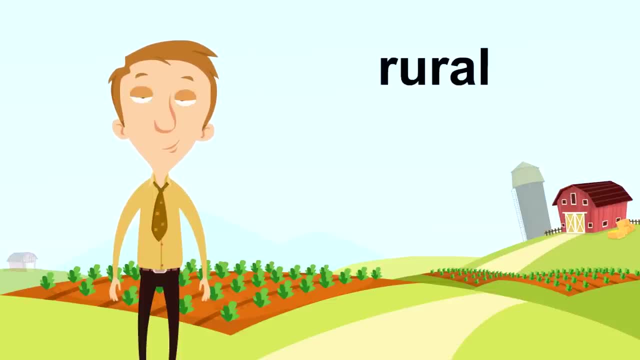 area, because it's not in the city or the suburbs. everything is very spread out. suburbs, everything is very spread out. suburbs, everything is very spread out. there are not a lot of people and not a. there are not a lot of people and not a. there are not a lot of people and not a lot of buildings. here's another example. 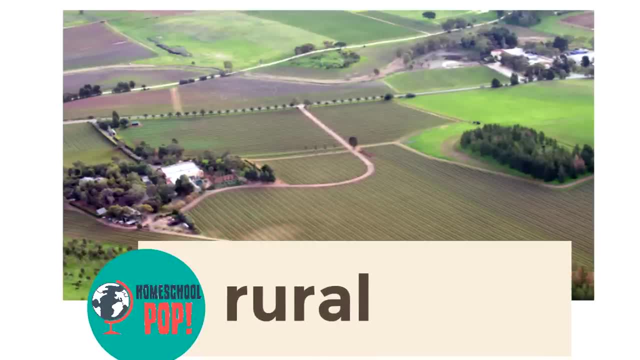 lot of buildings. here's another example: lot of buildings. here's another example of a rural area. look, there aren't that of a rural area. look, there aren't that of a rural area. look, there aren't that. many buildings, that many people. many buildings, that many people. 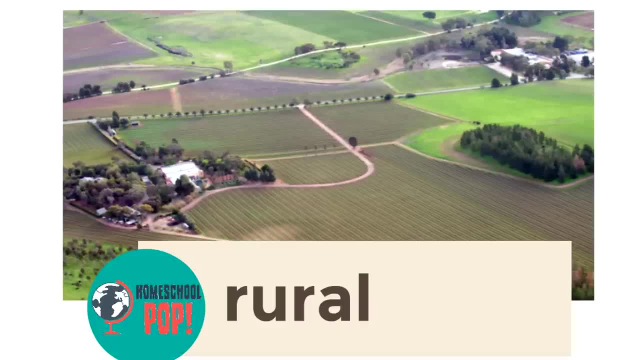 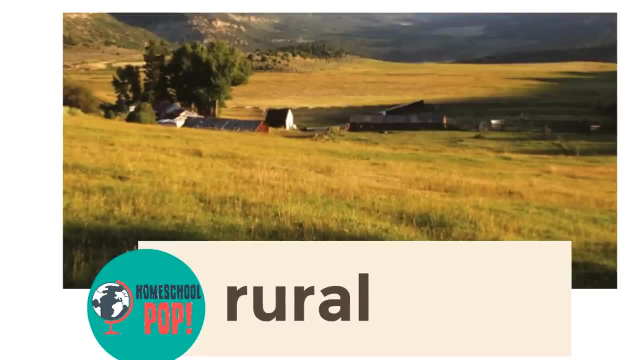 many buildings, that many people. everything is very spread out. it's rural. everything is very spread out. it's rural. everything is very spread out. it's rural. here's another picture of a rural area. here's another picture of a rural area. here's another picture of a rural area. look how spread out everything is you. 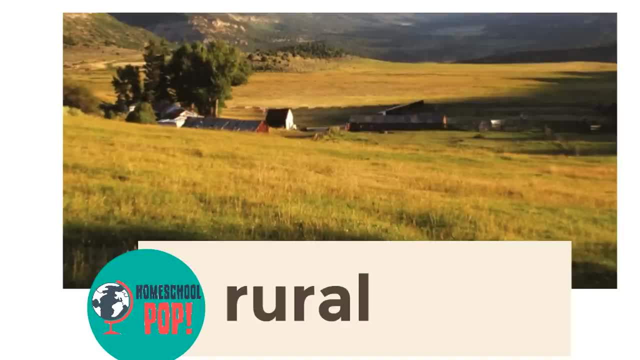 look how spread out everything is. you look how spread out everything is. you don't see the crowds. you don't see all. don't see the crowds. you don't see all. don't see the crowds. you don't see all the people. you don't see any big. 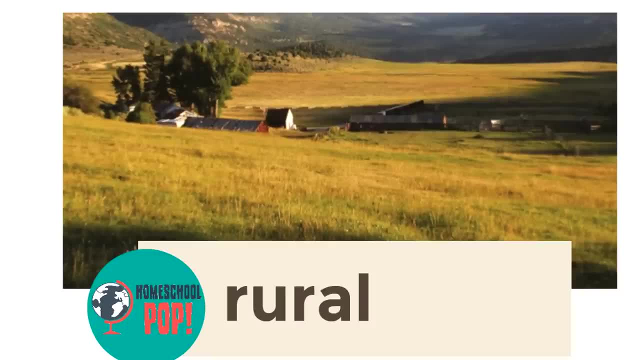 the people. you don't see any big the people. you don't see any big buildings. it's a rural area. look at this buildings: it's a rural area. look at this buildings. it's a rural area. look at this picture of a rural area. it's close up to. 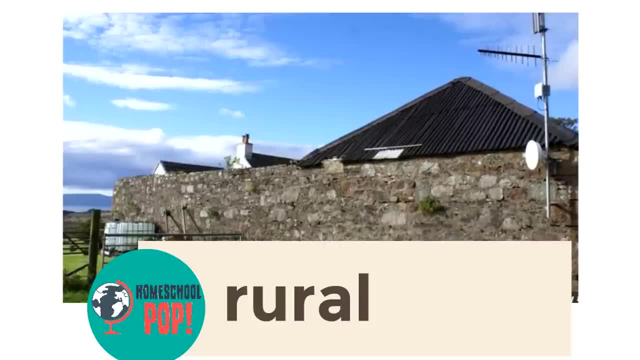 picture of a rural area. it's close up to picture of a rural area. it's close up to a house, but if you can look in the a house, but if you can look in the a house, but if you can look in the background, there isn't much of anything. 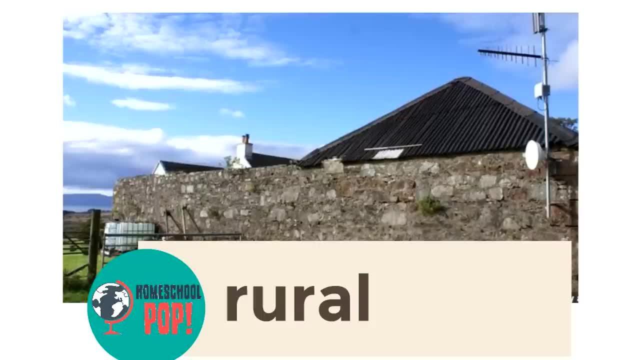 background, there isn't much of anything. background, there isn't much of anything else. around everything is spread out else. around everything is spread out else, around everything is spread out. there aren't that many buildings. it's there aren't that many buildings. it's. there aren't that many buildings. it's not in a neighborhood, it's rural here's. 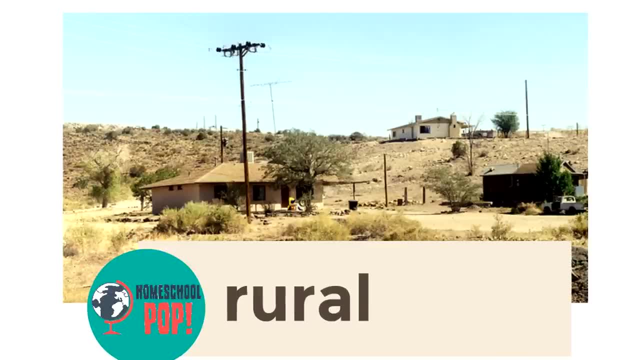 not in a neighborhood, it's rural here's not in a neighborhood, it's rural. here's our final picture of a rural area. look our final picture of a rural area. look our final picture of a rural area. look, it's not in the neighborhood, it's not in. 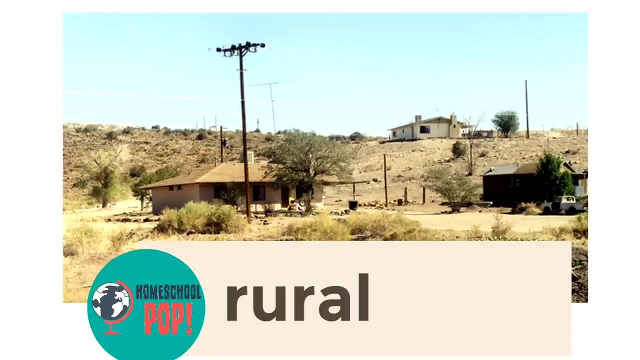 it's not in the neighborhood. it's not in. it's not in the neighborhood. it's not in the city. it's not the suburbs, it's a the city. it's not the suburbs, it's a the city. it's not the suburbs, it's a rural area where everything is spread. 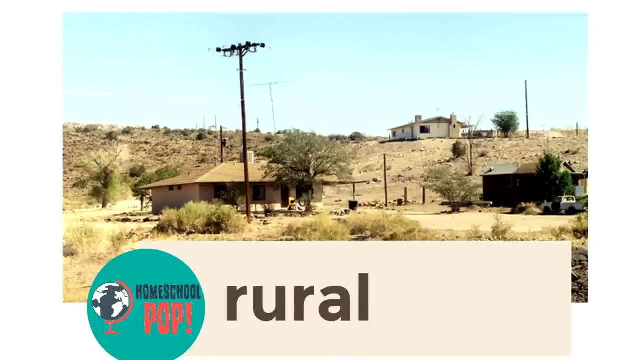 rural area where everything is spread out. there aren't a lot of people and out there aren't a lot of people and out there aren't a lot of people and there aren't a lot of buildings to there aren't a lot of buildings to there aren't a lot of buildings. to summarize, a rural area is away from the 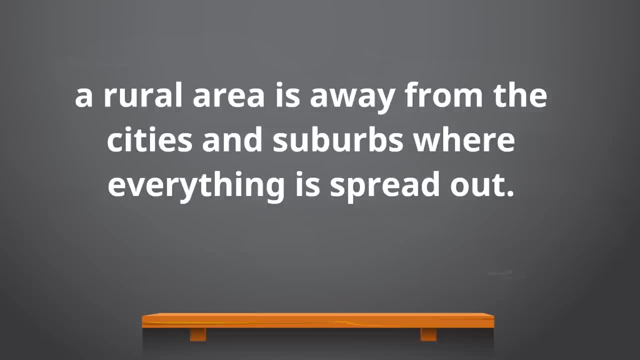 summarize: a rural area is away from the summarize. a rural area is away from the cities and suburbs where everything is cities and suburbs, where everything is cities and suburbs, where everything is spread out. it is not crowded. there are spread out, it is not crowded. there are spread out, it is not crowded. there are not many people or buildings. so where do 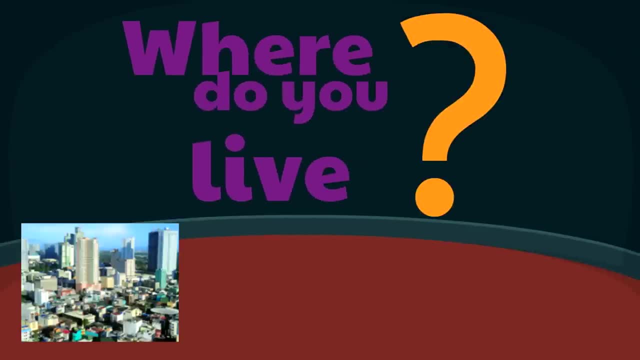 not many people or buildings. so where do not many people or buildings? so where do you live? do you live in an urban- you live. do you live in an urban- you live. do you live in an urban environment- the city- or do you live in environment- the city or do you live in? 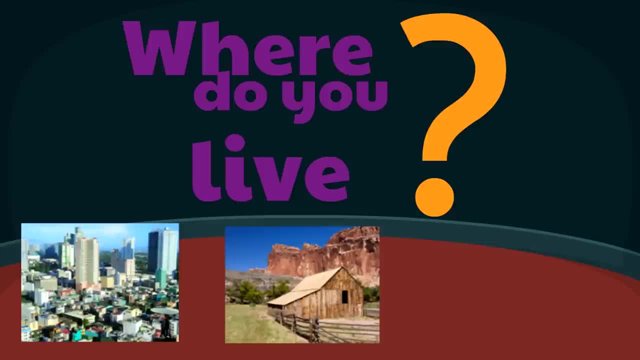 environment, the city, or do you live in the rural environment, where everything's the rural environment, where everything's the rural environment, where everything's spread out? or do you live in a suburban spread out? or do you live in a suburban spread out, or do you live in a suburban area or the suburbs that's near a city? 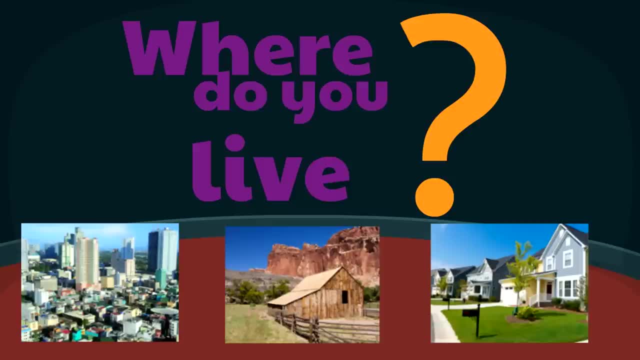 area or the suburbs that's near a city area, or the suburbs that's near a city, but it's not as crowded. it's not as loud, but it's not as crowded. it's not as loud but it's not as crowded. it's not as loud as the city. where do you live? cool? 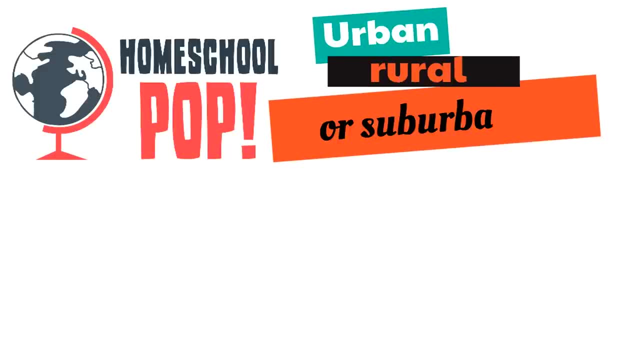 as the city. where do you live cool as the city? where do you live cool? we're gonna find out how much you learn. we're gonna find out how much you learn. we're gonna find out how much you learn. we're gonna play a game that we're 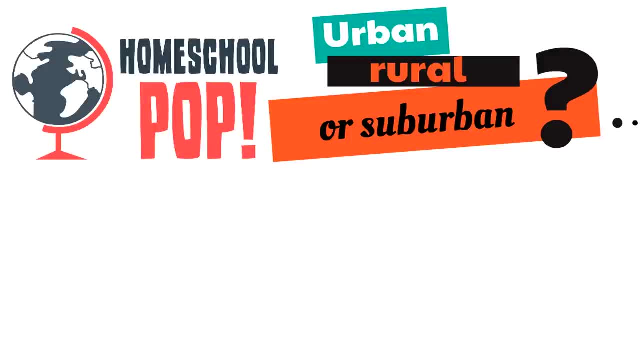 we're gonna play a game that we're. we're gonna play a game that we're calling urban, rural or suburban, and we're calling urban, rural or suburban, and we're calling urban, rural or suburban, and we're gonna show you some areas and you tell: gonna show you some areas and you tell: 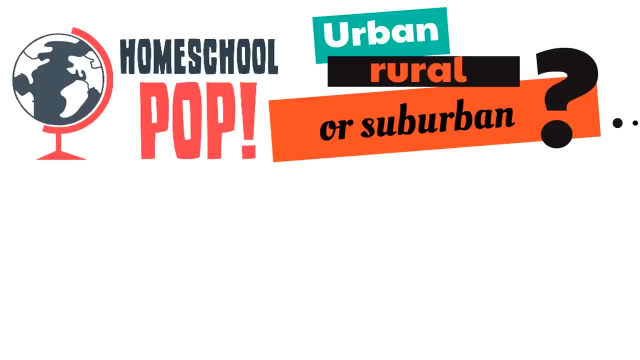 gonna show you some areas and you tell us which one it is. here's our first one. is this a picture? here's our first one. is this a picture? here's our first one. is this a picture of an urban area, a rural area or a of an urban area, a rural area or a? 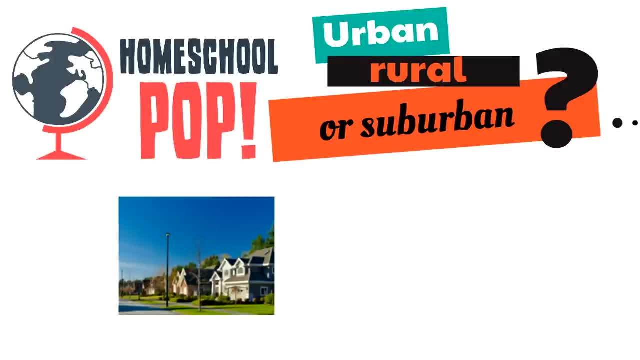 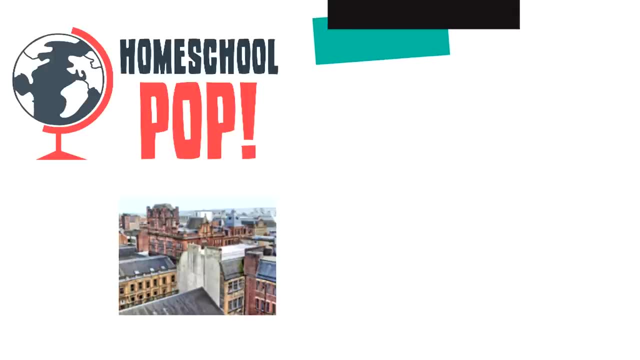 of an urban area, a rural area or a suburban area- suburban- great job, let's try suburban area- suburban- great job, let's try suburban area- suburban- great job, let's try this one, this one, this one. is this urban, rural or suburban? is this urban, rural or suburban? 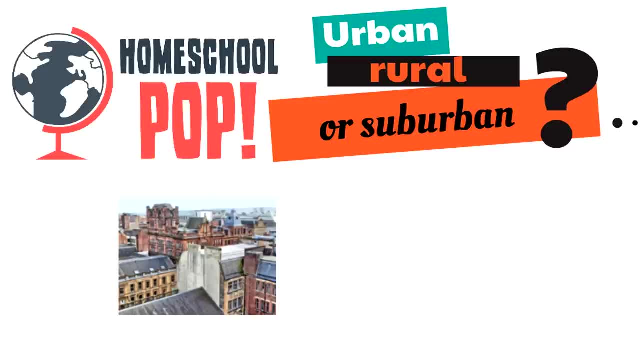 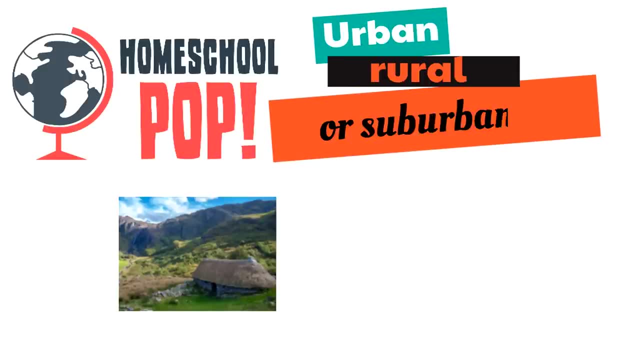 is this urban, rural or suburban? great job, it's an urban area, let's try. great job, it's an urban area, let's try. great job, it's an urban area. let's try this one. is it urban, rural or suburban? this one: is it urban, rural or suburban? 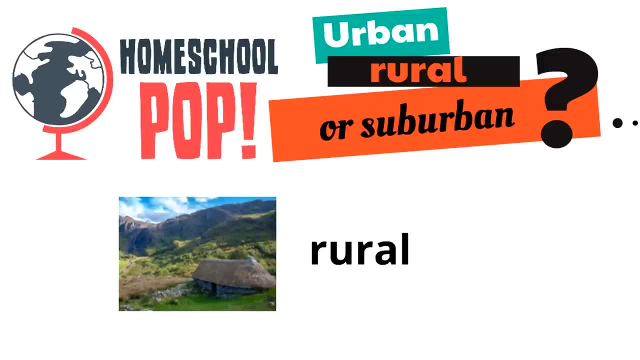 this one. is it urban, rural or suburban? it's rural, great job. this one looks like it's rural, great job. this one looks like it's rural, great job. this one looks like fun. is it fun? is it fun? is it urban, rural or suburban? urban, rural or suburban? 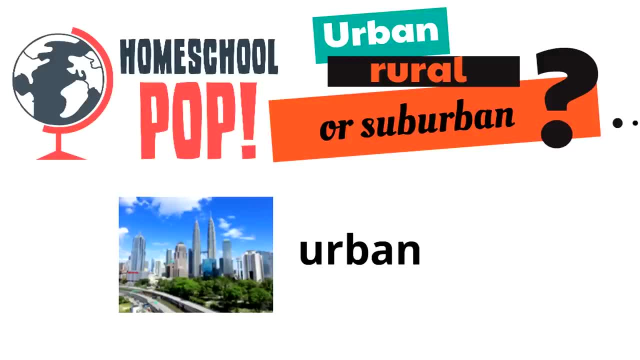 urban, rural or suburban? yeah, it's urban. yeah, it's urban. yeah, it's urban. here's another one. is it urban, rural? here's another one. is it urban, rural? here's another one. is it urban, rural or suburban? or suburban or suburban? yeah, it's suburban. yeah, it's suburban.